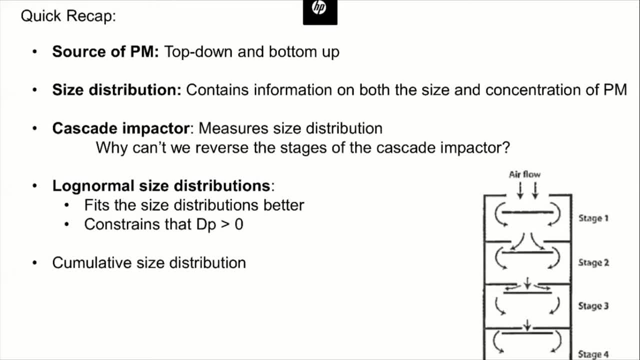 So last class we talked about the sources of PM. We mentioned that there are mainly two methods to form these PM. right, We can use the top-down method, which is breaking things apart. right, That happens when we do construction. And we also have the bottom-up approach. So this happens when we combust something, right? 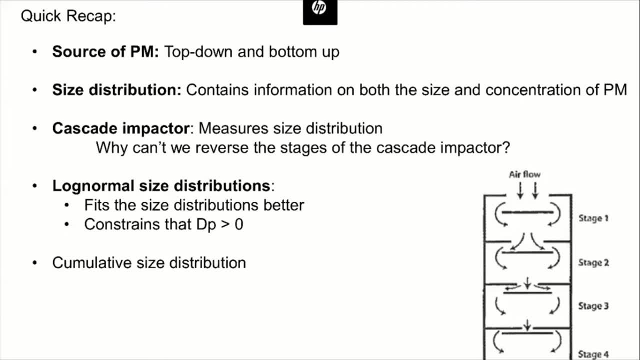 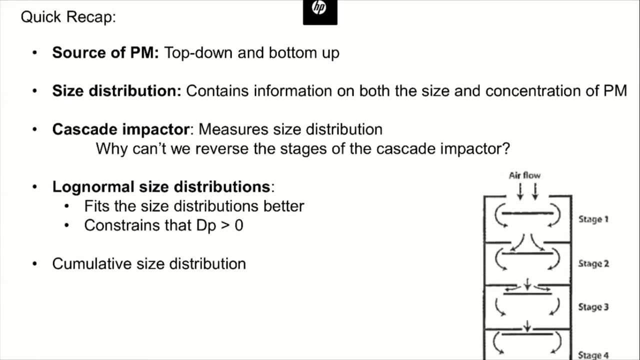 Or like the Smoky Mountain right. So we have molecules getting together with each other and form these stable clusters. So we also mentioned the size distribution. So basically people are maybe interested in a series of properties of particles. So last class we just mentioned about people are interested in the size, interested in concentration. 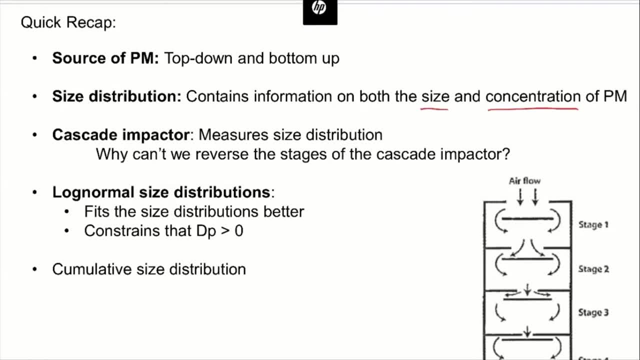 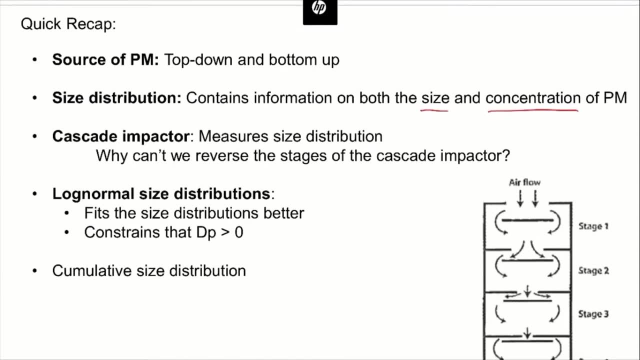 but actually people are also interested in the chemical composition, toxicity, so on, mass, so on and so forth. right, But the quite important one is called the size distribution, which basically contains both the size distribution and the concentration of the particles. 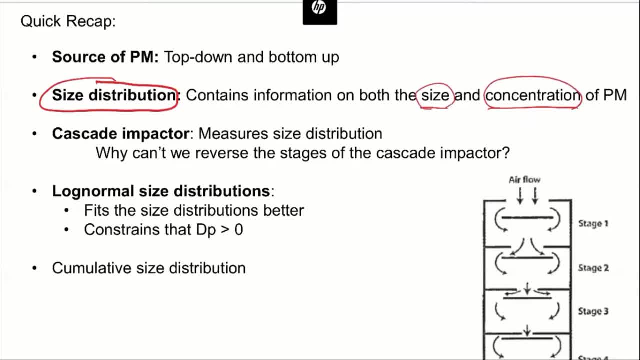 So remember, when we make the plot of the log, normal size distribution right. So this contains both the size of the particle and also the mass concentration of the particle. That's why a size distribution is a quite important item that we have to go through this class again. 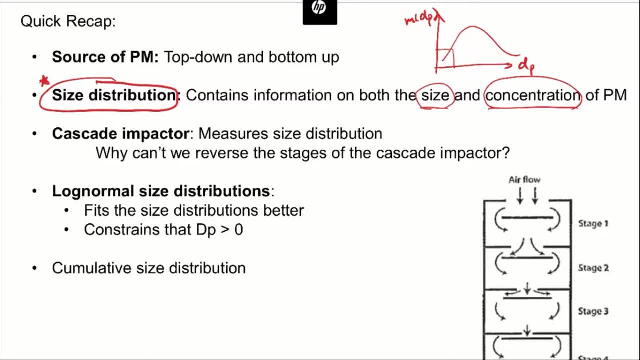 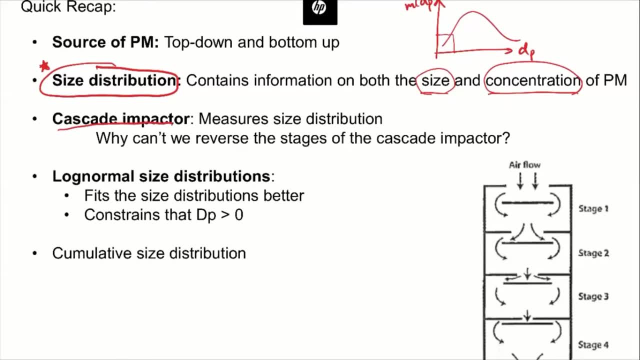 So, regarding the measurement of the size distribution, we mentioned that we can use the concentrationited distribution, right. Yeah, yeah, We're there. can use a cascade impactor. So a cascade impactor is just a multi-stage impactor, right. 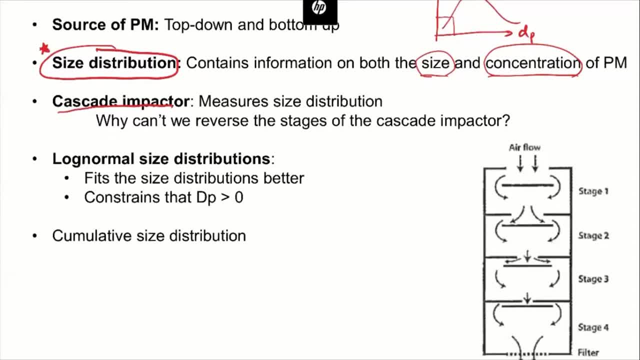 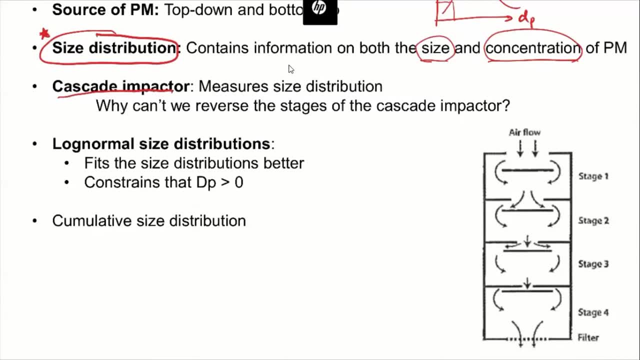 So each stage of the impactor will collect particles of specific size. So, for example, for this one, so particles of larger sizes will get collected by the stage one. Remember the potatoes will get collected on the first stage, Ping-pong ball will get collected. 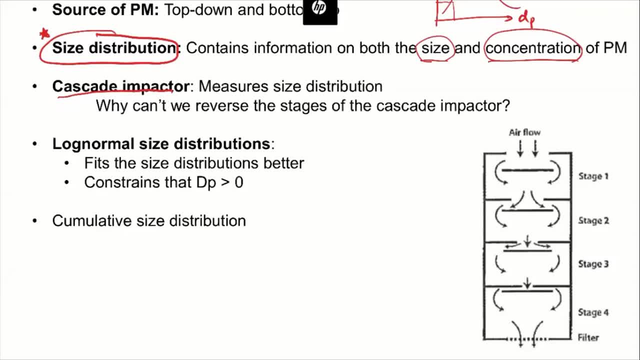 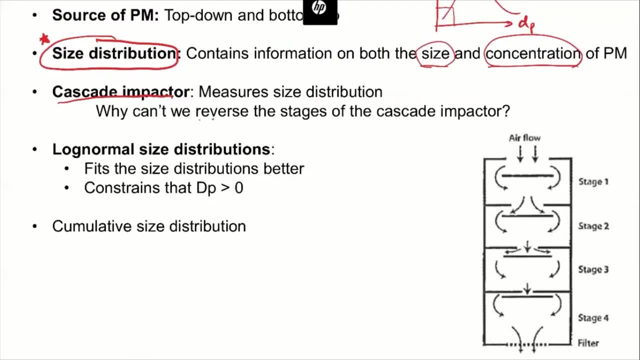 in the second stage, third stage, maybe the grain of sand right The first stage. it can be something else. So then we have a question: So why can't we reverse the stages of the cascade impactor? Let's say we put the stage four at the top stage three, two 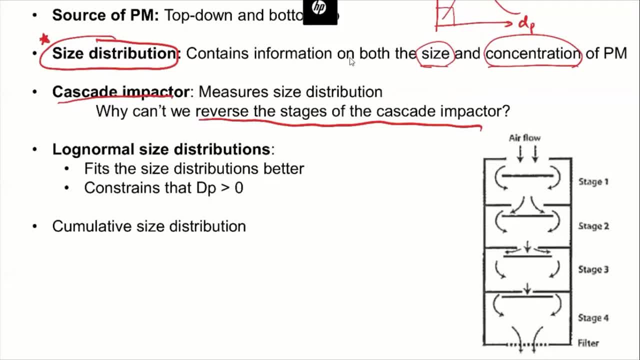 and one. So let's do a quick pool to see why can't we do that. Saddle it Five more seconds. Okay, stop here. All right, so most of you guys are correct, right? So it is quite obvious Basically: if we switch the fourth stage to the top, then we're gonna. 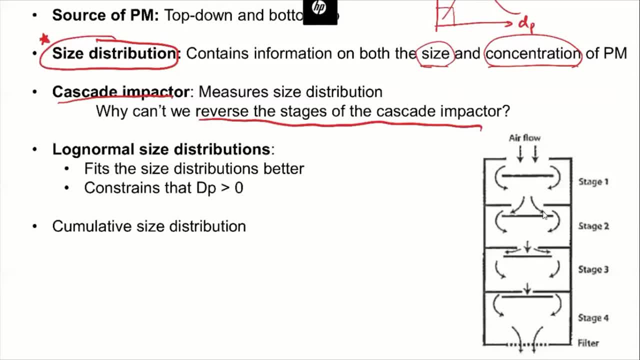 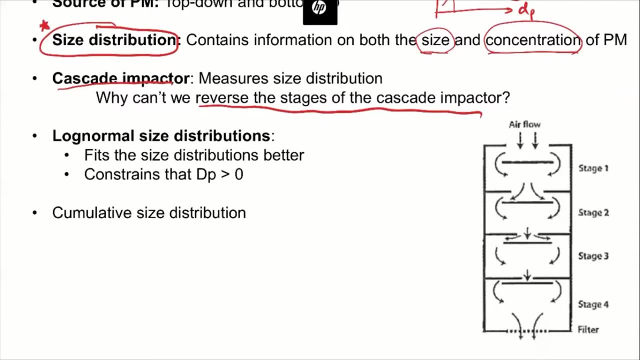 collect everything on the fourth stage, right. There's no way we can collect particles further below, and that's why we would not be able to differentiate particle sizes, So everything would just collect down here, right. That's why the stage sequence matters a lot. So, actually, when you use a 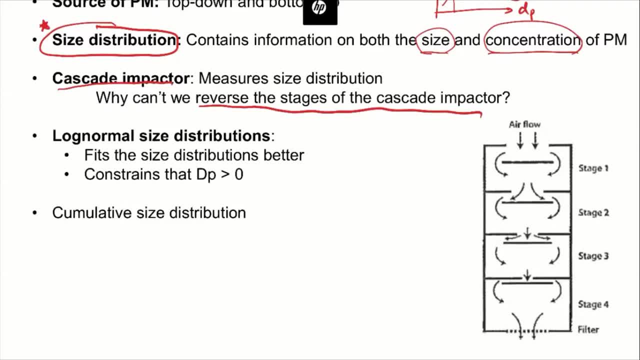 Cascadian vector. actually, I have some demonstrations of the Cascadian vector in my lab. They will specifically label the stage number one, two, three, four, five or ABCDEFG, right? So you have to arrange those stages in order, otherwise you 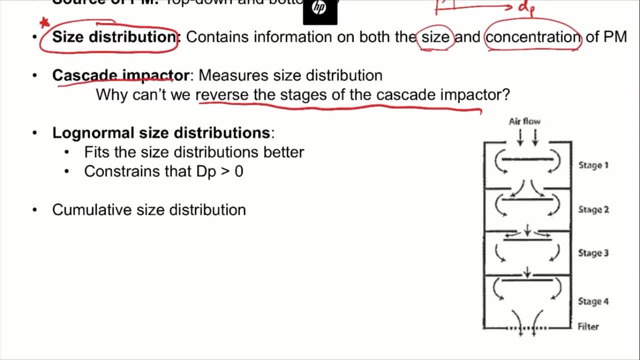 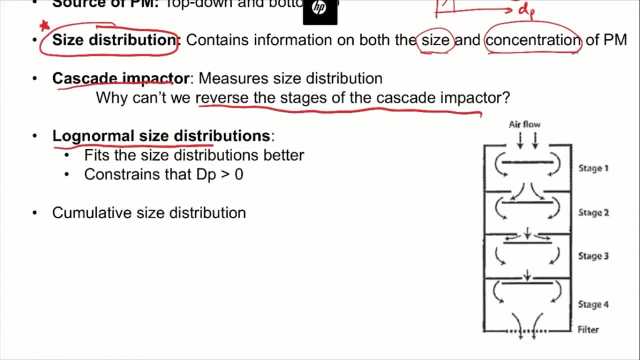 will just lose the size information. So after we have the size distribution we are going to move to the next slide. we mentioned that actually most of the PM in the atmosphere they will follow log-normal size distribution. People use these distributions quite a lot, right? So 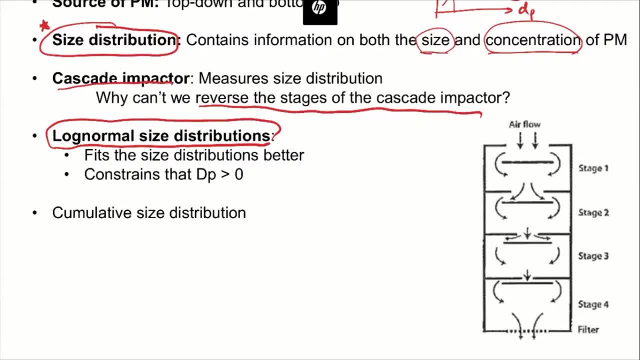 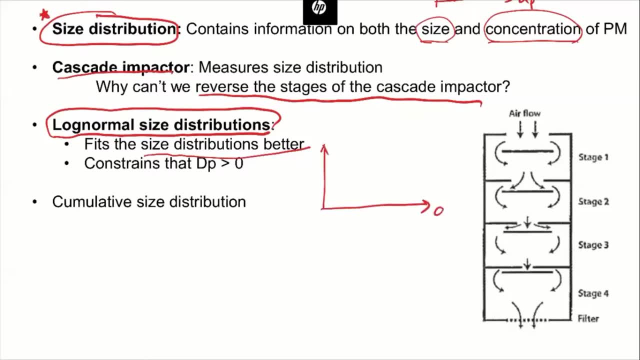 instead of using Gaussian we decide to use log-normal distribution, on one hand because it fits the size distribution better, because when we plot the size distributions, so the x-axis will just goes according to the log scale, right and normally the PM in the atmosphere, they will show size. 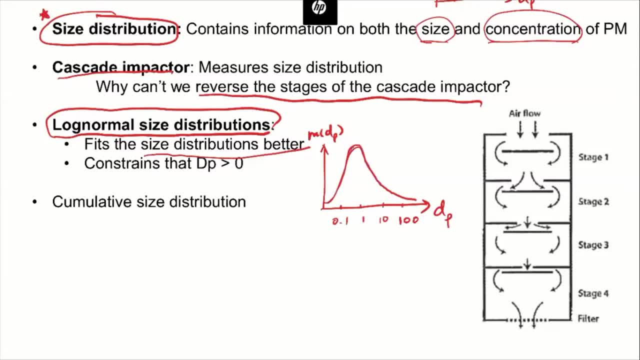 distribution looks like this: okay, And under this situation we can just easily use a log-normal size distribution to fit it right. But on the other hand, the log-normal distribution constraints that the DP have to be always larger than zero because we use Gaussian. and then if it's in linear scale, let's say 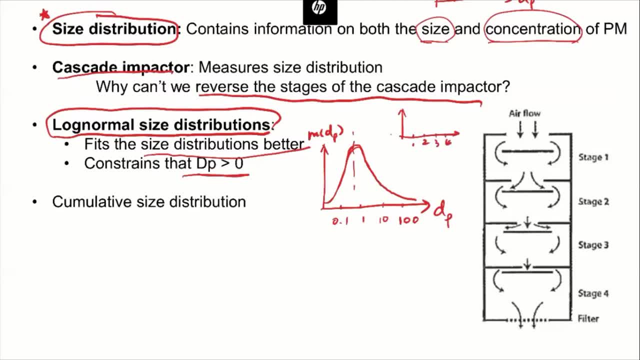 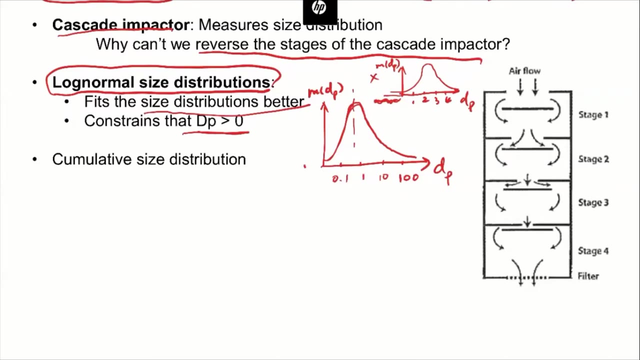 one, two, three, four. then it will have the scenario when DP is smaller than zero, right? So for this part, we just cannot explain it. that's why we don't want to use the Gaussian, but instead use the log normal, because even if we go across the x-scale, then it's. 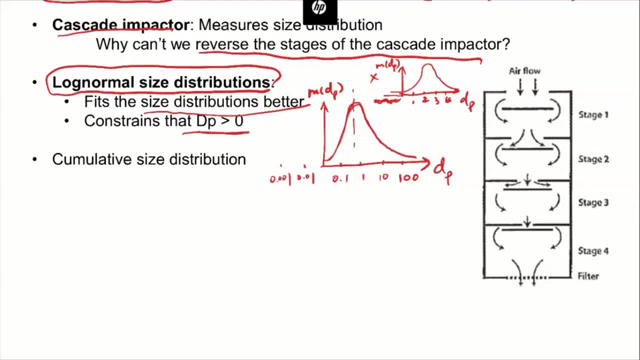 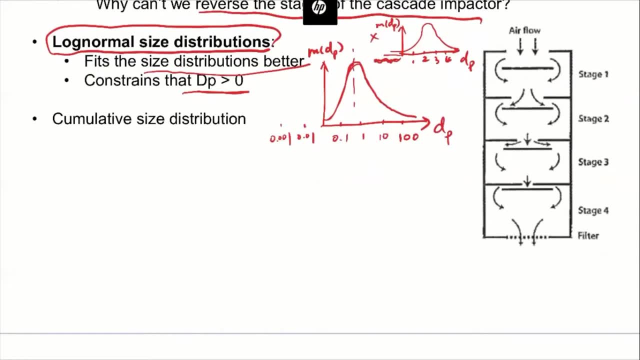 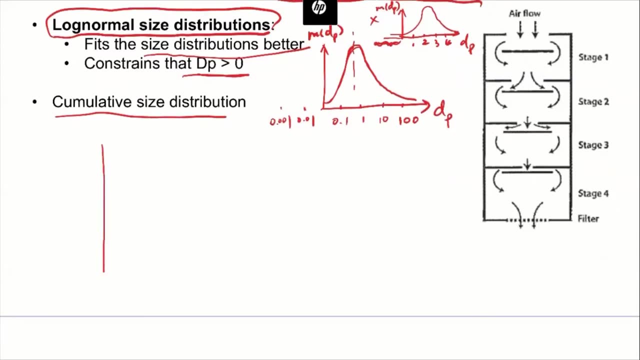 just going to be 0.01.. It's never going to reach to zero, So once we know the log, normal size distribution. finally, we'll mention something related to the cumulative size distribution. The cumulative size distribution just shows the fractions of particles below certain. 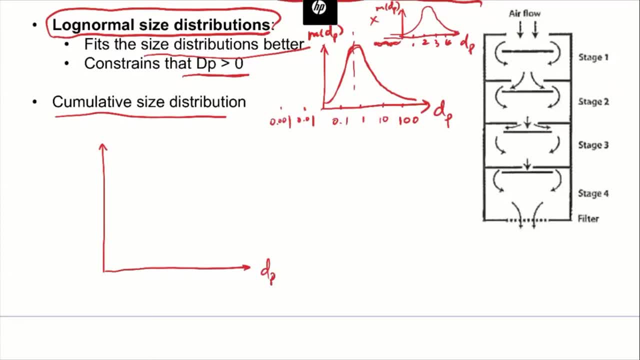 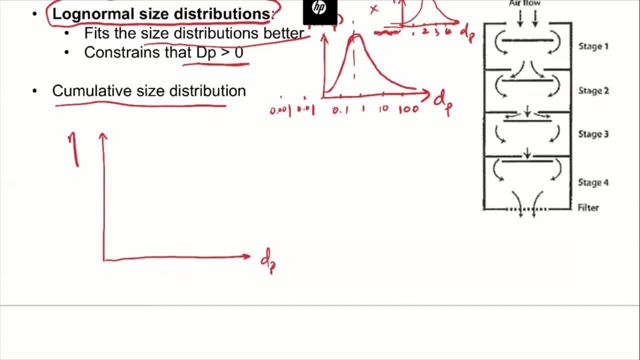 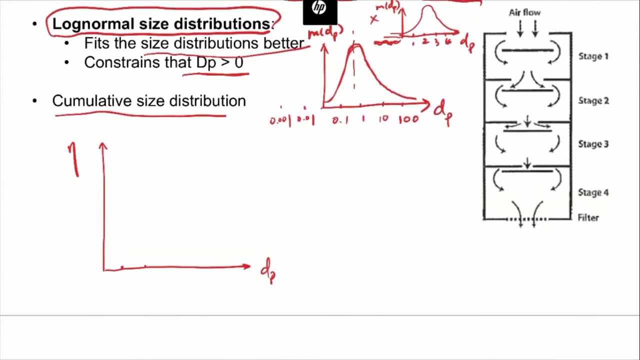 sizes Just shows the fraction of the particle below certain sizes. So, for example, if we still plot it in the log scale, it's going to show something like this: At the maximum size, the cumulative fraction would be 100%. Well, at the 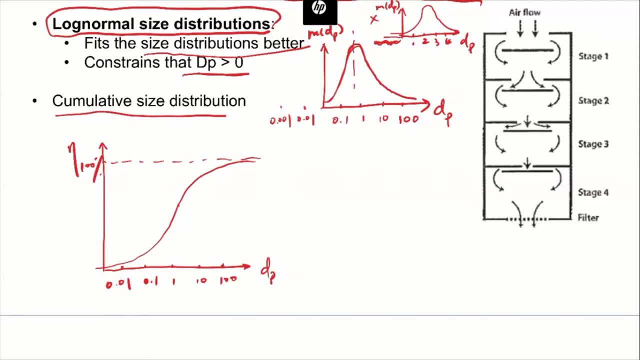 smallest size, the cumulative fraction will be almost zero And because the size distribution have a shape like this, since we're adding them up together, so it's going to grow faster at the near to the peak, or near to the peak size of the distribution. 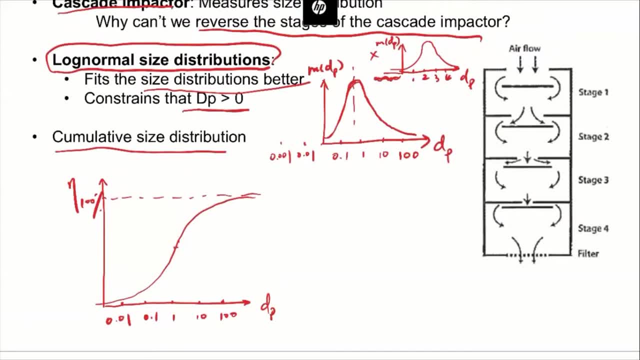 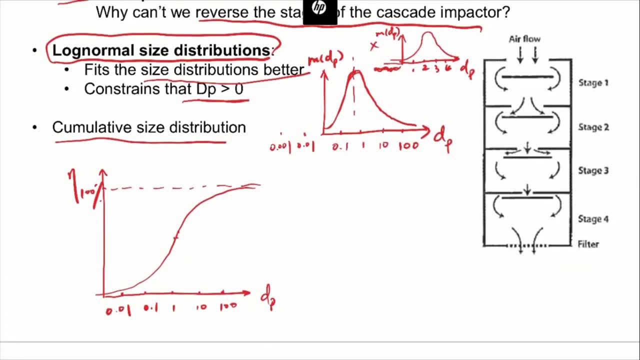 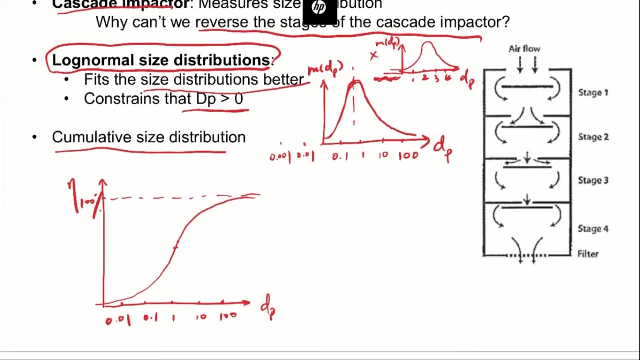 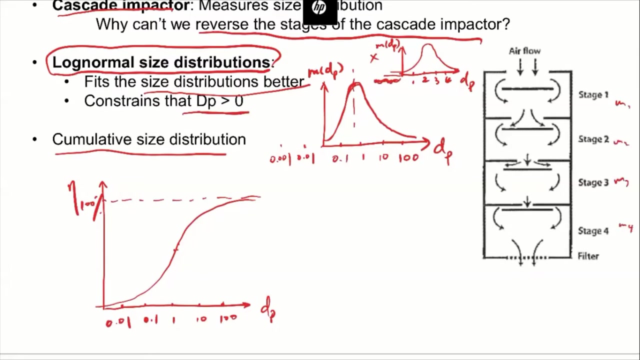 So it's going to show like this. So then we may have a question, because for a lot of actual applications we will try to. let's say we need to try to see whether a size distribution follows log normal distribution. Of course we can do the cascade impactor measurement. Let's say we measure M1, M2, M3, M4, so on and so forth. 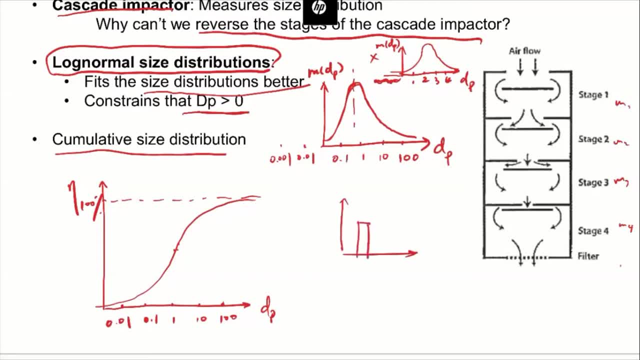 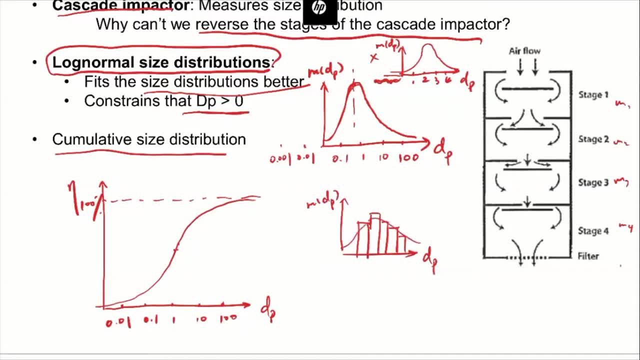 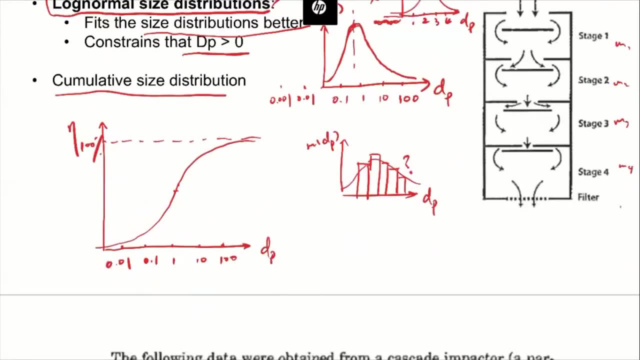 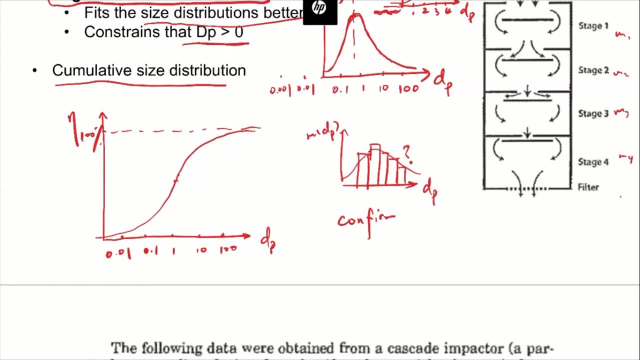 And use a curve fit to see whether it follows log normal or not. But there are actually easier ways to confirm whether a size distribution follows log normal. Size distribution follows log normal, normal. So there's an easier way in engineering to confirm this. okay, So for. 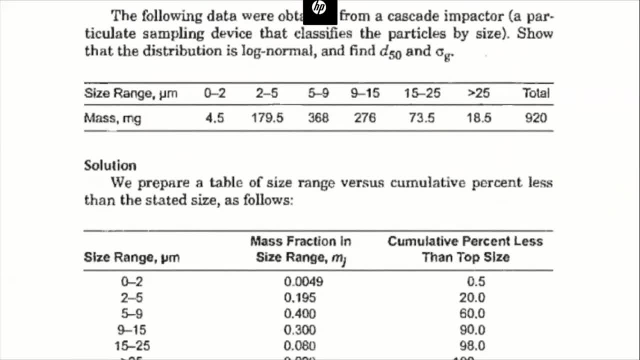 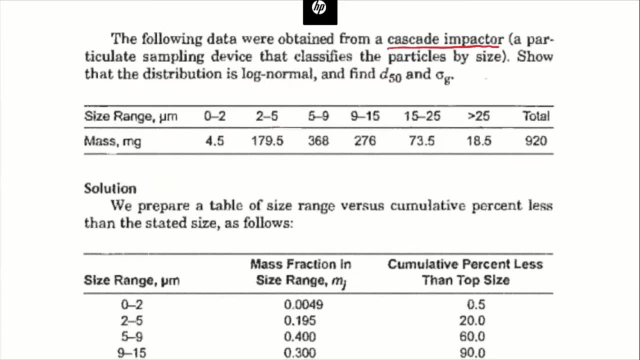 example. let's look at this problem here. So the following data obtained from a cascade impactor: okay, So, since we already introduced that. so basically, the cascade impactor is a particle sampling device that classifies particles by size, right? So it wants us to show that the size distribution or 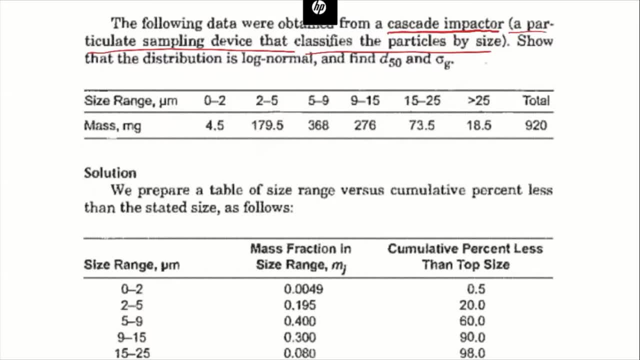 this information here below, so it shows that the size distribution is lognormal and it wants us to find the DP D50, which is the particle size that has a cumulative fraction of 50%, and the sigma G, which is a standard geometric standard deviation. okay, So this is an information. it provides us. 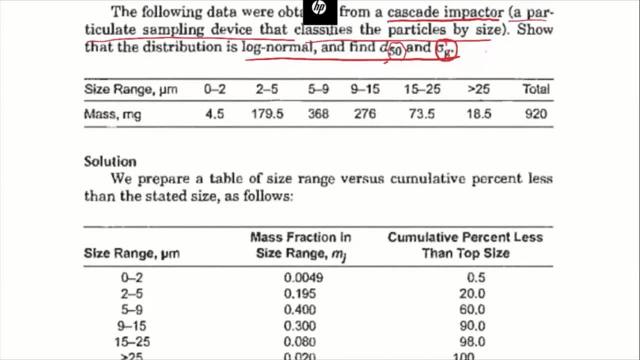 So, based on the properties or functionalities of the cascade impactor, basically tell us what is the mass of the particles in certain size range. right, For example, 0 to 2 micron, The mass is 4.5, 0 to 5 as this value. So 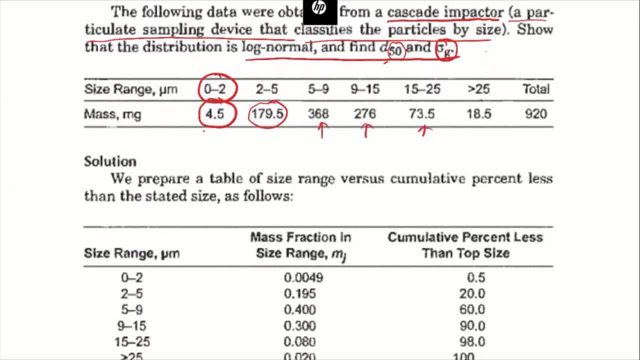 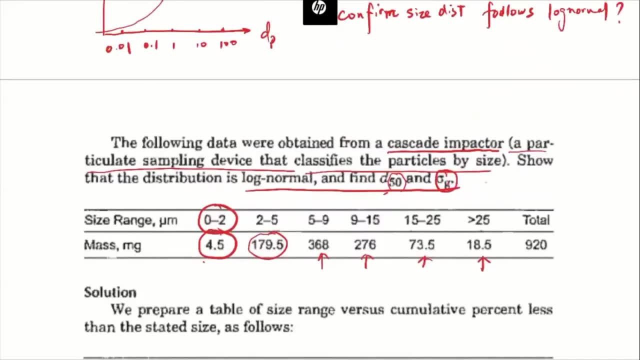 different stage will give us different mass right. Finally, above 25 micrometer, we have this mass. So if we correspond to an actual impactor, then this is going to be stage 1, right. Stage 1 has a cut size of 25 micrometer. 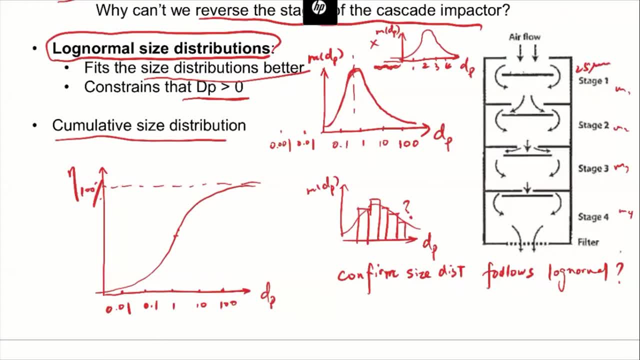 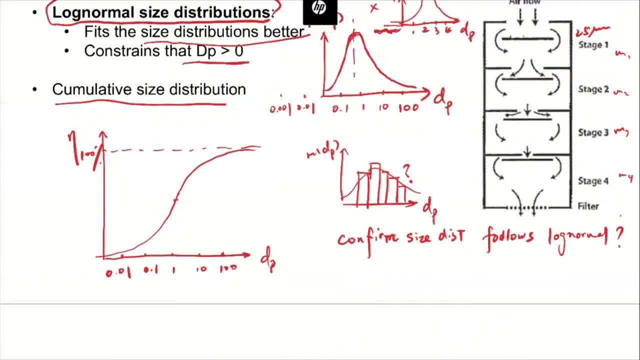 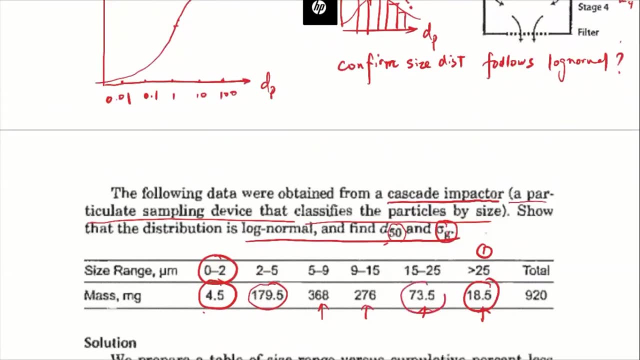 So all the particles above 25 microns are going to get collected here and we can measure its size. So the second stage has a cut size of 15 microns. So that's why here we can measure its mass. That's going to be 15 to 25, right? 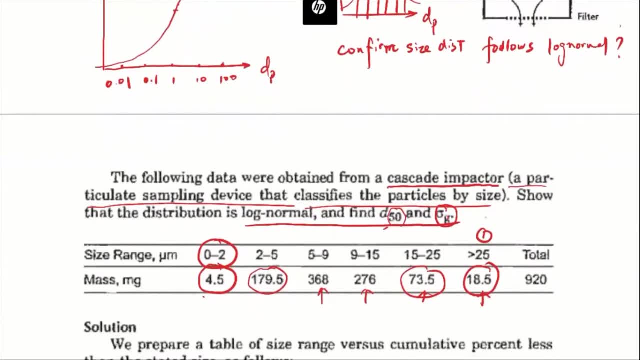 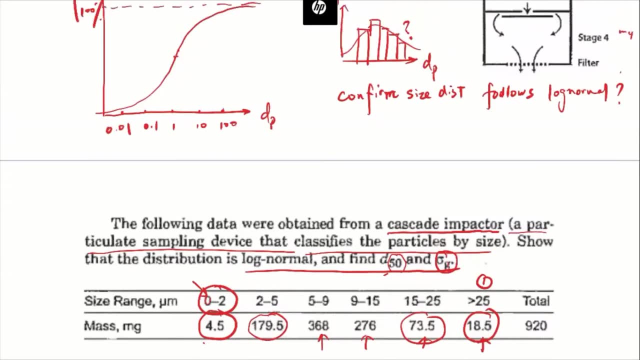 So, so, on and so forth, We can get all of this information. So, finally, for 0 to 2,, of course we cannot find a stage that has a cut size of 0. So the way we measure that is by letting the remaining particles go through a filter. 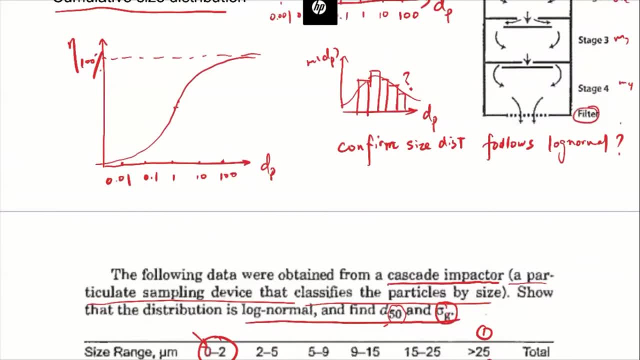 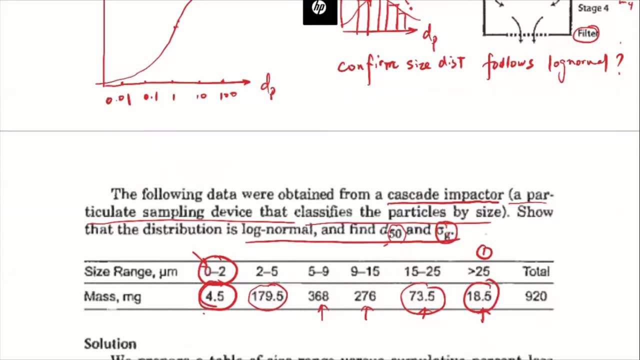 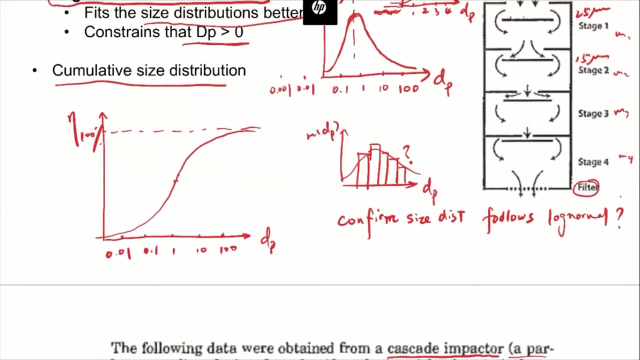 So the filter will collect all the particles that remain. This will give us the mass for the smallest particles. So now it wants us to confirm that this size distribution follows a log-normal size distribution. And it is quite challenging If we just plot it in this way. it's difficult to tell. 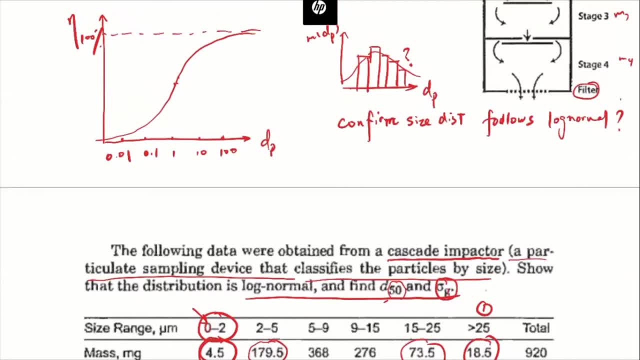 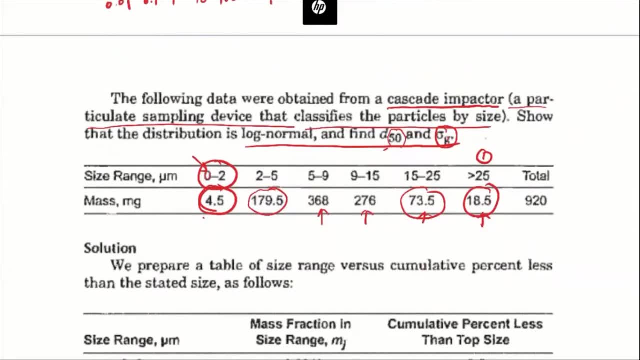 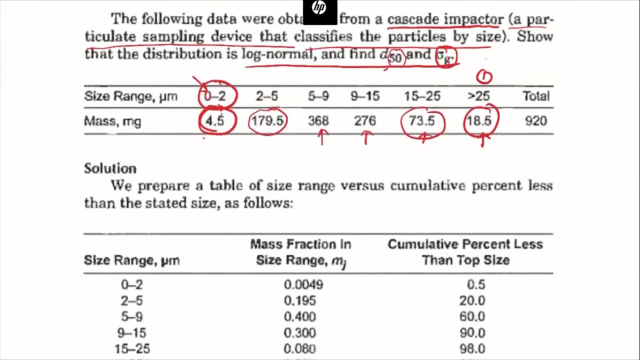 So the way we do it is to confirm it with the cumulative fraction. So we're going to first calculate what is the cumulative fraction of particles below 2, below 5, below 9,, all the way below 25,. okay, So the way we do that is: first, let's say we list out the cascade, impactor stages 0. 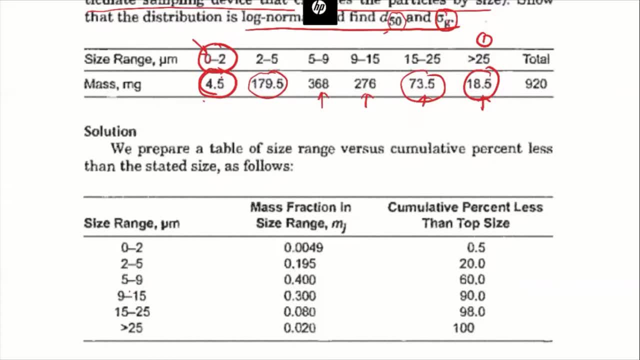 to 2,, 2 to 5,, 5 to 9.. 9 to 15,, 15 to 25, and above 25.. So we can list out what is the mass. And we have 44.5.. 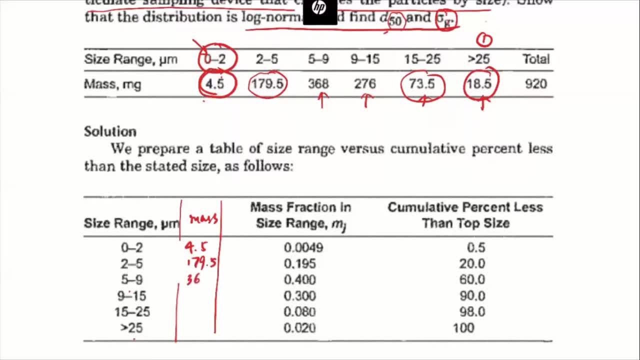 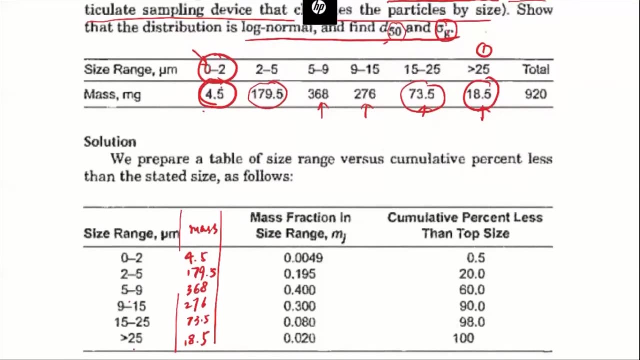 I'll just copy all of these numbers here. Okay, So with this mass information, we can first calculate what is the cumulative fraction. Okay, So, the way we do it, what is the fraction of the mass that's within this single bin here? 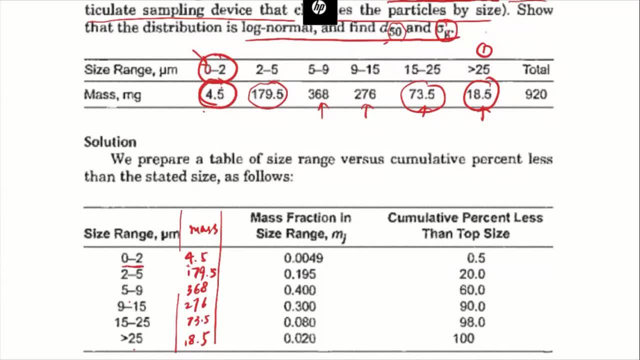 So the way we do that is, we can divide these numbers by 920, which is the total mass. Okay, So if you do the calculation, basically, this is going to be the value you have. Okay, Divide by 920. Okay. 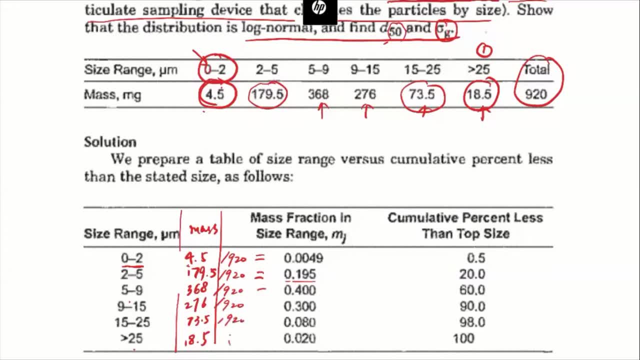 So this is going to be the value you have. Okay, Divide by 920.. Okay, So this is going to be the value you have. Okay, Yeah, Then we need to calculate a cumulative mass fraction. So the cumulative mass fraction is just the mass fraction of particles below a certain 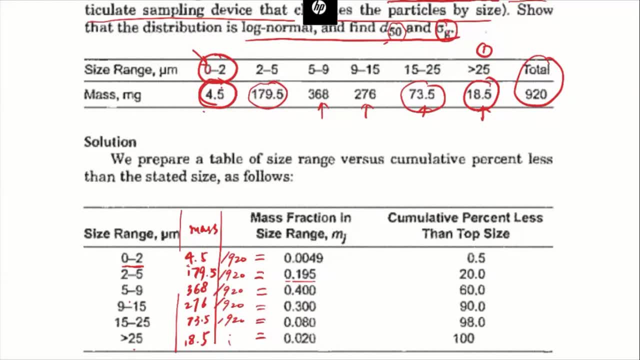 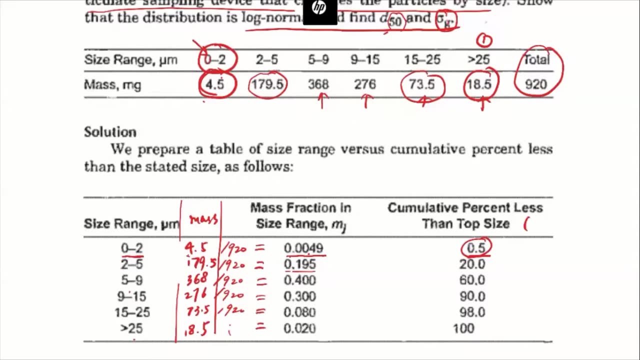 size Right. For example, below 2 microns. that's just going to be this value, Okay. So the percentage is going to be .49%. So here on the textbook it's just rounded to .5%. Okay, And then the cumulative mass fraction: right? 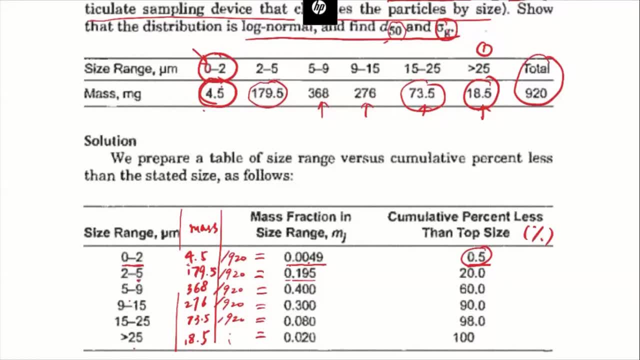 Cumulated mass fraction of particles below 5 microns are just going to be these two values added up together. right, These two add together, you have 20%. Okay, so the cumulative mass fraction particles below 9 microns are going to be these three adding up together. 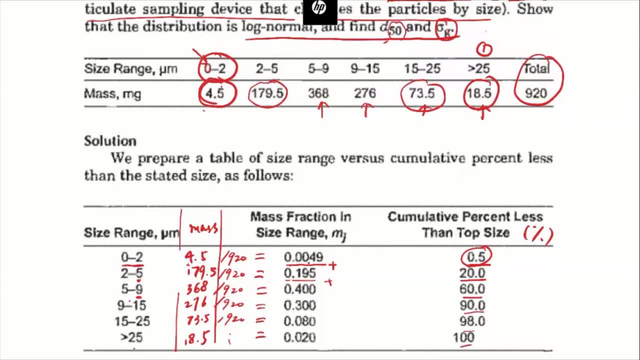 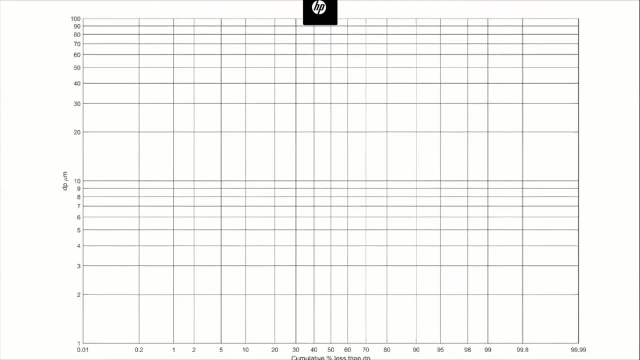 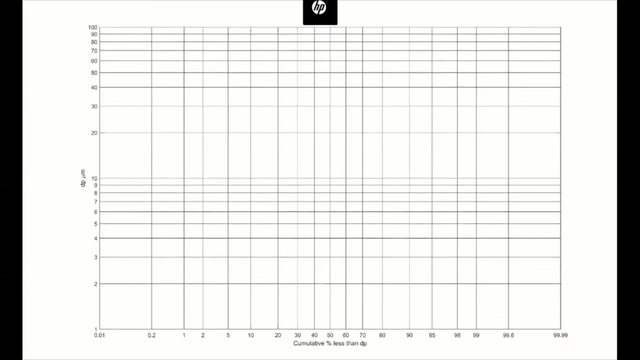 60%. So 90%, 98 and you 100%. Okay, so once we get the cumulative mass fraction, We can use a plot called the Semi-log plot. so here I'm showing the plot here. Maybe it's a little bit. Let's just zoom out a little bit, Okay? so this is the 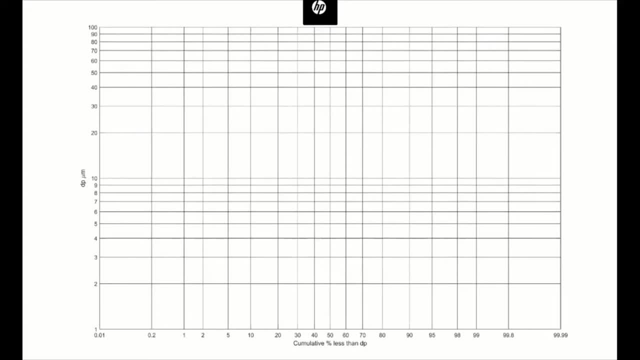 Engineering plot that people use a lot to tell whether Size distribution is log, normal or not. Okay, so they're. on the x-axis is Accumulated fraction of particles below certain size and on the y-axis is the particle size. Okay, so what we're going to do is? 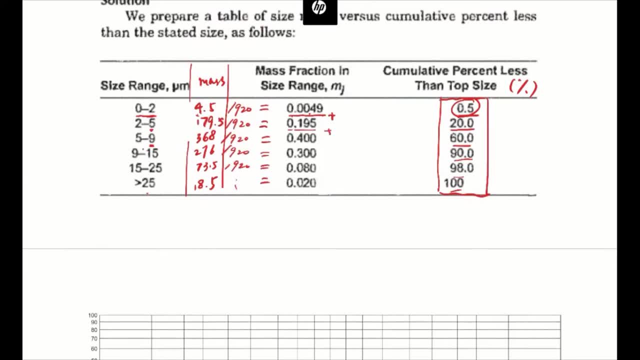 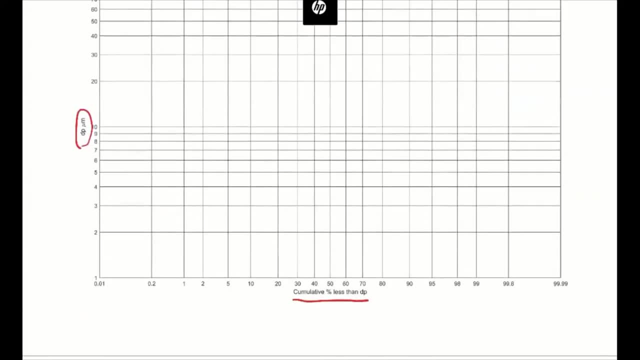 We'll just plot the data points. Let's say, the cumulative mass fraction of particles below 2 is 0.5. So we're just gonna add a point corresponding to 2 micrometer and then Find out the 0.5.. Okay, so 0.5 is going to be. 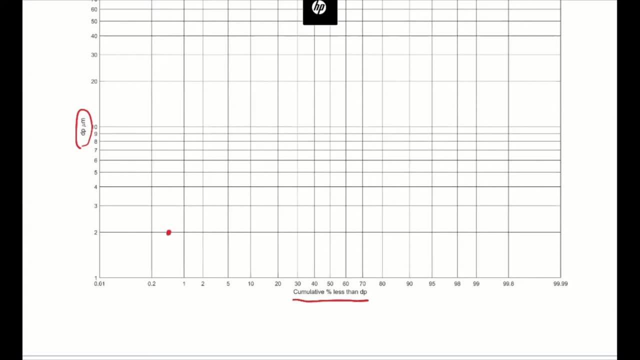 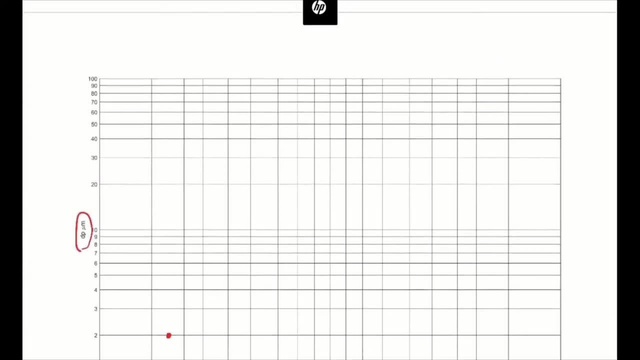 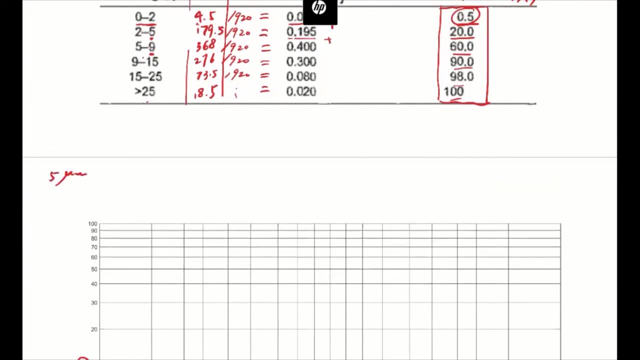 Somewhere. let's say here: Okay, this is the percentage Fraction right, 2 micron correspond to this point. So let's do the remaining data points. I'll just first copy the numbers here: 5 micron, 20, 9, you have 60, 15, 90. 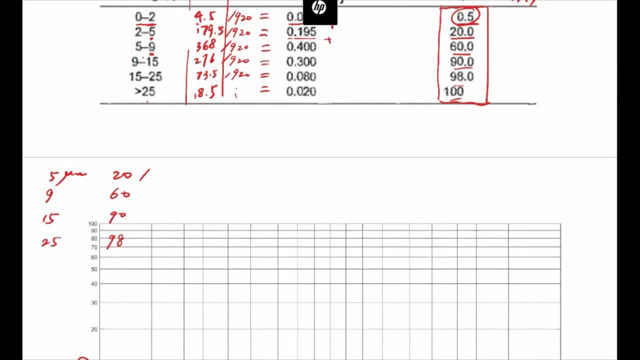 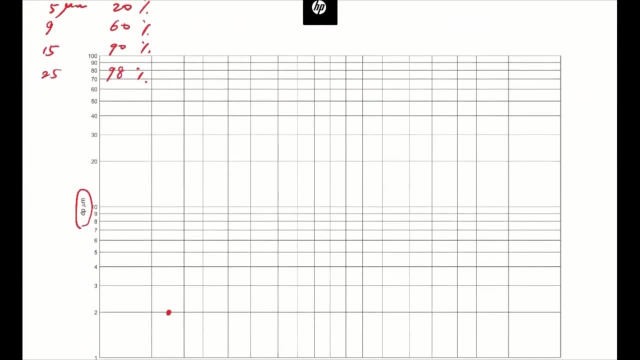 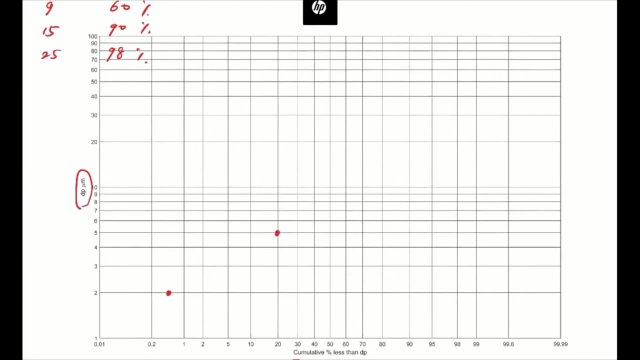 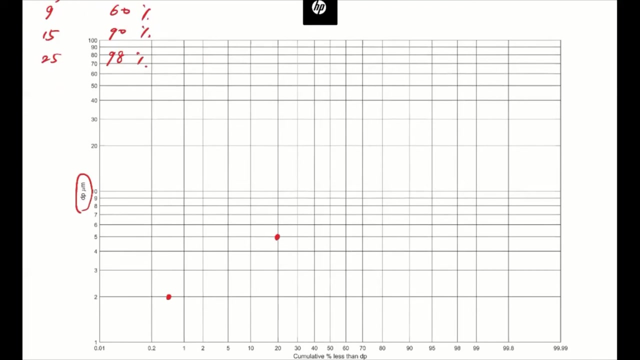 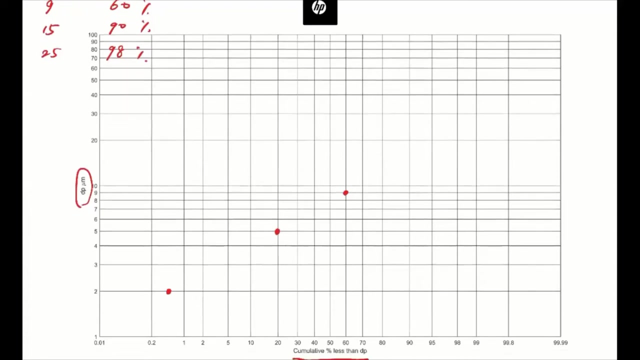 25, 98, Okay, And then we have a lot of points. So let's plot the remaining points. at 5 microns, we need to find 20%, Which is here Right. and then 9 microns, we have 60 percent. 15 micron- that's somewhere here, right We have, we have 90 percent. 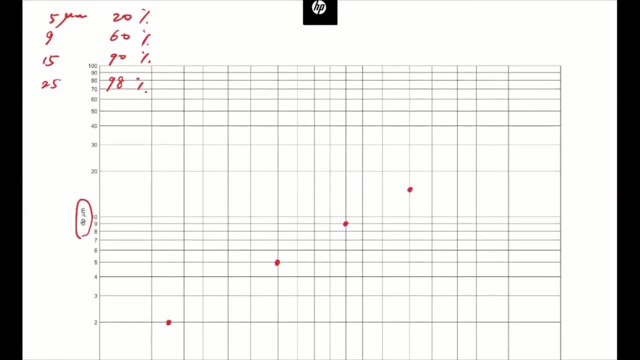 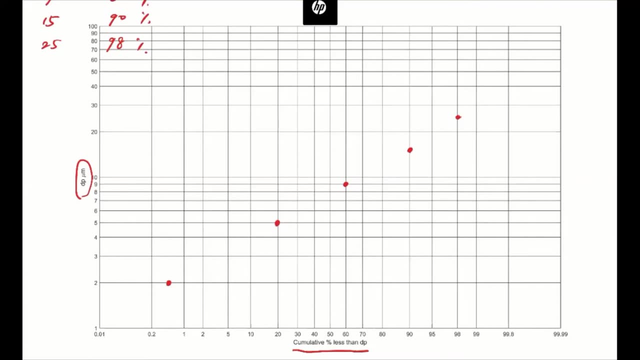 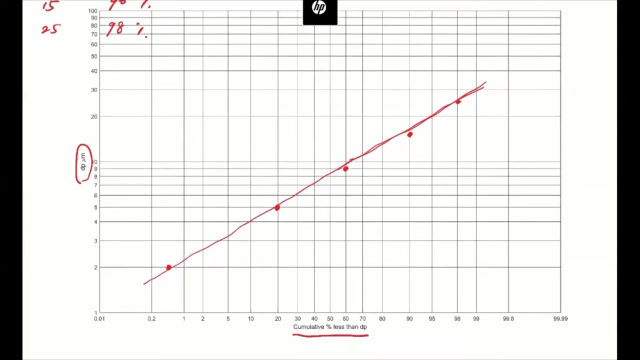 and then at 25 we have 98. okay, so now. so the engineering plot, or semi log plot. make sure that if it's a log normal size distribution it's going to follow a straight line. okay, it is almost very close to a straight line here, so that's. 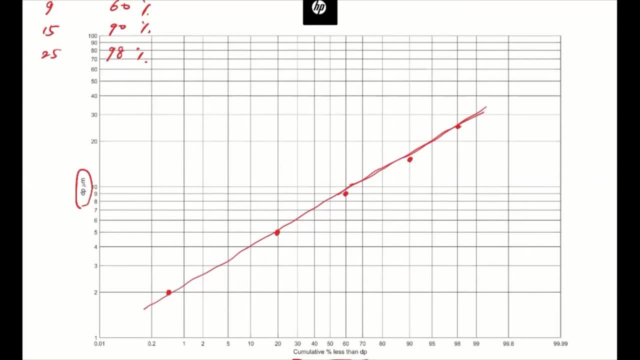 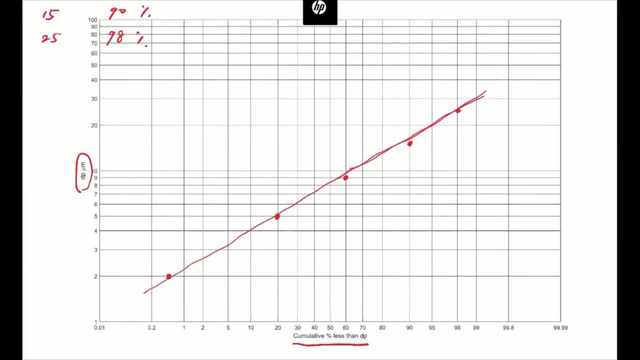 why it is a log normal size distribution. okay, so if you look at further, take a look at the, the semi log plot. it is a little bit different from the most commonly used semi log plots. on the y-axis it's still log normal scale, right? you have 1 to 10, 10 to 100. they have the same gap here, right? but on the 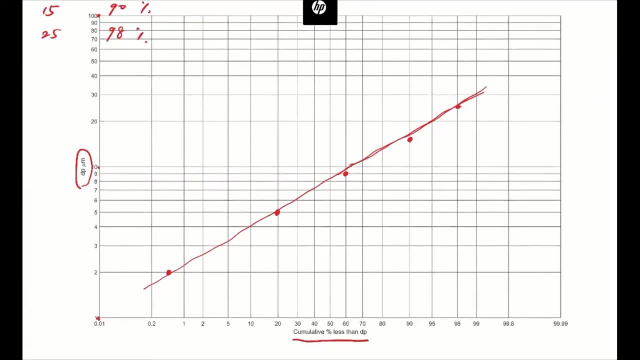 x-axis for the fraction. it's not in linear scale, right. so you see that the fraction that's close to the fraction, that are close to 50%, they're more crowded, but the fractions that are very small or very large, they're stretched right. so this kind of makes sense because 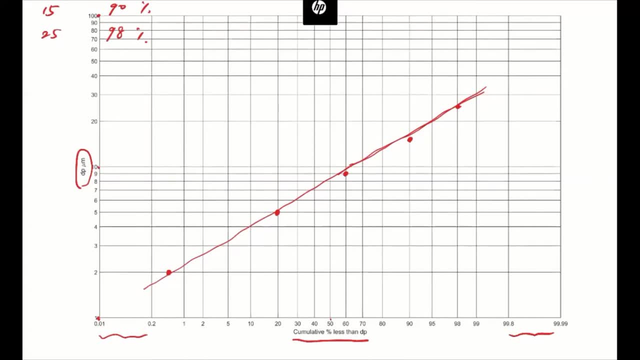 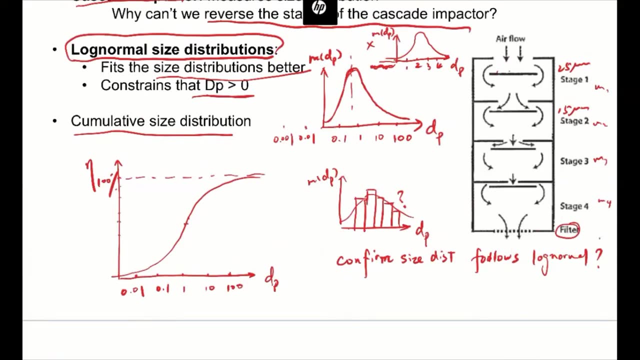 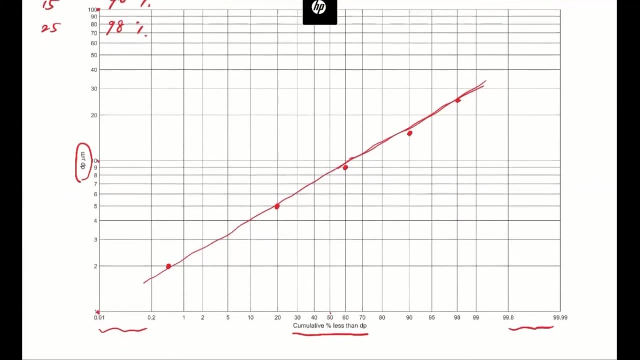 theoretically, if this scale is linear, if this scale is linear, it's going to look like this plot, right? if it's linear scale in the fraction, then it's going to. it's not going to show a straight line here, right? so we may have a question. so why is it? why is this plot so magical, right? 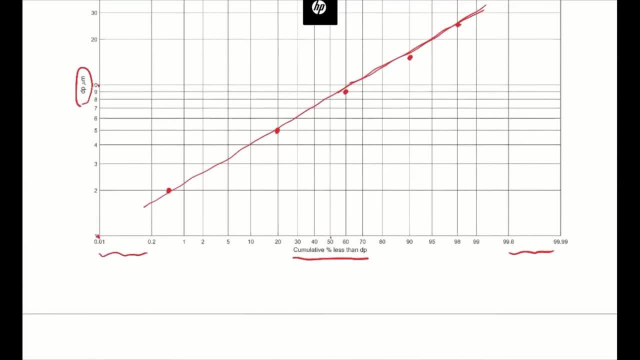 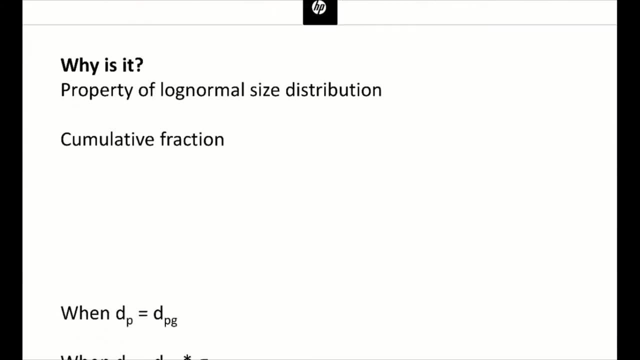 so this has to deal with the. so basically, these are the data points again, right. so it has to deal is because of the properties of these log normal size distributions. so so, last class, we show that actually the log norm size is a vertical line, one is a horizontal line and the vertical line is a vertical line. 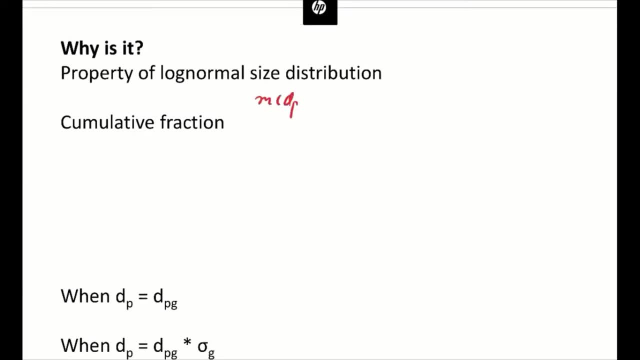 so if you look at the data points in between these two classes here, you can see that these numbers, this and the log-normal size distribution follows the equation of m total divided by square root of 2 pi dp sigma g Forgot a log here. log dp minus log dpg divided by 2 log of sigma g squared. 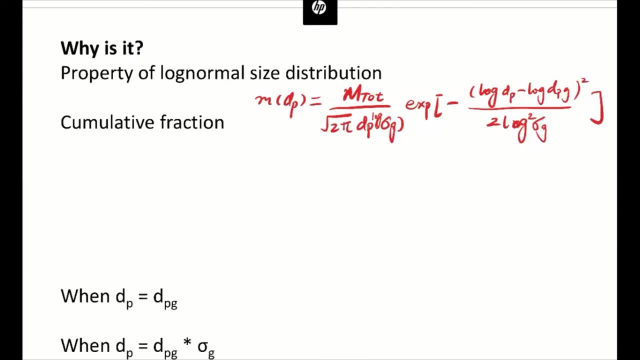 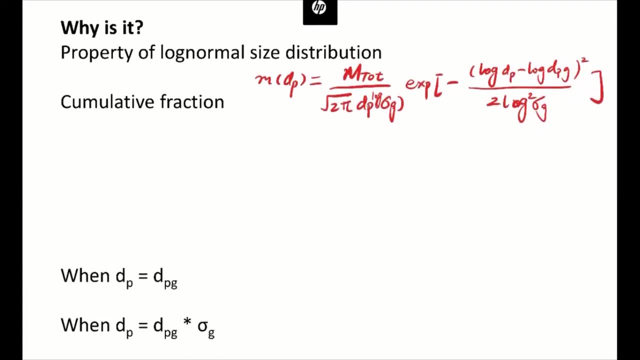 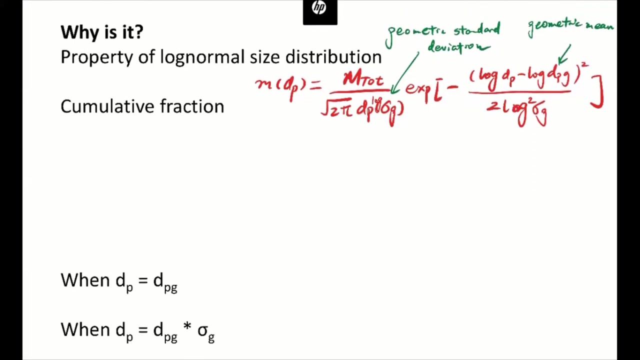 So last class we showed that the log-normal size distribution are going to follow an equation that looks like this, And so basically, in this equation we mentioned that the sigma g is the geometric standard deviation And the dpg is called the geometric mean. So for log-normal size distribution, if we calculate its cumulative fraction, we should: 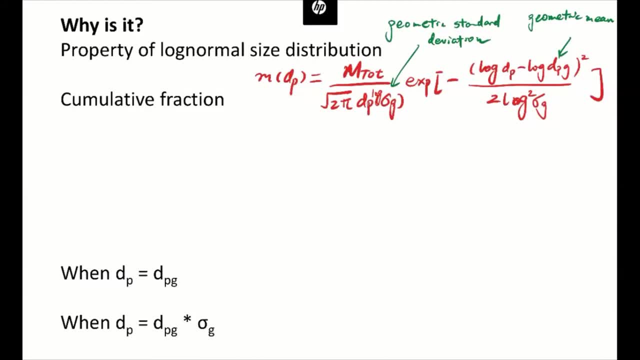 know how the cumulative fraction works, Right? So it's just an integral. let's say 0 to, let's say this way. So this is how we calculate the cumulative mass fraction, Right? Okay? So basically it's according to the definition, right? 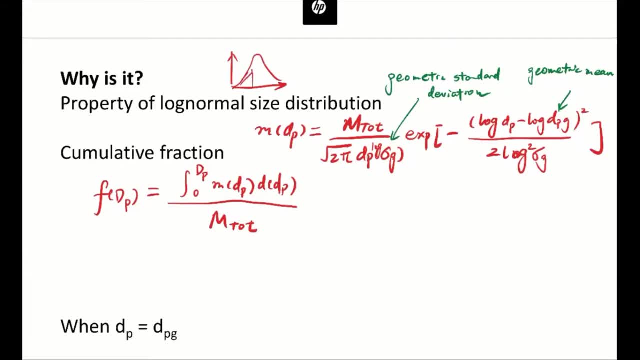 So we have to integrate. we have to integrate the area that's below the size distribution and divide that by the total area or the total mass. So the total area will be mass, total right, And then we just need to calculate what is the mass that's below this certain size. 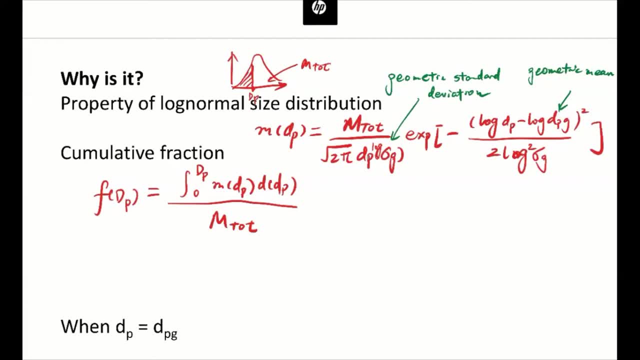 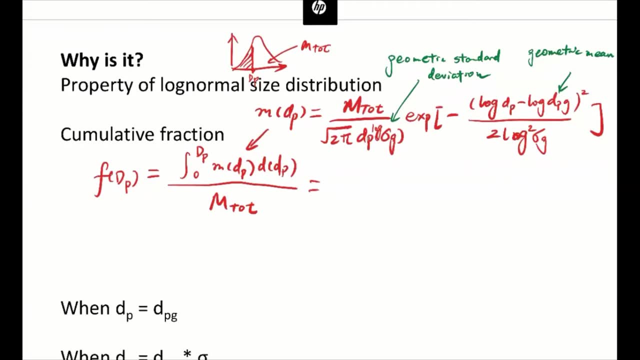 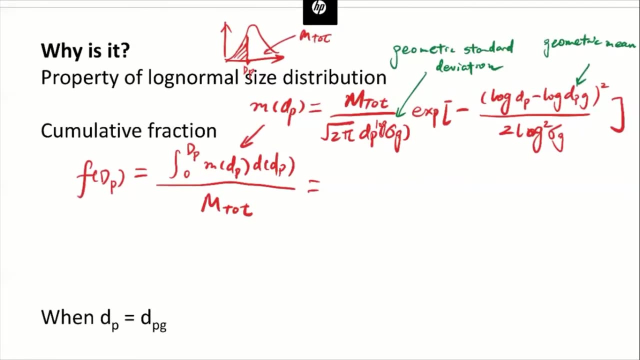 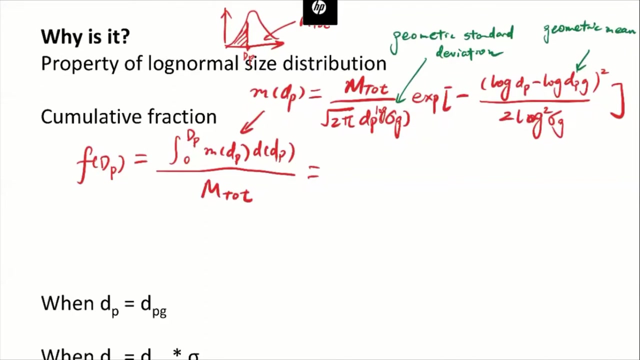 This is how we should calculate the cumulative fraction. So if you plug in this equation to the integral, I'll just skip it for this class. If you want to know more again, go to your cumulative calculus class. okay, So the final solution for this equation is actually this: 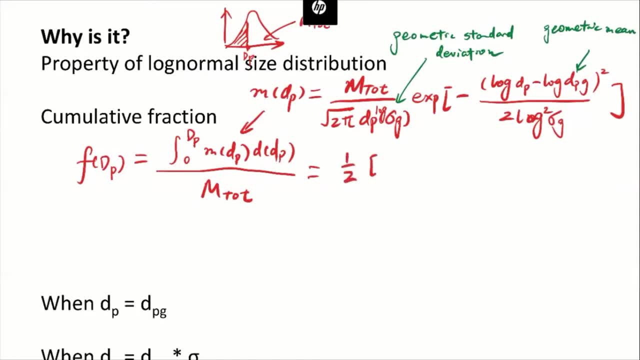 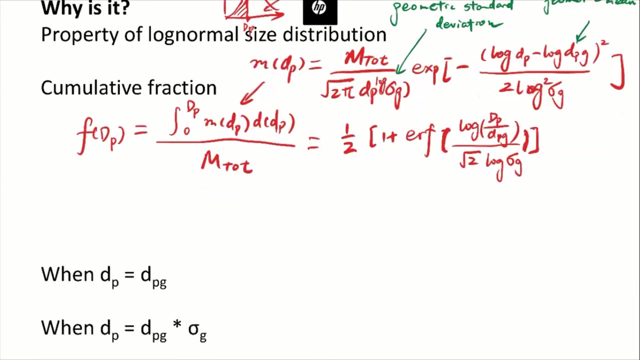 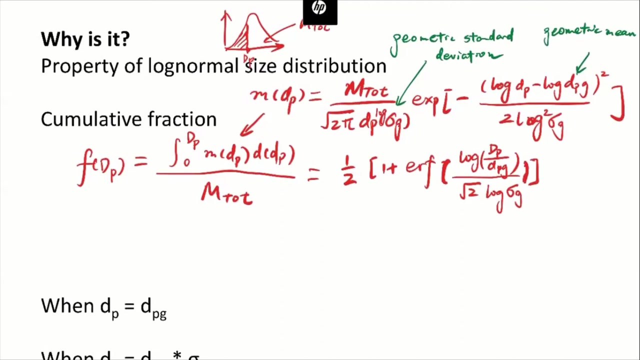 So it's 1 over 2, 1 plus error function. Okay, Okay, Log dP: dPg divide by square root of: okay, So the final solution looks like this- Okay, little bit scary, I would say, because we're dealing with another function- that 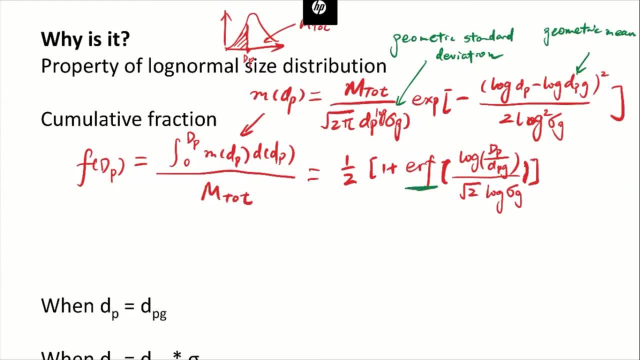 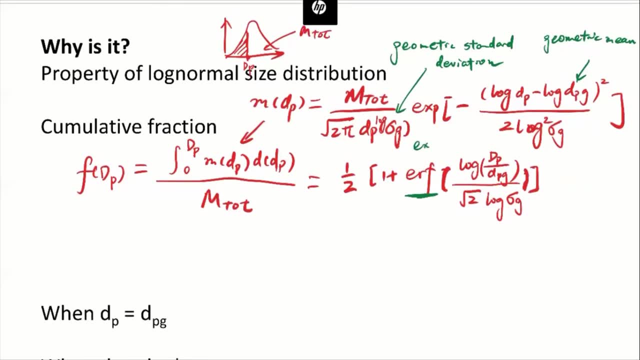 we're not quite familiar with. Okay, so this is called the error function. So the error function, you can just regard it as a symbol. Okay, so it's similar to, let's say, exponential or log. Okay, so it's just a way of representing. 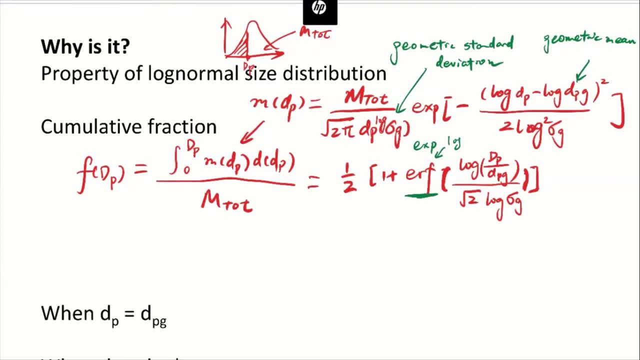 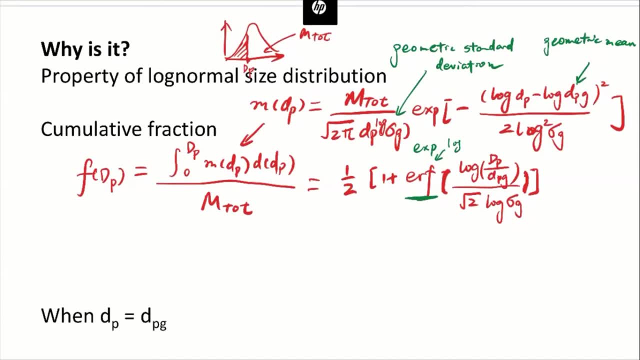 a calculation process. Okay, so now you can see that the cumulative fraction, cumulative mass fraction- depends on three parameters. So it depends on the size we are interested in, right? Let's say, if we want to calculate the cumulative mass fraction up to 10 microns, then this capital DPU will just. 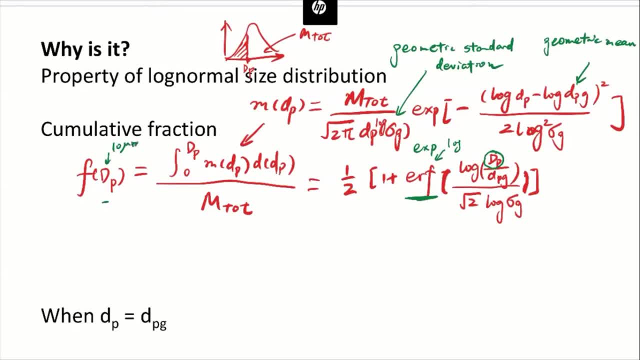 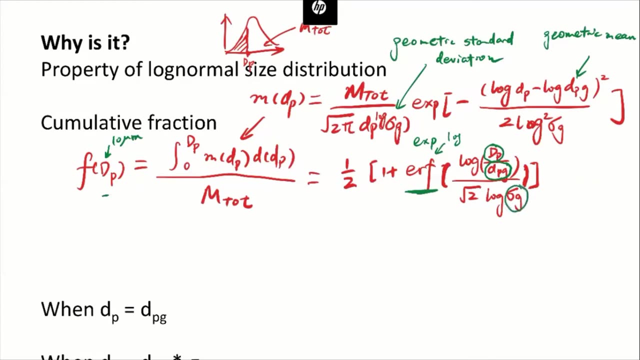 be 10 microns, Right? So this is a size that we're interested in. So it depends on the geometric standard deviation. It also depends on the geometric mean. It also depends on the geometric standard deviation. So it depends on these three. 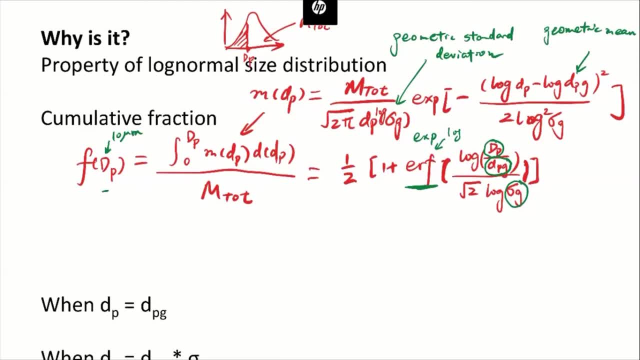 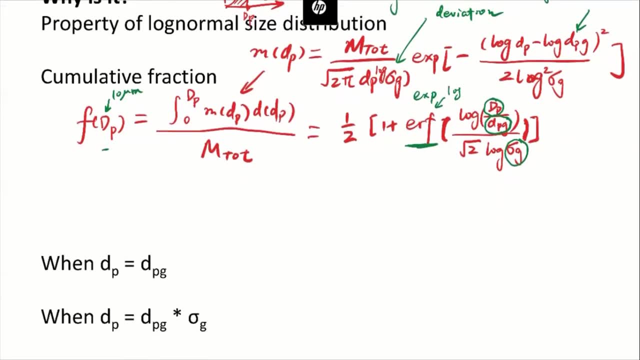 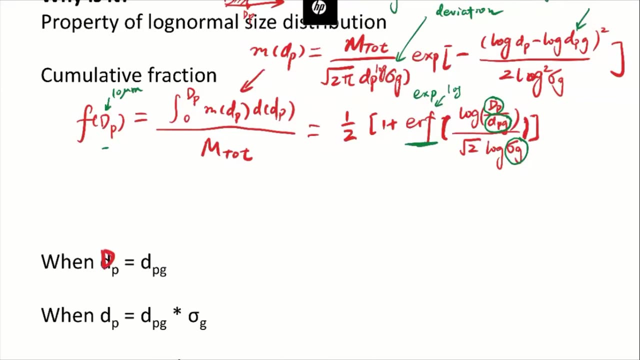 values here. But one thing we can know for sure is that it is quite special, under three conditions. Okay, for example, when we use theboutest bars, once we multiply the left and ¿ quanto do we avoid the cost and the front of the given shape? When Dp we should use capital D. 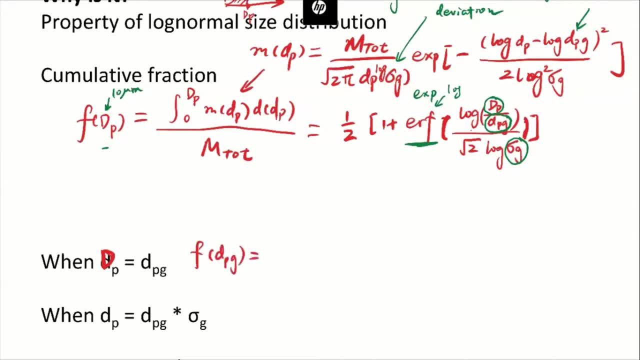 here, When Dp is equal to dpg, then we know that the log transform will become log one, right? So basically, this cumulative fraction will become 1 over 2,, 1plus our function of log 1, divided by something in the denominator. right. So log 1, dPn, dpG is a double derivative, derivative right XZ is part of it. So we sing those two terms and instead of log 1 it's equal to dash. very soon, cross-segmental know to you will see that in here. 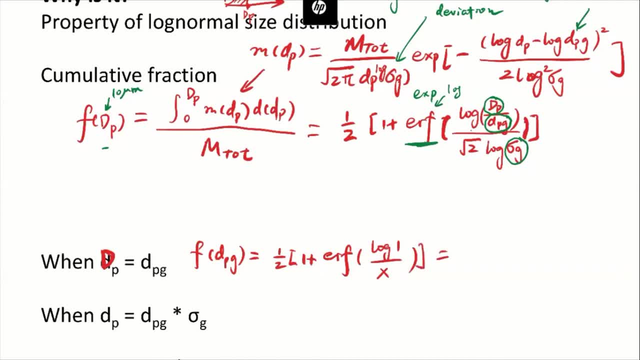 it must be exponent of 1.. The stay inz is equal to 1.. So what? you are, Ariel, right, it's only getting amount of Öyle and for a loss of a certain value, and you, one is equal to zero, and error function of zero equals to zero. 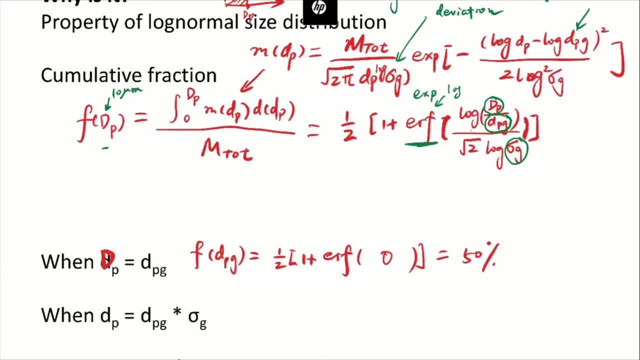 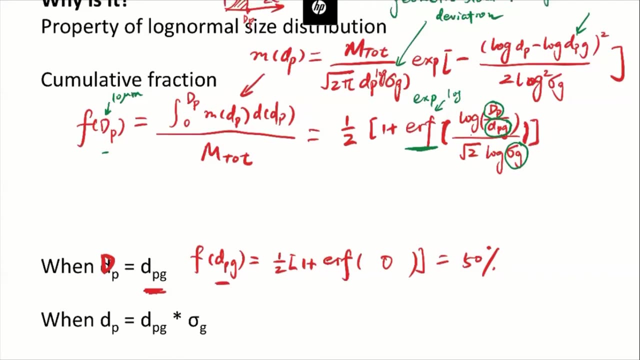 so that's going to be 50 percent. okay. so what this means is that when the size of interest we're interested in a size of interest is equal to the geometric mean, then the cumulative fraction will be 50 percent. so what does that mean? it just means. 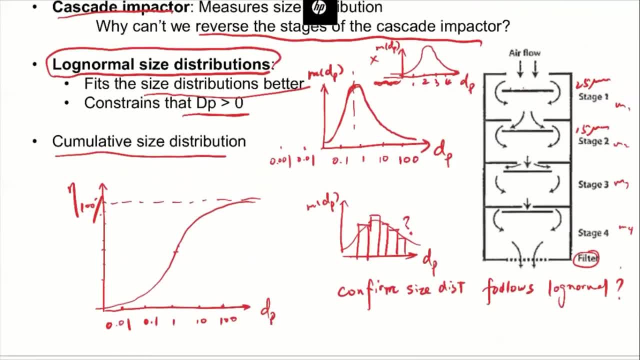 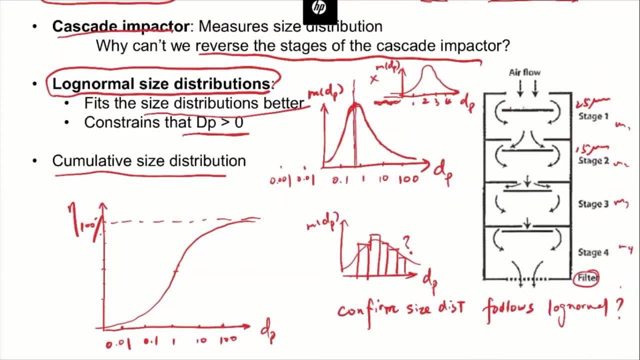 that let's say, if we go back to the size distributions, so the, the middle point or the axis of symmetry, will correspond to the size of dpg. so on the left hand side the mass fraction is 50 percent. on the right hand side the mass fraction is 50. 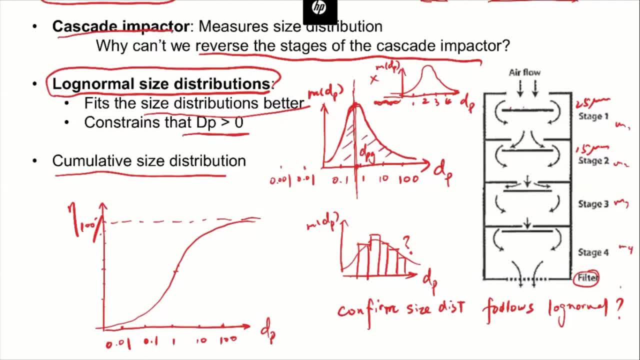 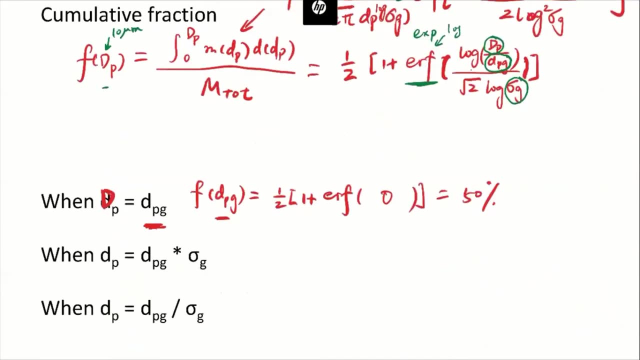 okay, so this is a special size. when the particle size is equal to the geometric mean, then basically the mass fraction on before that mass fraction after that are going to be equal, which are 50 percent. okay, so when dp dp equal to dpg, we have 50 percent. 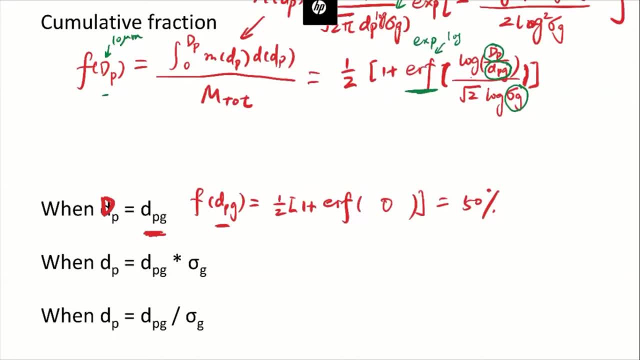 so the other point of interest is when dp is equal to dpg multiplied by sigma g. so if we plug in this term into the calculation so you can see that um on the g g will be equal to one plus error function of log sigma g. okay, if we plug in this dp into this equation here. 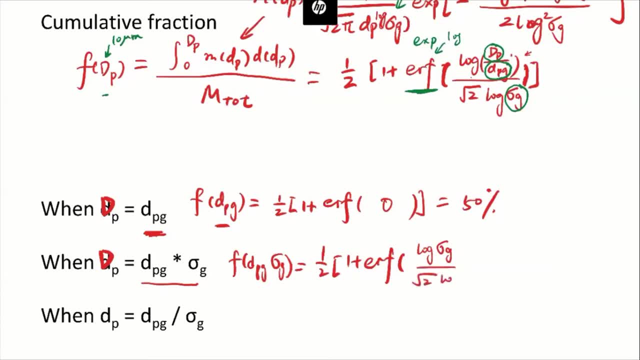 and then on the denominator we have a square root of two log, sigma g. okay, so these thing, these two things will cancel out. so we're going to get a constant value here. all right, that's 84.1 percent. so this will apply for all log normal size distribution. so if we 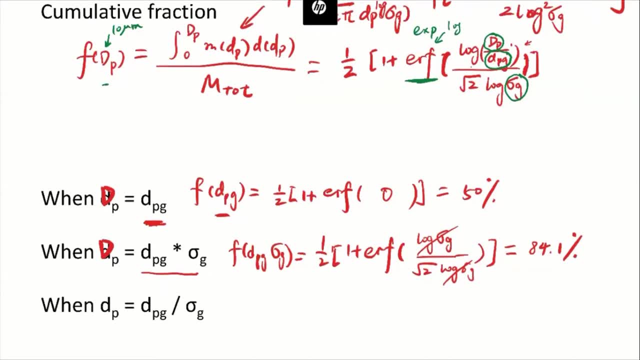 log our distribution, then if the size is equal to the geometric mean multiplied by geometric standard deviation, then the cumulative mass fraction will be, always, will always be, 84.1 percent. all right, so if a subsequent measurement we're going to do will give us exactly this length a, 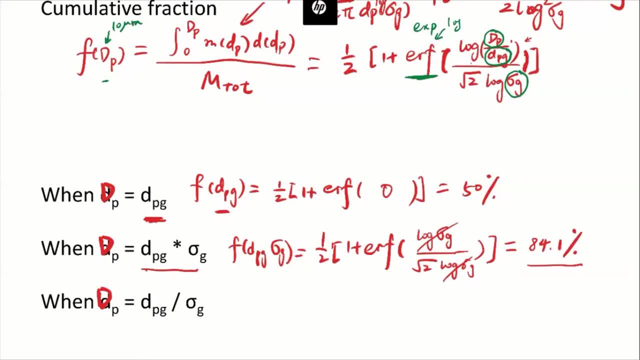 Similarly, if the particle size that we're interested in is equal to dpg divided by sigma g, we can do the similar thing. So dpg divided by sigma g, 2, 1 plus our function log, 1 divided by sigma g. So we know that log of 1 over something is just negative of that term, right. 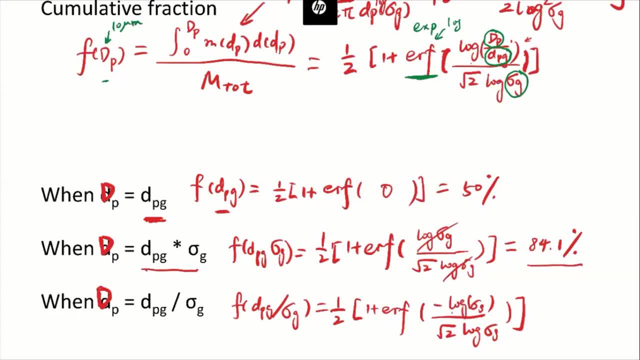 So we have negative log, sigma g. So again, these two will cancel out right. We just have 1 plus error function of negative 1 over square root of 2.. So this is going to have a value of 15.9%. 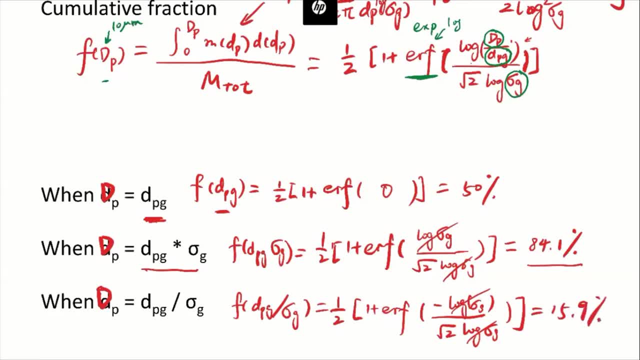 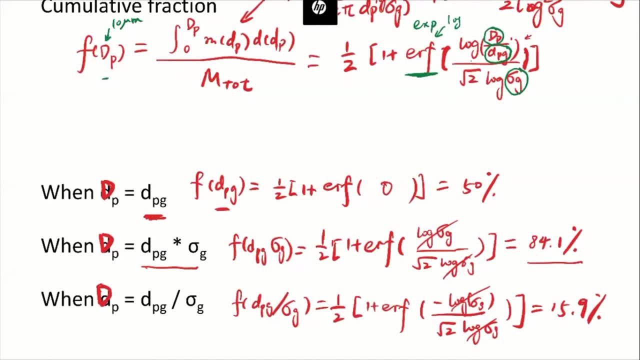 OK, So these are the properties of the log normal size distribution. So basically, if we have three different sizes, so it just applies for all different types of log normal size distribution. We always have the mass fraction when the particle size is equal to dpg, the cumulative. 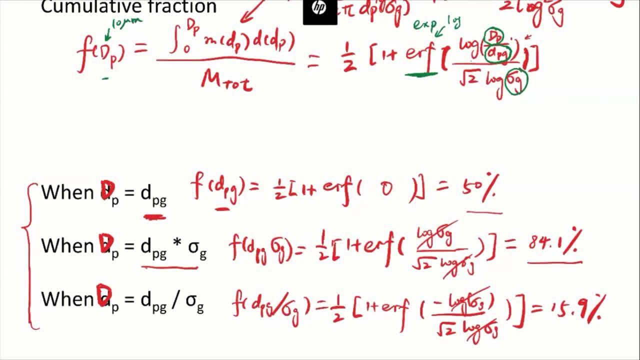 mass fraction is 50% When it's equal to dpg multiple. When it's equal to dpg by sigma g, the mass fraction will be 84.1, and when dp is equal to dpg divided by sigma g, the mass fraction is 15.9.. 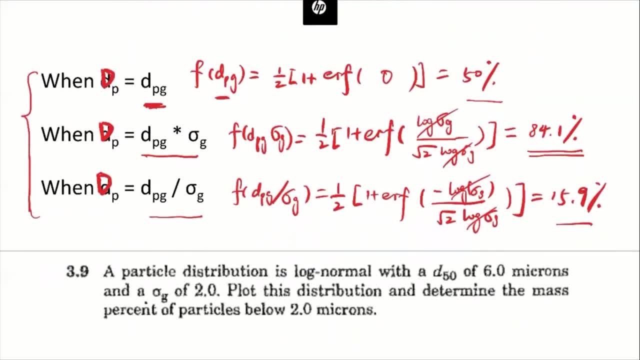 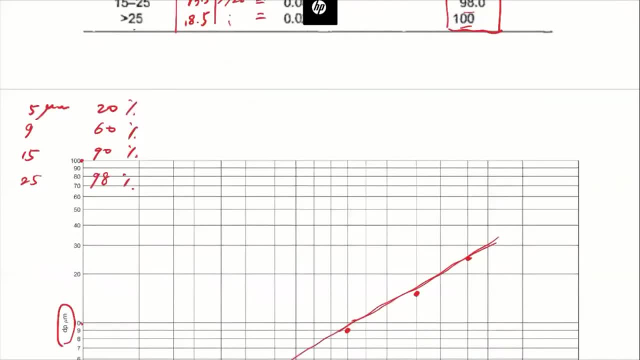 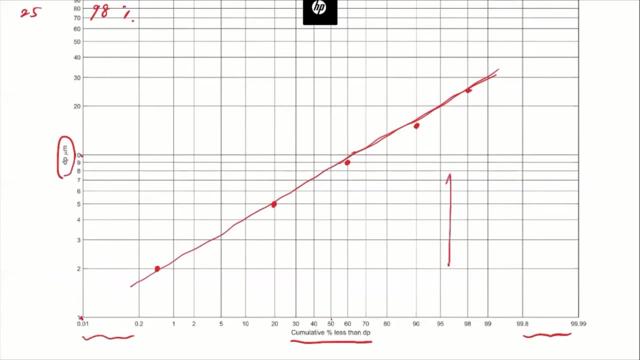 OK. So again, let's say, if we go back to the, I think originally we were trying to discuss why this is a case, right? So why is it going to follow a straight line here? So if you, basically, if you recall, 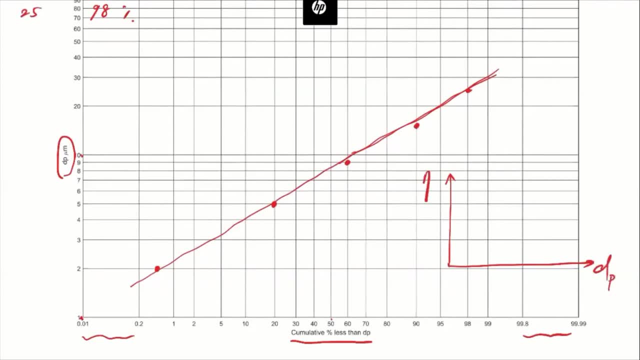 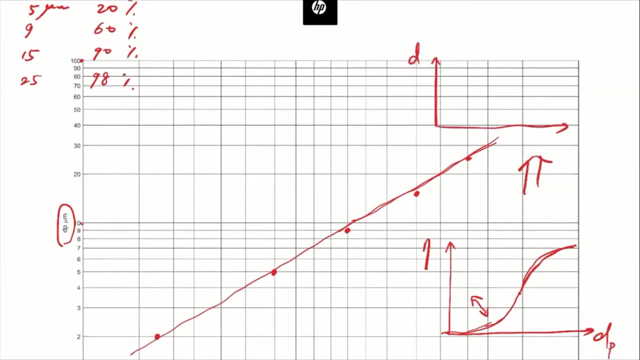 When we plot out the cumulative mass fraction, we had something like this: OK, So basically what happens is, for the log normal plot, we just switch the x-axis and y-axis. first Let's say: this is what we get, Then we know. 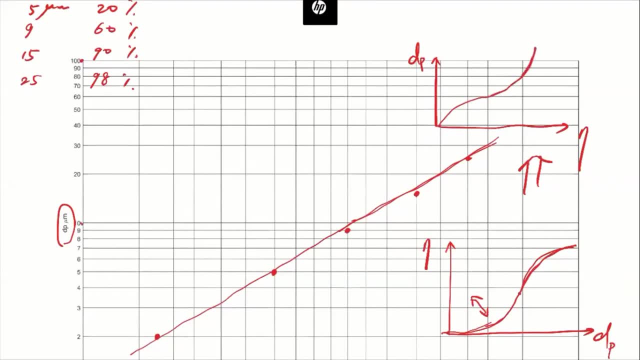 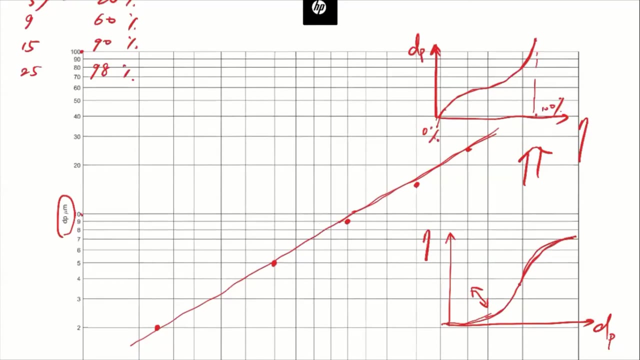 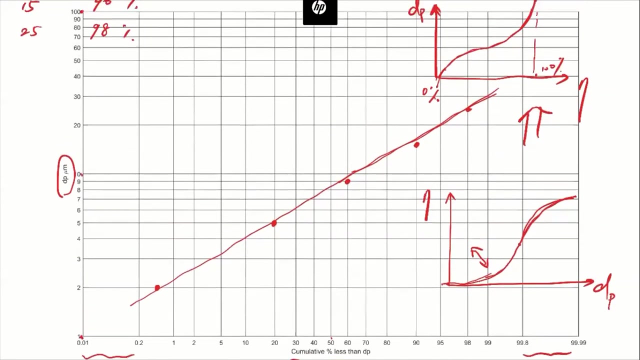 It's going to be Something that looks like this: So we have 100% here right, and then around zero here. OK, So, if you compare. so this is when the cumulative mass fraction is in the linear scale. So now you see what this plot does. is it basically stretch out the region here and here? OK. 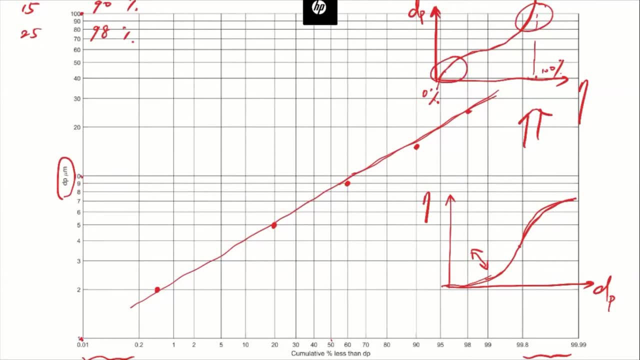 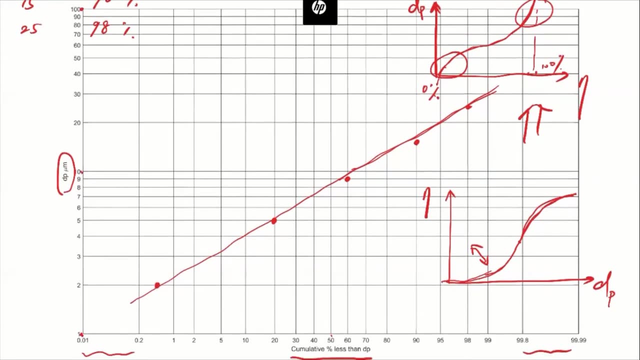 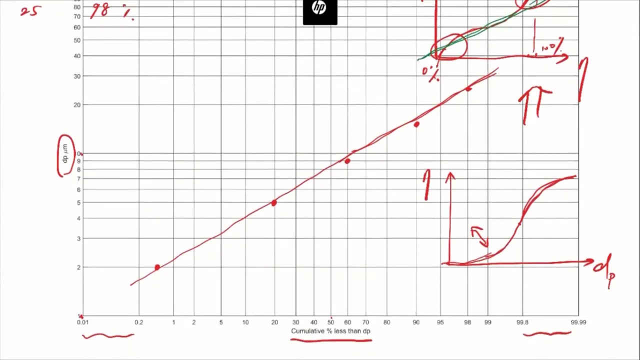 It stretches the fraction when it's getting close to 100%. It also stretches the fraction when it's getting close to 0%. So by stretching that we can get a linear plot. OK, So this is what this engineering plot did, right. 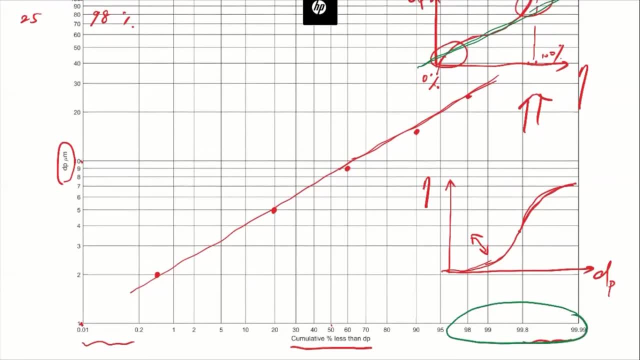 So we stretch out the region where the fraction is OK. So this is what this engineering plot did, right? So we stretch out the region where the fraction is the largest and also stretch out the region where it's the smallest. So that's why we get this plot here. 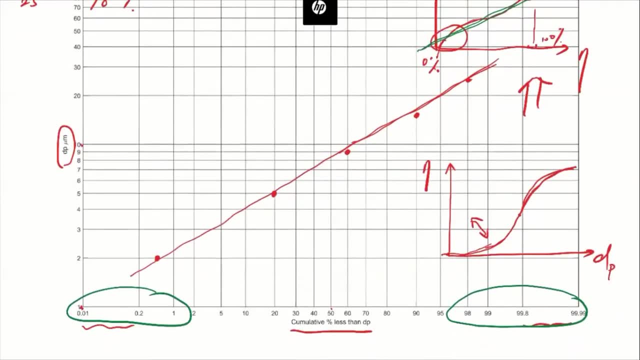 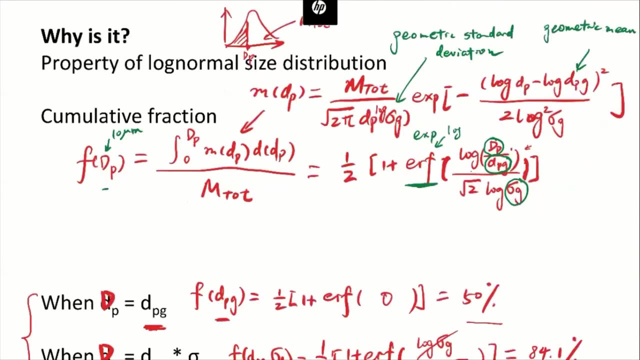 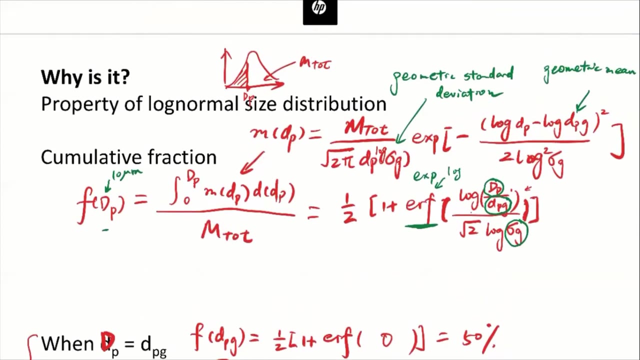 So, if you're interested, actually this stretching has to follow the error function that we discussed earlier. OK, So I have a few backup slides at the end of this class note. If you're interested in that you can see actually how they generate this plot and actually 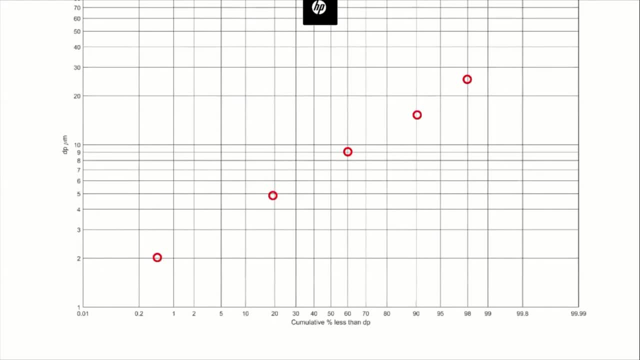 applies for all different types of log normal distributions. OK, So if you're interested in that, you can see actually how they generate this plot and actually applies for all different types of log normal distributions. For example, if a log normal distribution looks like this: right, 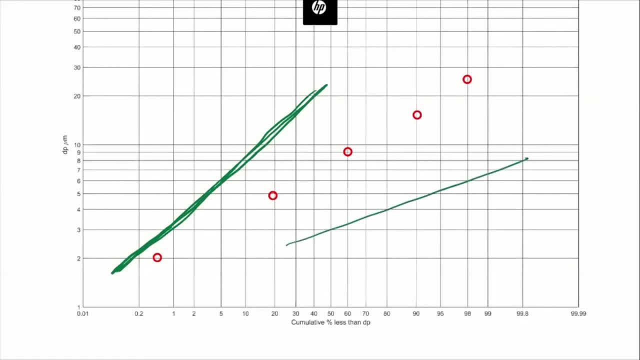 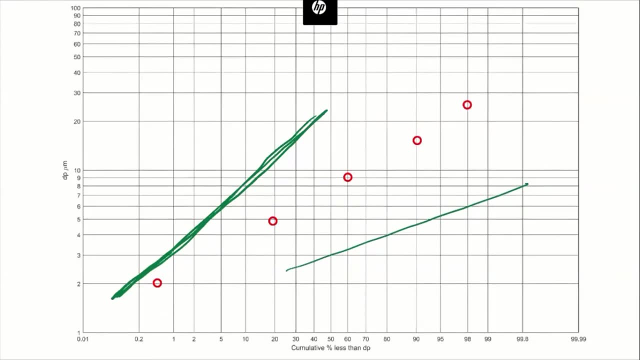 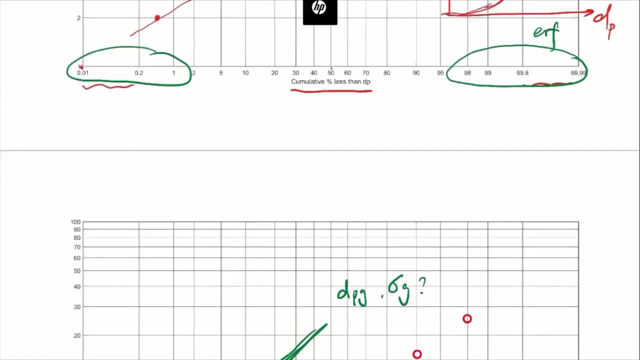 If a distribution looks like this, it's also a log normal. If it looks like this, it's also a log normal distribution. So it's the parameters we discussed. What are the DPG or what are the sigma G? OK, So now let's get back to this problem here. 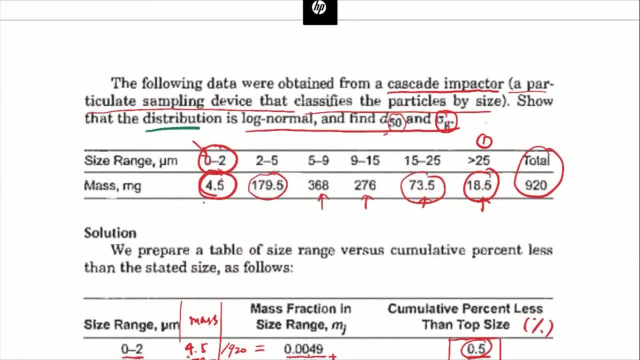 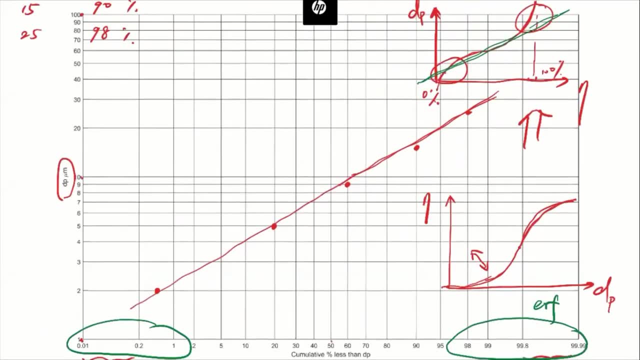 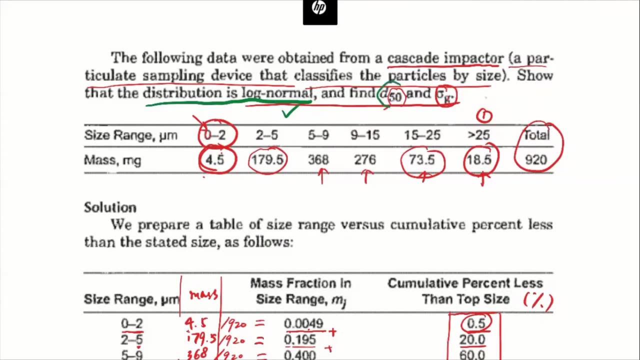 So it wants us to first confirm: OK, The size distribution is log normal. We have done that Right. It is linear, It shows a straight line in this semi-log plot. So that's why it is log normal. But it also wants us to find D50, which is the size that has 50% of the cumulative mass. 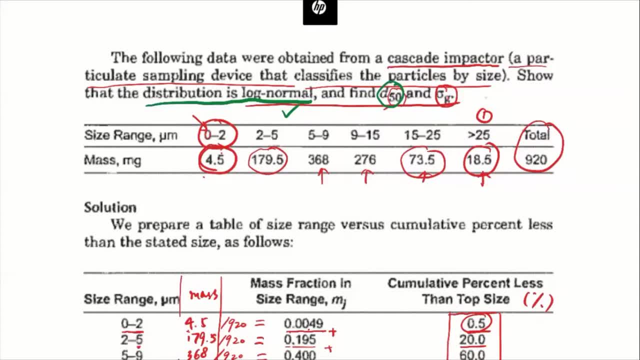 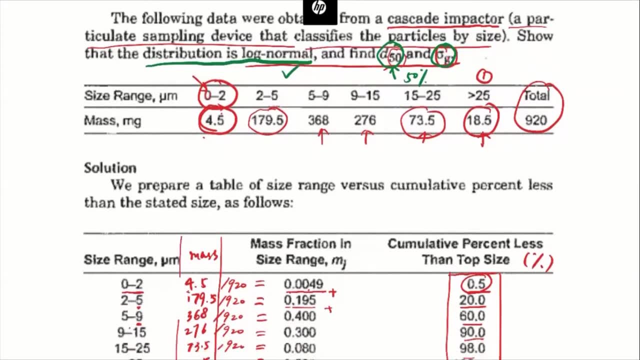 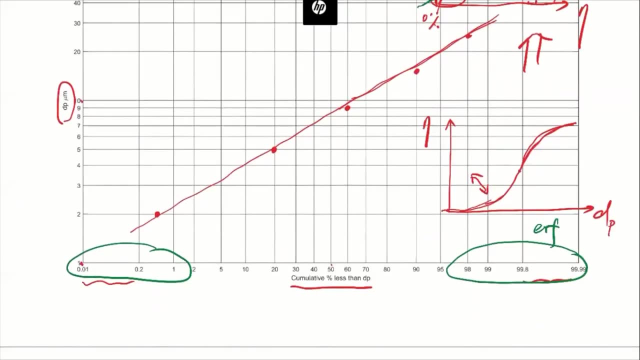 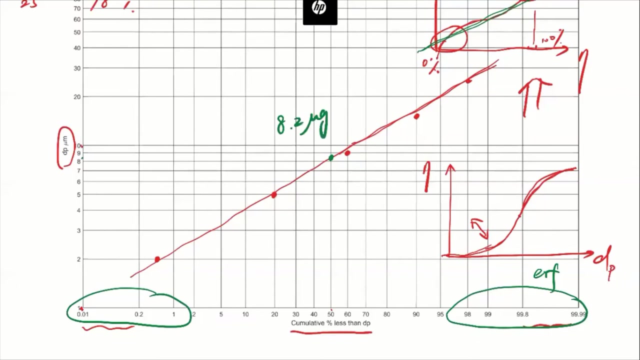 fraction, OK, And also sigma G. So now, if we want to look for this point, 50%, right, It should just be the point that has 50% of the cumulative mass fraction and we can trace that. That's somewhere around, let's say, 8.2 micrometer. 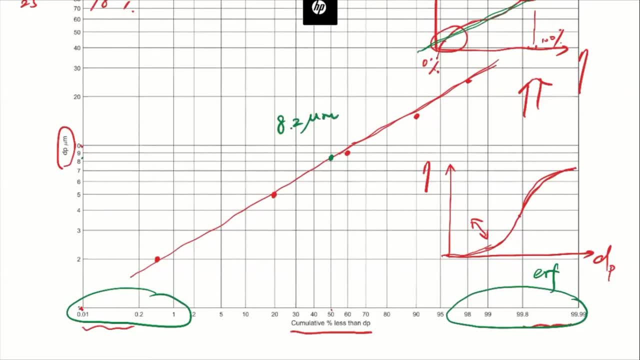 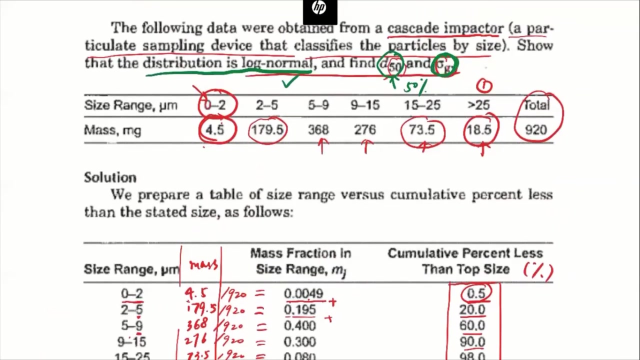 OK, So this is D50.. OK, and this is also dpg, right? we mentioned when the particle size is equal to geometric mean, then the mass fraction, cumulative mass fraction, is 50 percent, right? so now we just need to solve for sigma g. so how do we do that? 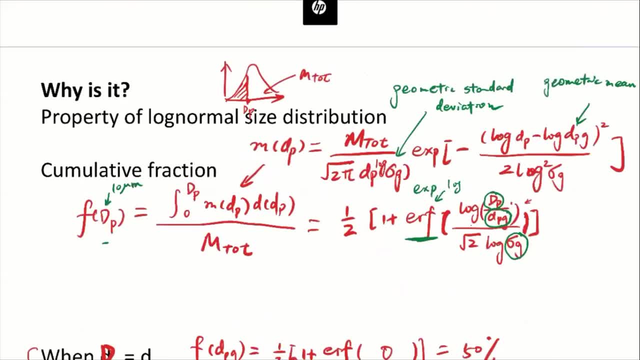 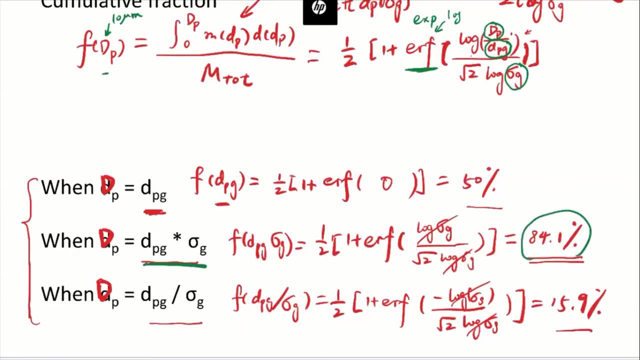 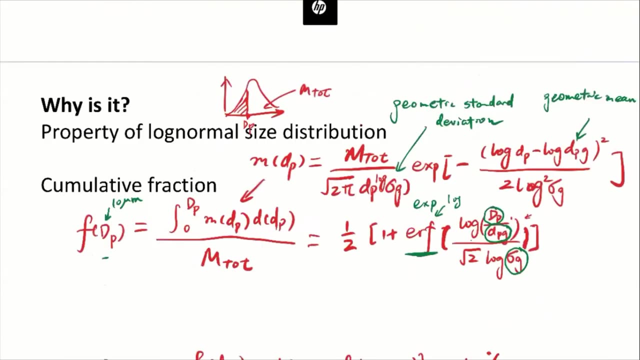 so, if you recall, here we introduced that when particle size is equal to dpg multiplied by sigma g, we have 84.1. when particle size is equal to dpg divided by sigma g, we have 15.9. right, we can just look at these two data points. 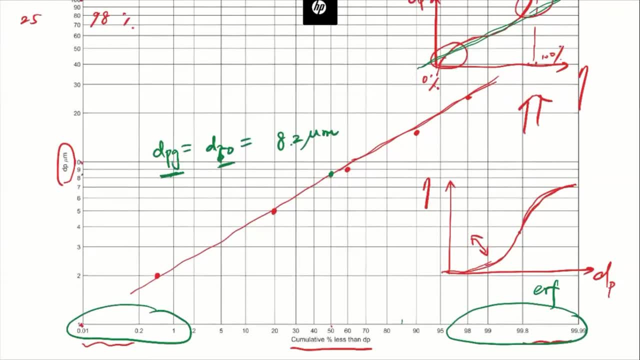 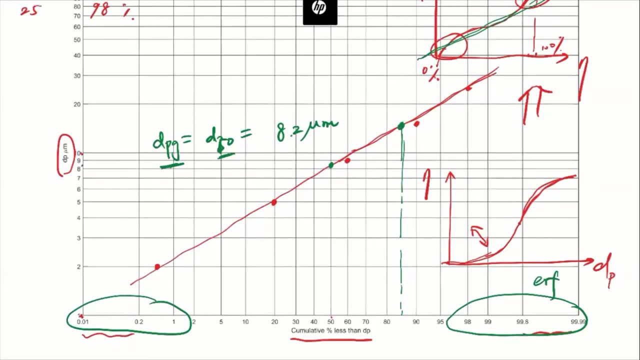 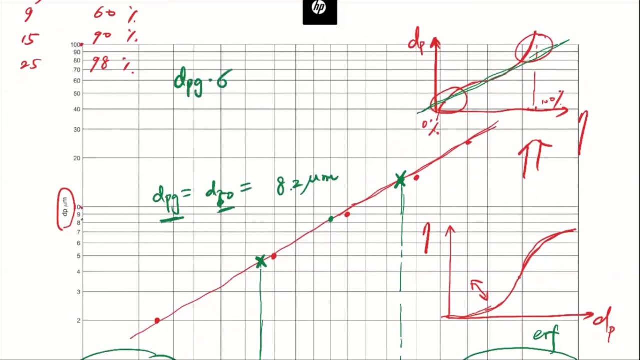 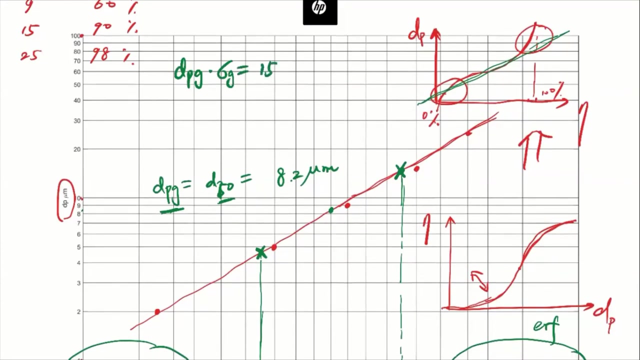 so when at 84.1, that's somewhere here, right, and at 14.9, somewhere here, okay. so now we know that dpg multiplied by sigma g is equal to, let's say, this is 15, okay, and then dpg divided by sigma g is going to be equal to. 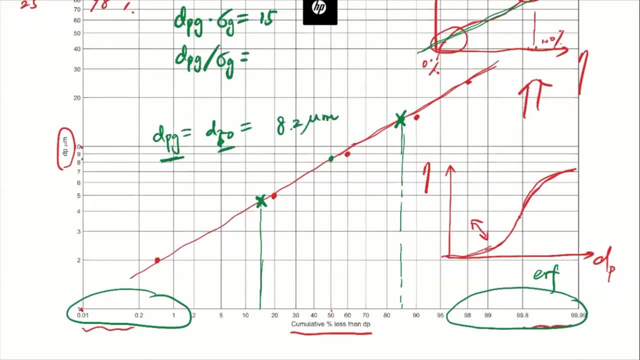 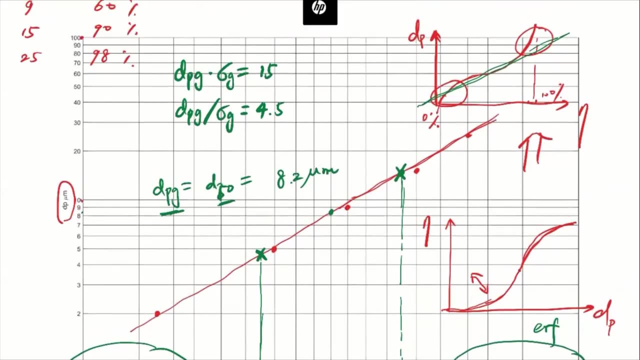 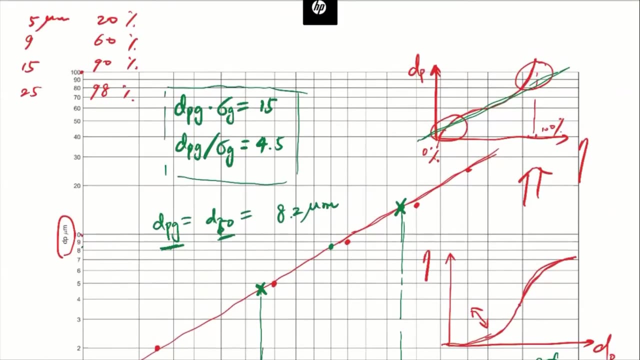 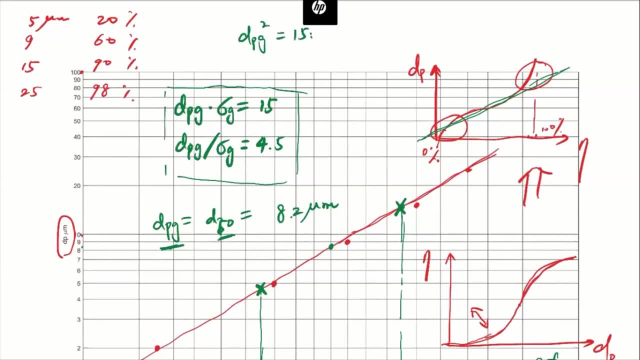 and then we can again solve for dpg. if we multiply these two equations together, so dpg together, so dpg together, so dpg square is going to be equal to 15 multiplied square is going to be equal to 15 multiplied square is going to be equal to 15 multiplied by 4.5. 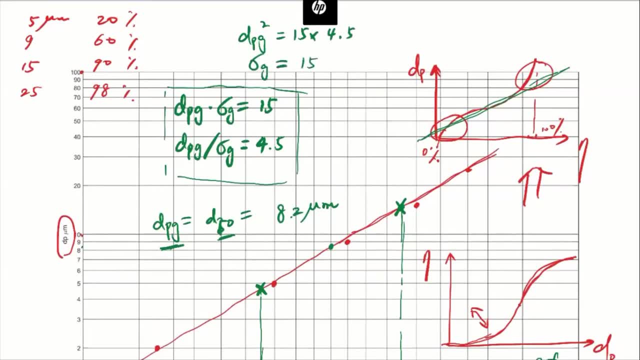 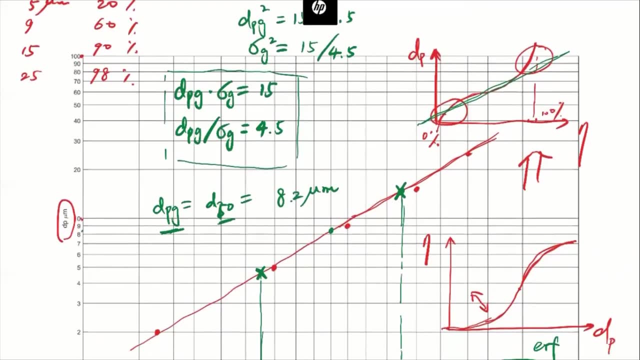 by 4.5, by 4.5, and sigma g is just these two equations and sigma g is just these two equations and sigma g is just these two equations dividing each other: 15 divided by 4.5. okay, so by using this plot, we can: 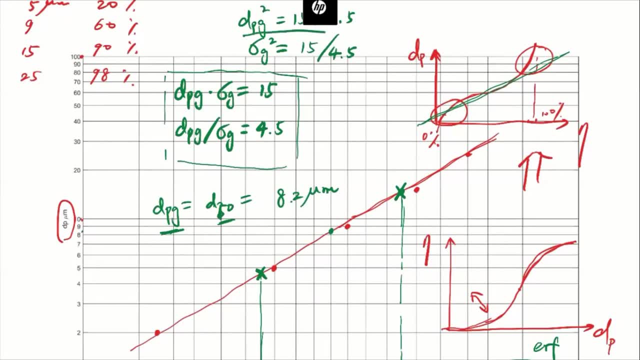 okay, so by using this plot, we can. okay, so by using this plot, we can solve for these parameters. so you may solve for these parameters. so you may solve for these parameters. so you may wonder: does this number match with this? wonder: does this number match with this? 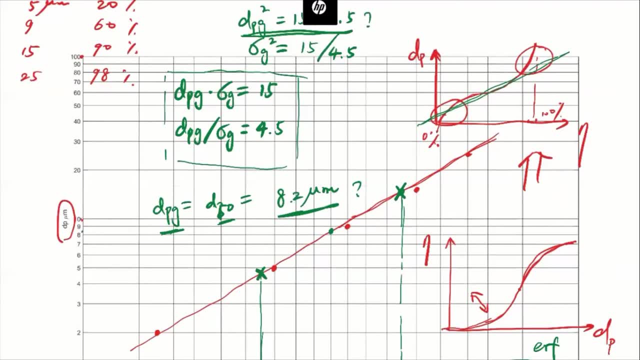 wonder: does this number match with this number, number, number? so we have to do the calculation. so if so, we have to do the calculation. so if so, we have to do the calculation. so if they, theoretically they should be exactly they, theoretically they should be exactly they, theoretically they should be exactly the same. but normally, 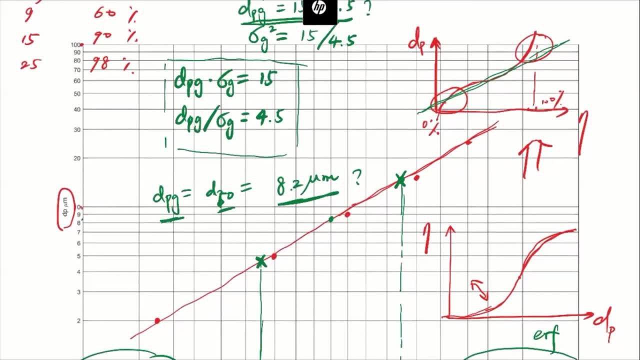 the same, but normally the same. but normally, when we use this plot to identify the, when we use this plot to identify the, when we use this plot to identify the data points, they may differ by a little data points. they may differ by a little data points. they may differ by a little bit. so we can just. 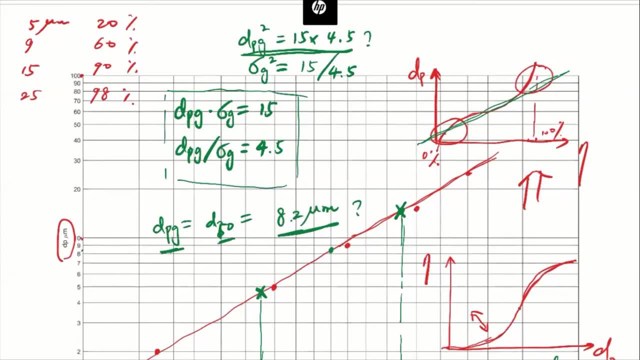 bit, so we can just bit, so we can just calculate in this way, and then take the calculate in this way, and then take the calculate in this way and then take the average. okay, so that's going to be more average. okay, so that's going to be more. 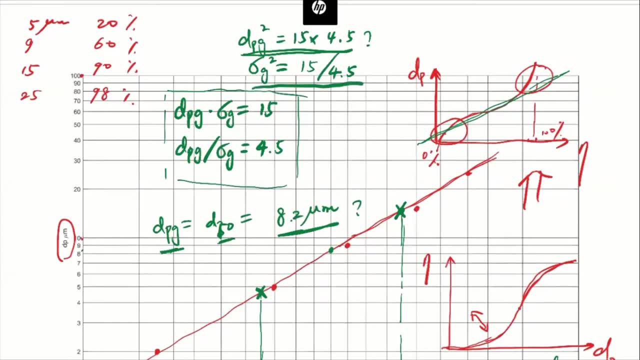 average. okay, so that's going to be more accurate. accurate. accurate, but based on this equation, we can. but based on this equation, we can. but based on this equation, we can. calculate what is the sigma g, calculate what is the sigma g. calculate what is the sigma g. so this is all by just using this. 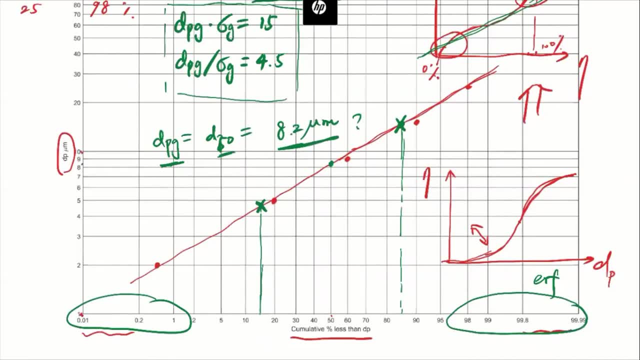 so this is all by just using this. so this is all by just using this simple semi-log plot. we simple semi-log plot, we simple semi-log plot, we basically, we can get a lot of, basically, we can get a lot of, basically, we can get a lot of information out of it. 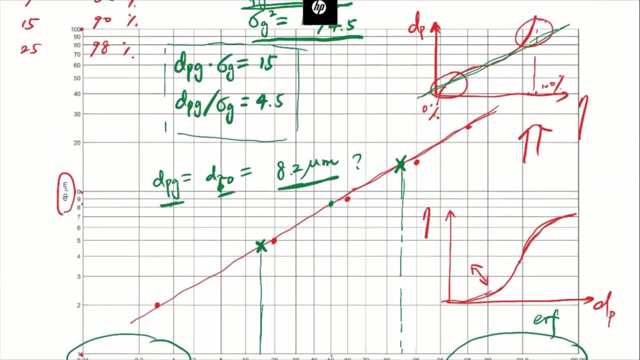 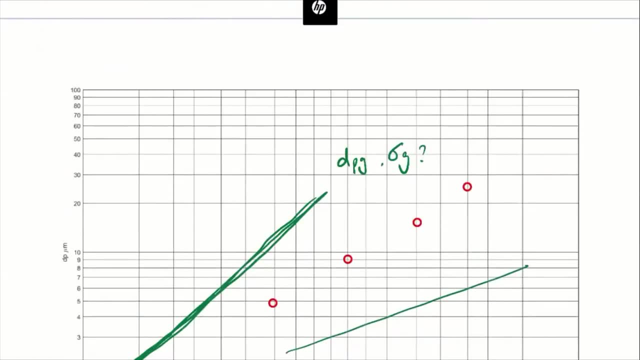 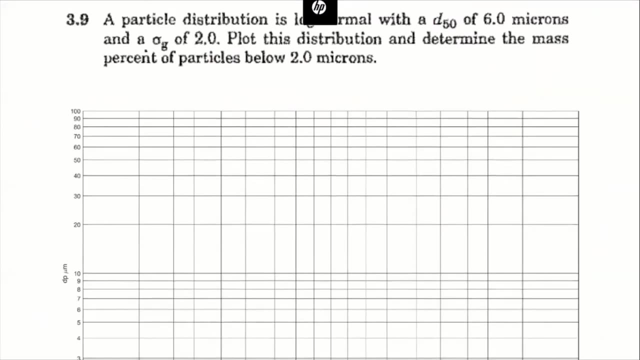 information out of it. information out of it, all right, all right, all right. so any questions until now. so any questions until now. so any questions until now. good, good, good, okay, nice, okay, nice, okay, nice, um, um, um, so let's do another practice, all right. so let's say we have a. 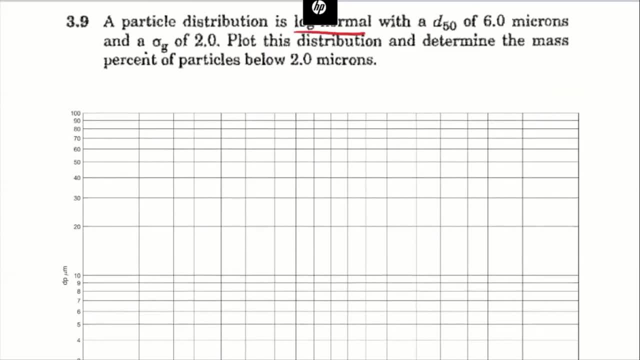 all right. so let's say we have a. all right, so let's say we have a particle size distribution that is log particle size distribution. that is log particle size distribution. that is log, normal, normal, normal. so it has a d50 or the dpg of save the. 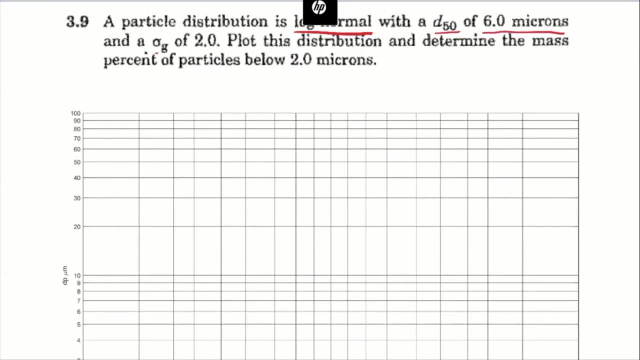 so it has a d50 or the dpg of save the. so it has a d50 or the dpg of save the six microns. six microns, six microns, okay, and a sigma sigma g of two. okay, and a sigma sigma g of two. 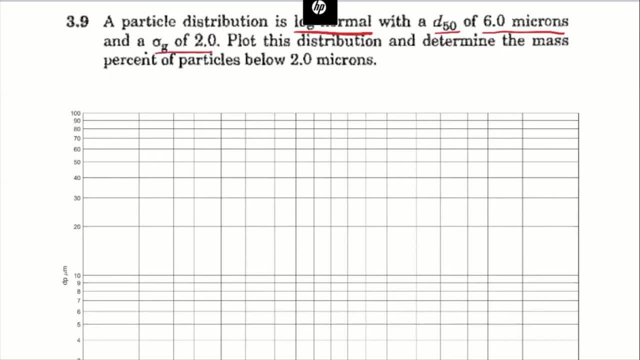 okay, and a sigma, sigma g, of two. so this time we know that this is a. so this time we know that this is a. so this time we know that this is a log- normal size distribution log- normal size distribution log- normal size distribution. okay, so it wants us to plot the. 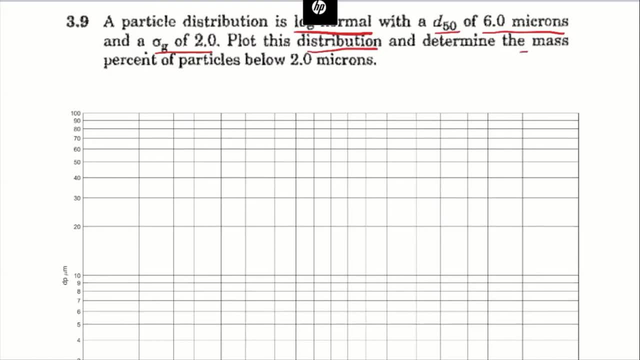 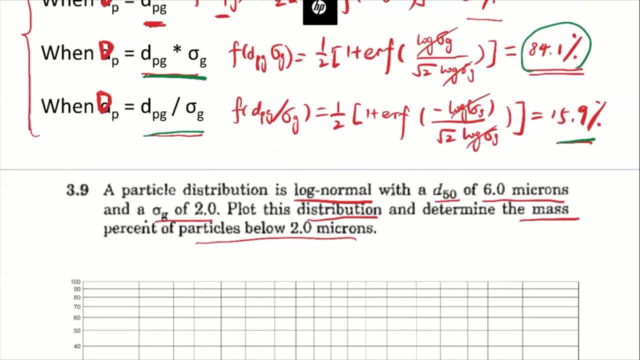 okay, so it wants us to plot the. okay, so it wants us to plot the distribution. okay, so it wants us to plot the distribution, distribution, distribution. so if we don't have this, so if we don't have this, so if we don't have this semi-log plot, so the typical way is: 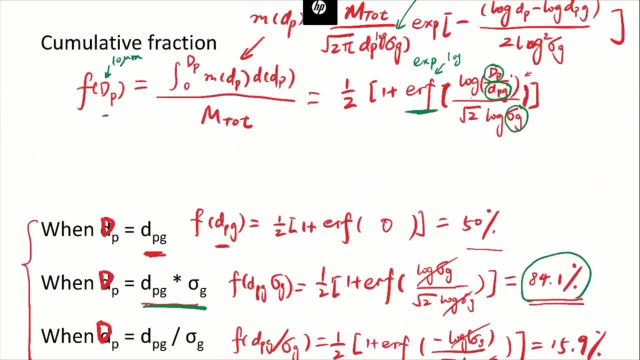 semi-log plot. so the typical way is semi-log plot. so the typical way is: we'll just plug in these six and two, we'll just plug in these six and two, we'll just plug in these six and two into this equation, into this equation, into this equation, into the size distribution. let's say and: 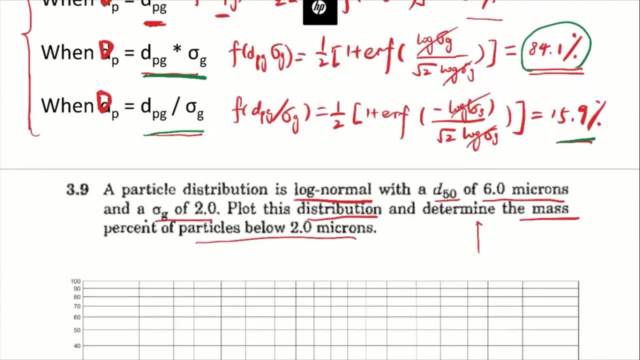 into the size distribution, let's say, and into the size distribution, let's say, and then make the plot. but that's going to then make the plot, but that's going to then make the plot. but that's going to be very complicated. be very complicated, be very complicated. the semi-log plot help us solve quite 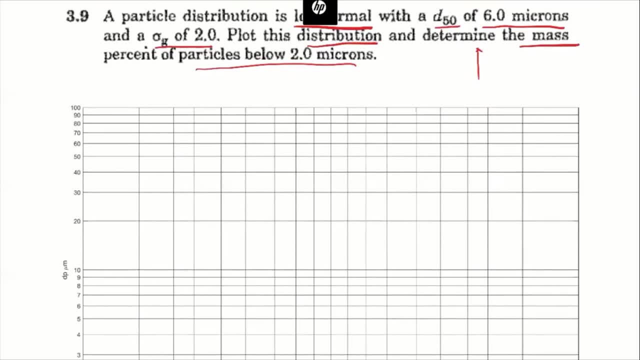 the semi-log plot. help us solve quite the semi-log plot. help us solve quite many things, okay. so the way we do that many things, okay, so the way we do that many things, okay, so the way we do that is first. so d50 is six microns, so let's. 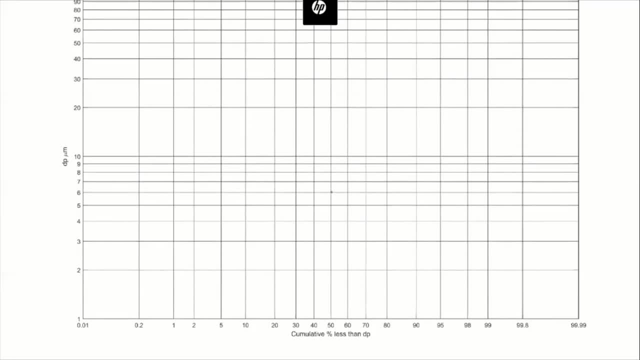 is first. so d50 is six microns, so let's is first. so d50 is six microns. so let's just look at six, just look at six, just look at six. okay, so that's going to be this point. okay, so that's going to be this point. 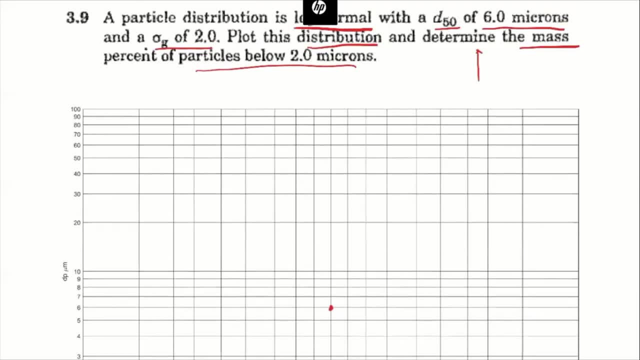 okay, so that's going to be this point right, and we have d50 right, and we have d50 right and we have d50 and also sigma g. so we know that when dp and also sigma g. so we know that when dp and also sigma g, so we know that when dp is equal to. 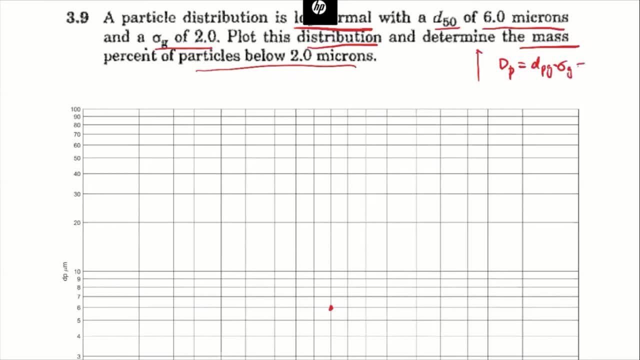 is equal to: is equal to: dpg multiplied by sigma g. dpg multiplied by sigma g. dpg multiplied by sigma g, which is 12, which is 12, which is 12, the cumulative fraction is 84.1. the cumulative fraction is 84.1. 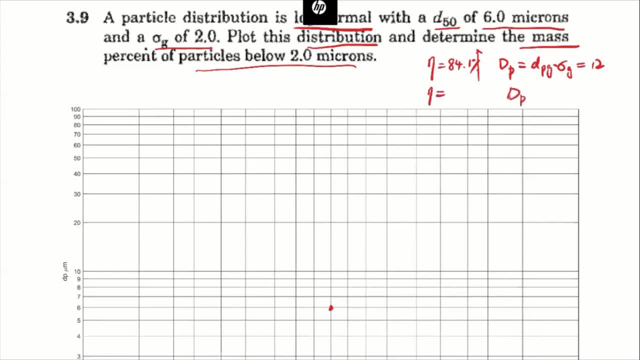 the cumulative fraction is 84.1. okay, okay, okay, when, when, when, when dpg. when dp is equal to dpg. when dpg. when dp is equal to dpg. when dpg. when dp is equal to dpg, divided by sigma g. divided by sigma g. 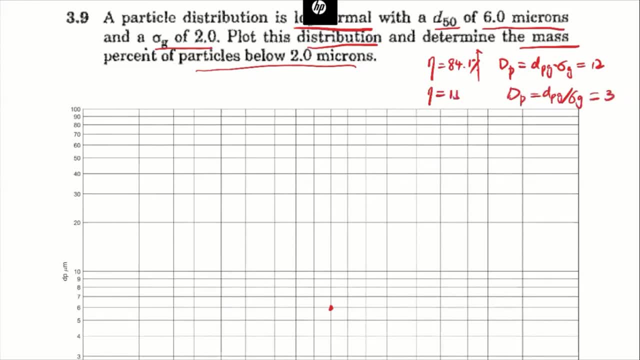 divided by sigma g, which is three, which is three, which is three, the cumulative fraction should be 15.9. the cumulative fraction should be 15.9. the cumulative fraction should be 15.9, percent, percent, percent. so the way we do that is: let's look for. 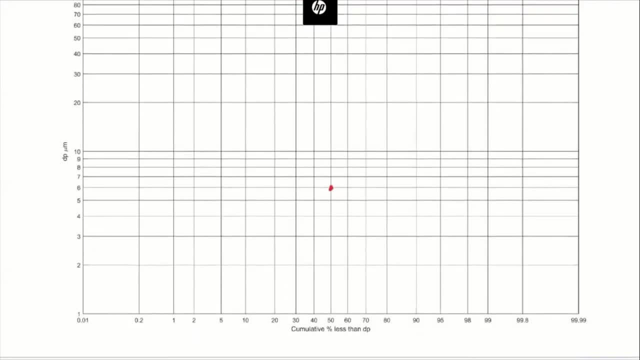 so the way we do that is: let's look for. so the way we do that is: let's look for 12, 12, 12, 12. is somewhere here? okay, let's look for. is somewhere here? okay, let's look for. is somewhere here? okay, let's look for the three first. 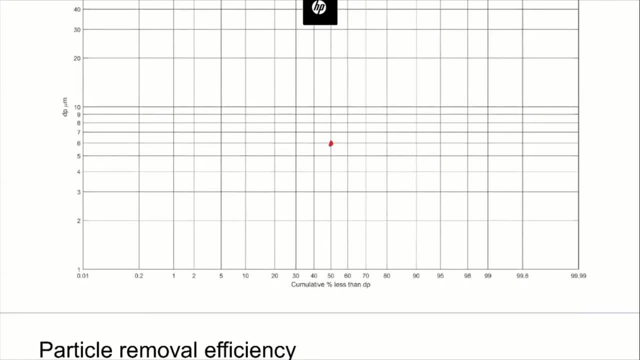 the three first, the three first. three is somewhere here, right, and we'll three is somewhere here, right, and we'll three is somewhere here, right, and we'll look for, look for, look for 14.9, which is somewhere here. 14.9, which is somewhere here. 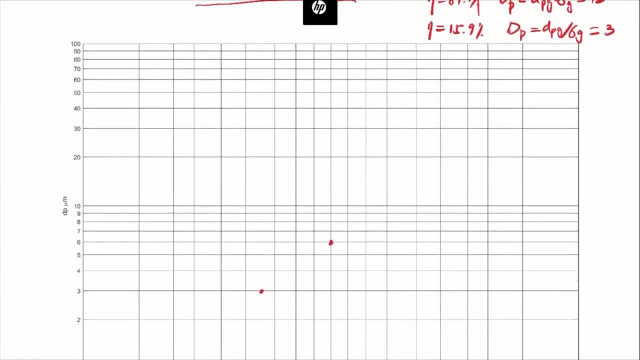 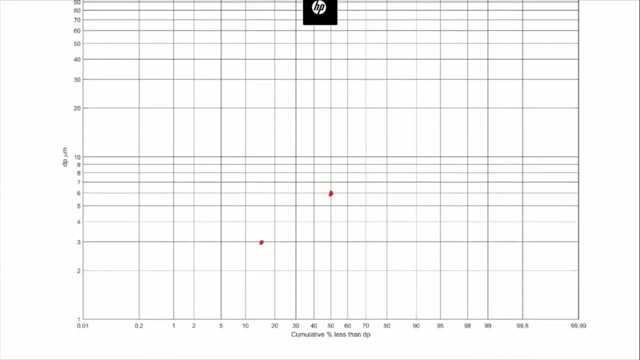 14.9, which is somewhere here, and then, and then, and then. for the dpg equal to 12, for the dpg equal to 12, for the dpg equal to 12, that's equal to, that's equal to, that's equal to 84.1. 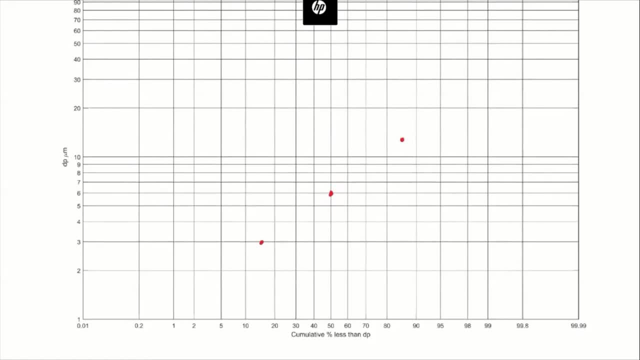 84.1, 84.1. it should be somewhere here. it should be somewhere here, it should be somewhere here. okay, so then we can just draw a straight line. so then we can just draw a straight line. so then we can just draw a straight line, because we already know. 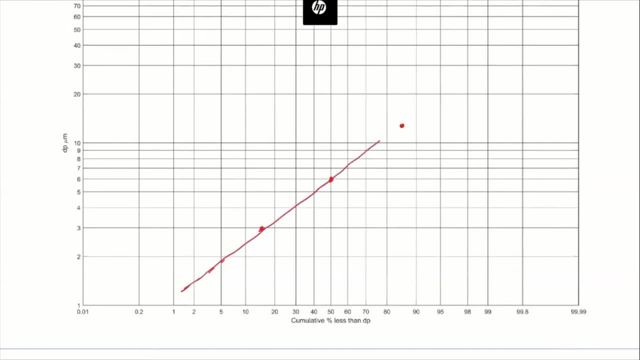 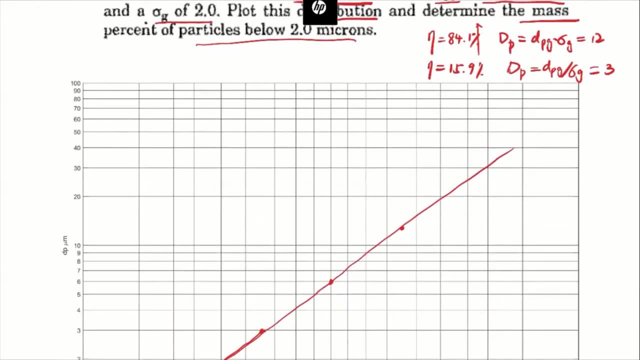 because we already know, because we already know that it is a log normal size, that it is a log normal size, that it is a log normal size distribution. okay, so now, how do we determine the mass? okay, so now, how do we determine the mass? okay, so now, how do we determine the mass percent of particles below two microns? 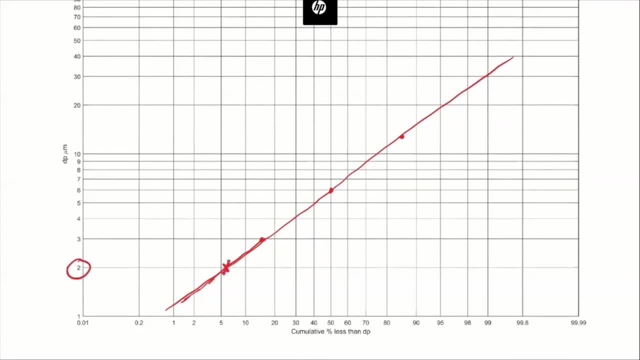 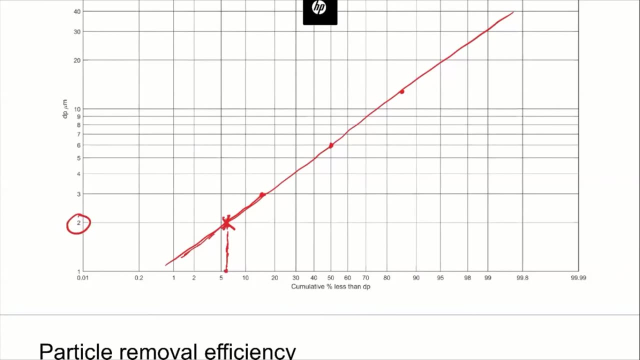 we'll just use this line, right. we'll just use this line, right. we'll just use this line right. this is two microns, this is two microns, this is two microns. look for here vertical line, vertical line, vertical line. right, that's somewhere around. right, that's somewhere around. 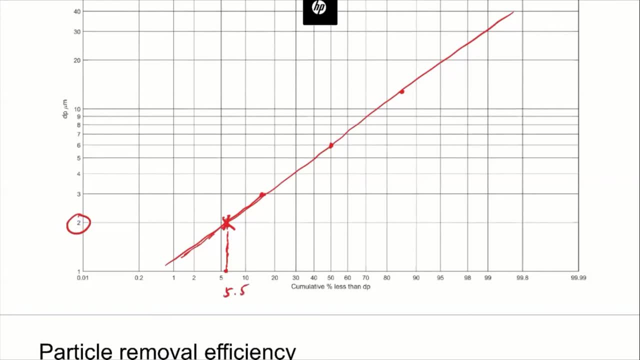 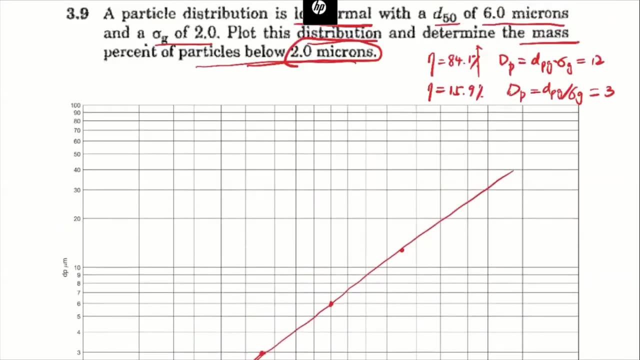 right, that's somewhere around uh uh, uh. this, this is probably around 5.5 percent. this is probably around 5.5 percent. this is probably around 5.5 percent, okay, so so, so, by using this plot, it really simplifies. by using this plot, it really simplifies. 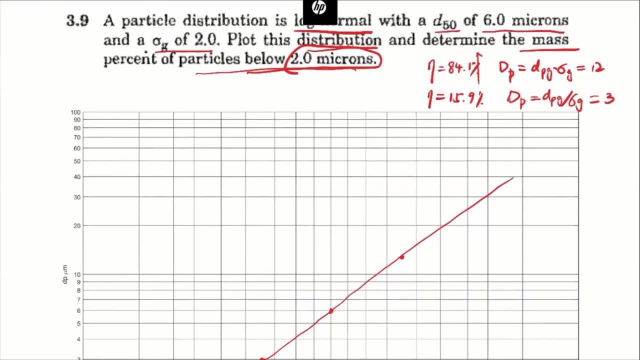 by using this plot, it really simplifies a lot of things, a lot of things, a lot of things. right, so we don't need to go through those right. so we don't need to go through those right, so we don't need to go through those very complex calculations. just. 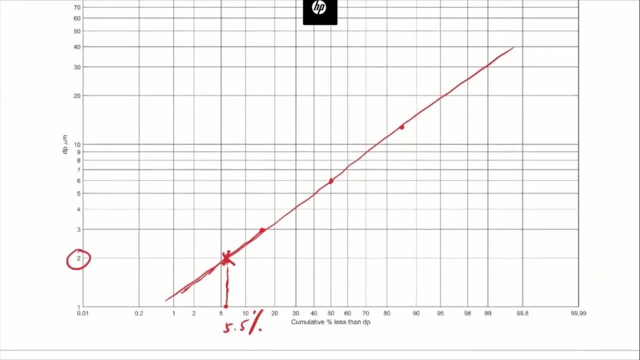 very complex calculations, just very complex calculations. just need to make a few data points, and then need to make a few data points, and then need to make a few data points, and then we can easily do, we can easily do, we can easily do easily calculate the mass fractions for. 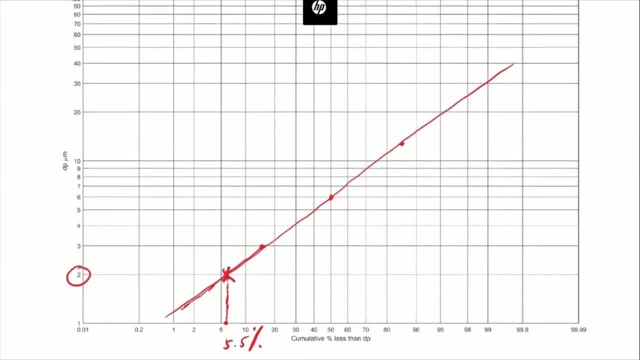 easily calculate the mass fractions. for easily calculate the mass fractions, for example, example, example. let's say, now we're interested in the. let's say now we're interested in the. let's say now we're interested in the cumulative fraction below four microns, all right, below four microns. 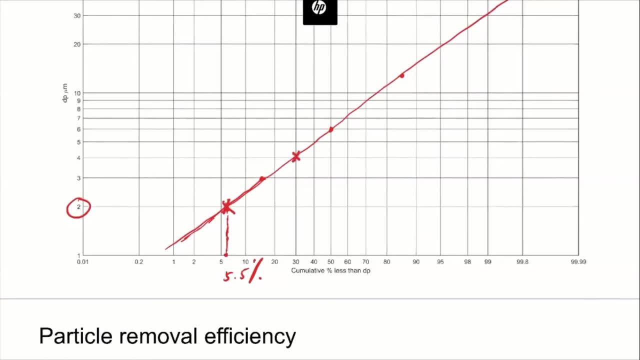 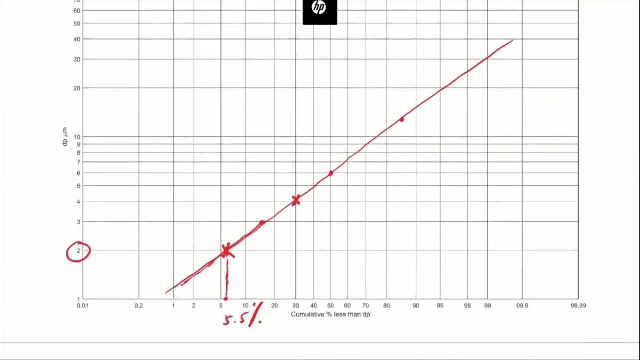 all right below four microns. all right below four microns. again. look for the again. look for the again. look for the data point here, data point here, data point here. right, that's around 30 percent, right, right, right. so i hope this is clear enough um. 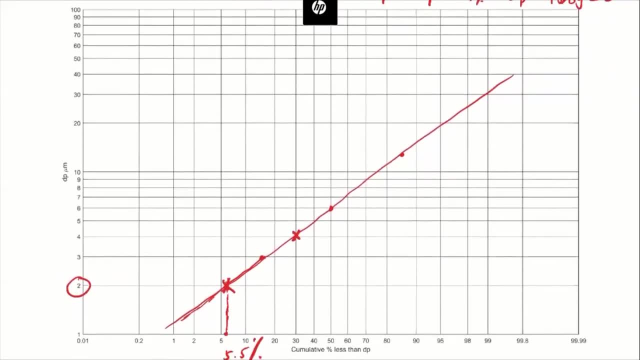 so i hope this is clear enough. um, so i hope this is clear enough. um, you also get a few practices in your. you also get a few practices in your. you also get a few practices in your homework problems. okay, so let's try to. homework problems- okay, so let's try to. 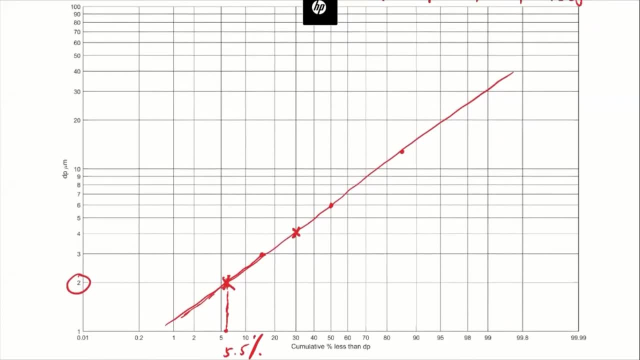 homework problems. okay, so let's try to get familiarized with this. get familiarized with this. get familiarized with this semi-log plot. it's going to be very semi-log plot. it's going to be very semi-log plot. it's going to be very helpful. 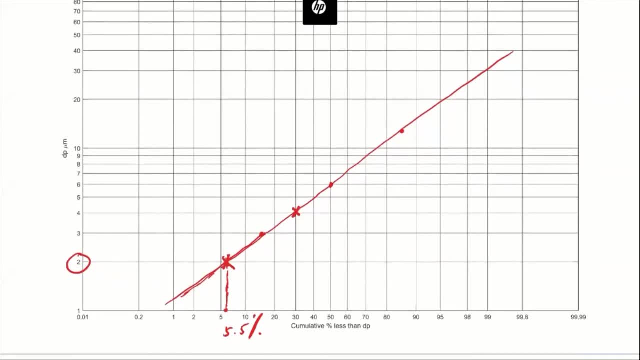 helpful. helpful when we try to look for the size. when we try to look for the size, when we try to look for the size, distributions- but let me know if you have distributions. but let me know if you have distributions. but let me know if you have any questions or if you are not clear on 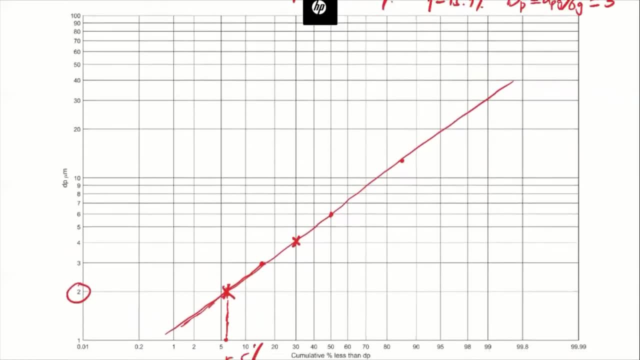 any questions, or if you are not clear on any questions, or if you are not clear on anything, anything, anything, all right, um so, all right, um so, all right, um. so, at the end of this class, um, i think, at the end of this class, um, i think. 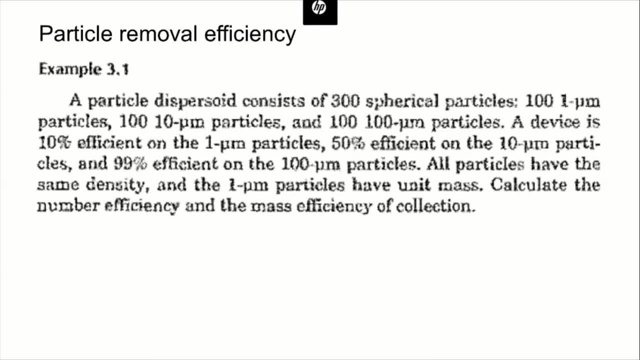 at the end of this class. um, i think, basically i also want to go through the. basically, i also want to go through the. basically, i also want to go through the calculation of the particle removal. calculation of the particle removal, calculation of the particle removal or, or or the gas pollutant control. right, let's. 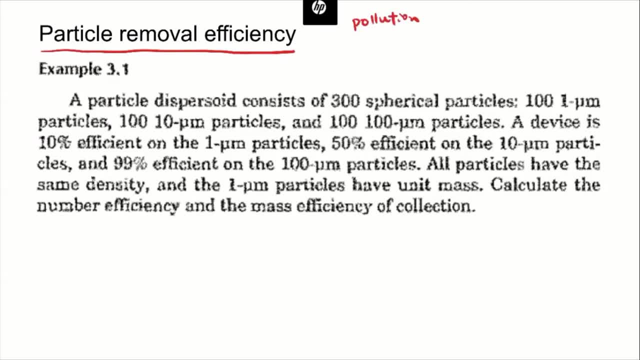 the gas pollutant control. right, let's the gas pollutant control, right, let's say the pollution control, pollution control methods. okay, so people will always discuss. okay, so people will always discuss. okay, so people will always discuss something, something, something. for example, the removal efficiency, or for example, the removal efficiency, or 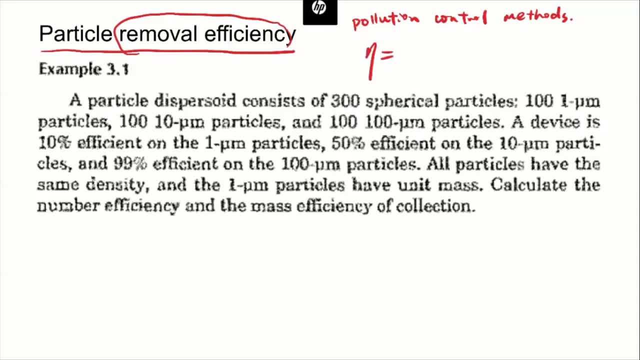 for example, the removal efficiency or control efficiency, control efficiency, control efficiency. so this efficiency, so this efficiency, so this efficiency just means, just means, just means the parts or the, the parts or the, the parts or the, let's say the quantity, let's say the quantity, let's say the quantity removed. 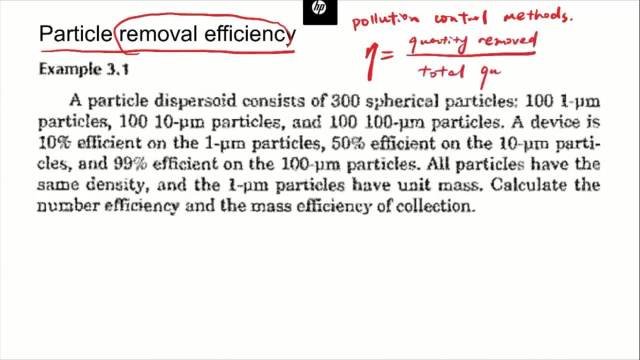 divide by the total quantity. okay, so this is how we calculate the okay. so, this is how we calculate the okay. so this is how we calculate the removal efficiency. removal efficiency, removal efficiency. so if the removal efficiency is 100, so if the removal efficiency is 100, 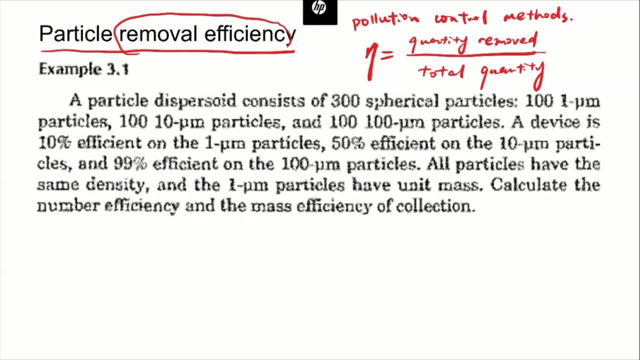 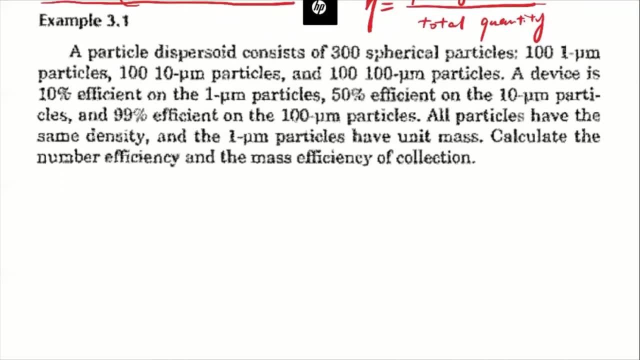 so if the removal efficiency is 100, then the quantity to remove is going to, then the quantity to remove is going to, then the quantity to remove is going to be equal to the, be equal to the, be equal to the total quantity right. total quantity right. total quantity right. so let's say we have this example here. 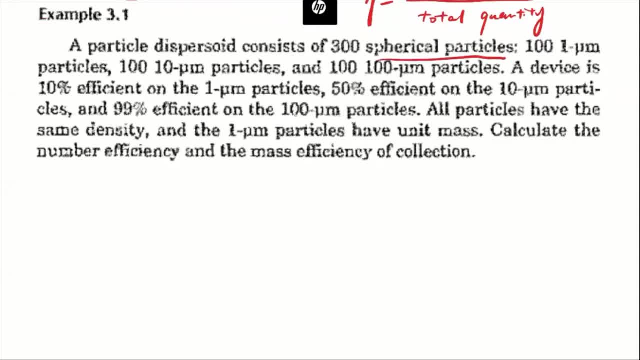 let's say we have 300. let's say we have 300. let's say we have 300 spherical particles. but these 300 spherical particles, but these 300 spherical particles, but these 300 particles have different sizes. particles have different sizes, particles have different sizes. so 100 of them. 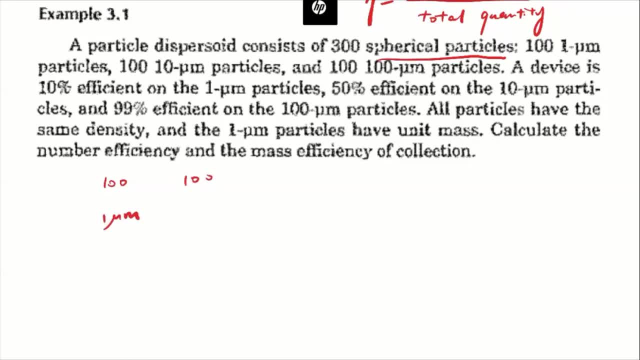 so 100 of them. so 100 of them are one microns are one microns are one microns. 100 of them are 10 microns, 100 of them are 10 microns, 100 of them are 10 microns and 100 of them are 100 microns. 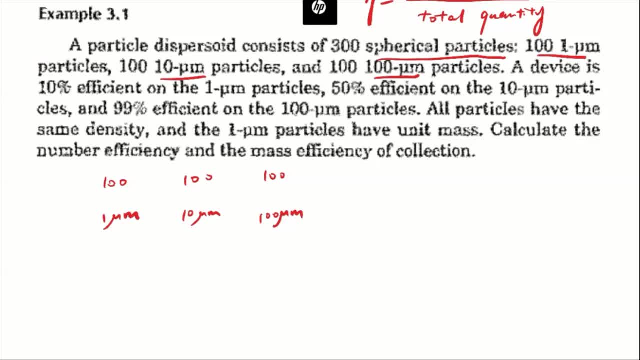 and 100 of them are 100 microns. and 100 of them are 100 microns. okay, so they have different sizes. okay, so they have different sizes. okay, so they have different sizes. so let's say we have a device, we have a. so let's say we have a device, we have a. 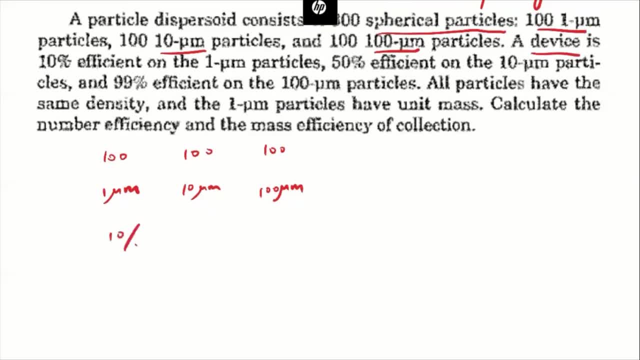 so let's say we have a device, we have a control device that is 10 percent control device. that is 10 percent control device. that is 10 percent efficient for the one micron particles. efficient for the one micron particles. efficient for the one micron particles: 50 percent. 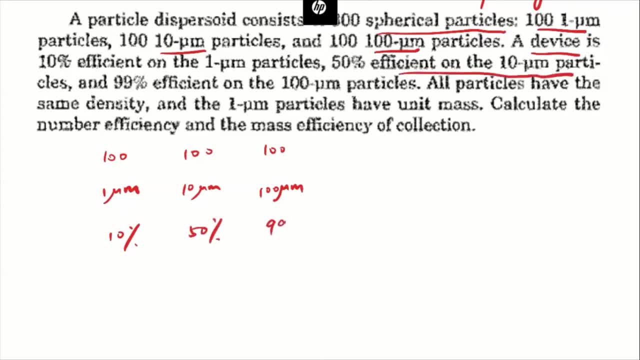 50 percent. 50 percent efficient for the 10 microns and 99 efficient for the 10 microns and 99 efficient for the 10 microns and 99 efficient for the 100 micron particles. efficient for the 100 micron particles. efficient for the 100 micron particles. actually, this is a typical situation for 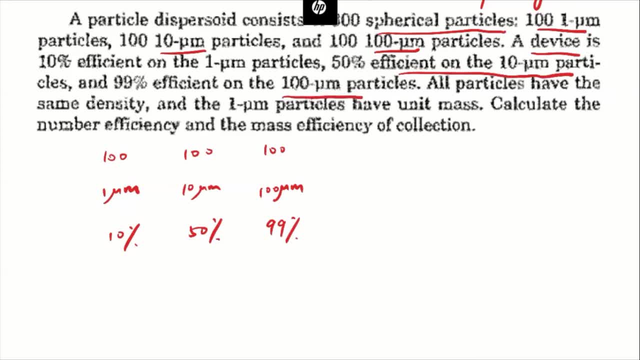 actually this is a typical situation, for actually this is a typical situation for a lot of particle removal device, a lot of particle removal device, a lot of particle removal device. they're very efficient for removing very. they're very efficient for removing very. they're very efficient for removing very large particles. 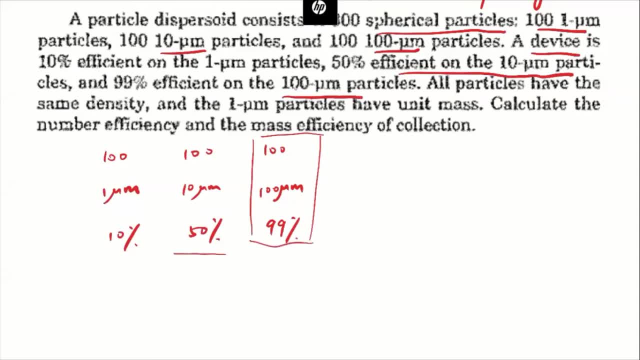 large particles, large particles, but they're less efficient when we talk. but they're less efficient when we talk. but they're less efficient when we talk about smaller particles. this is also the about smaller particles. this is also the about smaller particles. this is also the reason why. 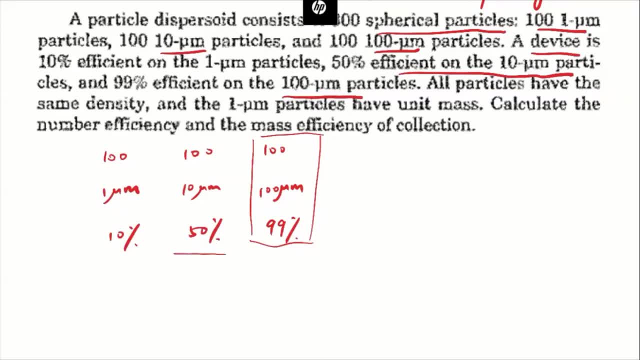 reason why? reason why we have a lot of pm 2.5 right pm 10. we have a lot of pm 2.5 right pm 10. we have a lot of pm 2.5 right pm 10, pm 2.5 mainly because these control. 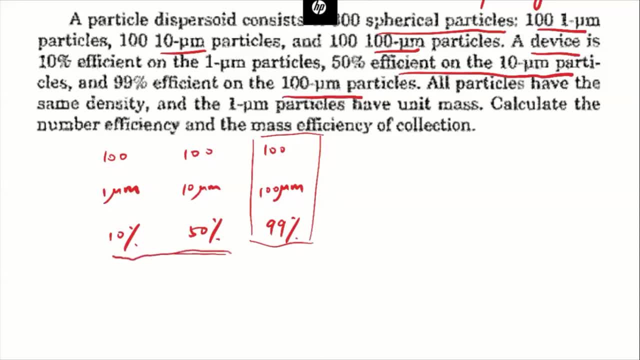 pm 2.5. mainly because these control pm 2.5, mainly because these control devices. they're not efficient devices. they're not efficient devices. they're not efficient when they're removing these smaller, when they're removing these smaller, when they're removing these smaller particles. 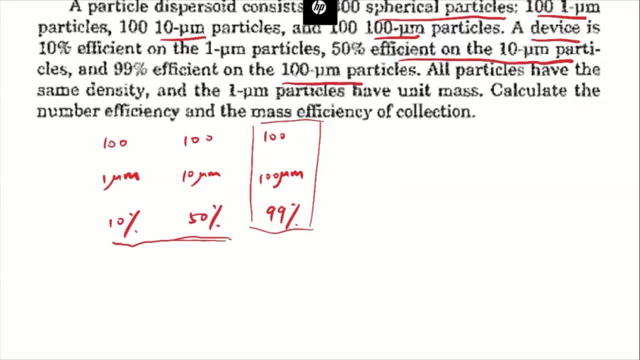 particles, particles, okay, so let's further assume that all okay. so let's further assume that all okay. so let's further assume that all the particles have the same density. the particles have the same density, the particles have the same density and the one micron particles have the 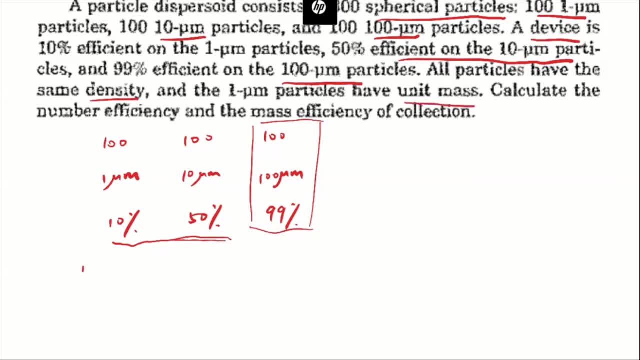 and the one micron particles have the and the one micron particles have the unit mass, unit mass, unit mass. this is just meaning that the density is. this is just meaning that the density is. this is just meaning that the density is one is equal to the density of water. 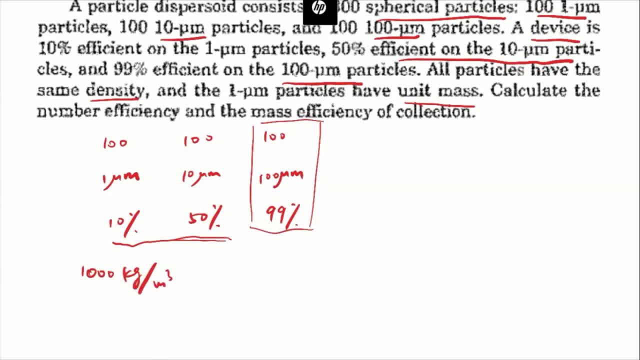 one is equal to the density of water. one is equal to the density of water, which is one thousand kilogram per meter, which is one thousand kilogram per meter, which is one thousand kilogram per meter. cube, cube, cube. so it wants us to calculate what is. 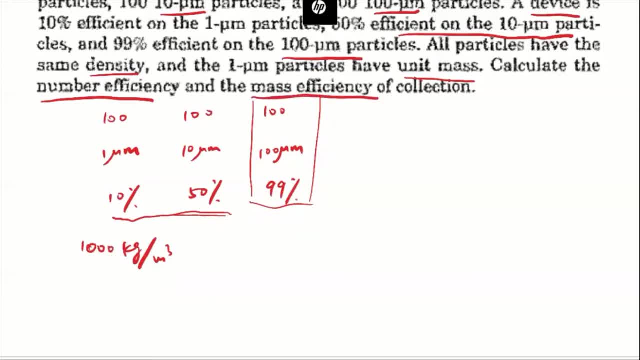 so it wants us to calculate what is so it wants us to calculate what is: number efficiency, number efficiency, number efficiency and the mass removal efficiency for the. and the mass removal efficiency for the. and the mass removal efficiency for the device, device, device. okay, so, okay, so, okay, so people will also use these different. 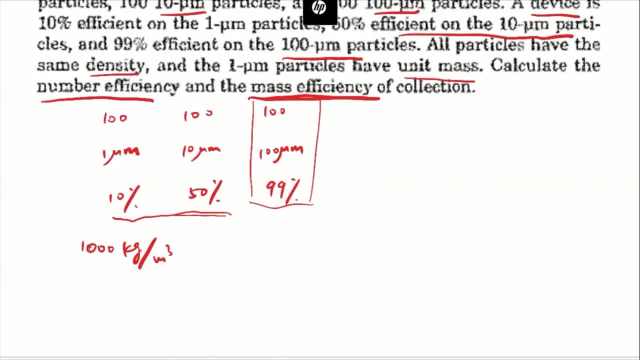 people will also use these different people will also use these different values of efficiencies. so, right now, values of efficiencies. so, right now, values of efficiencies. so right now, let's say for power plants when they're- let's say for power plants when they're, let's say for power plants when they're removing pm. they're mainly referring to 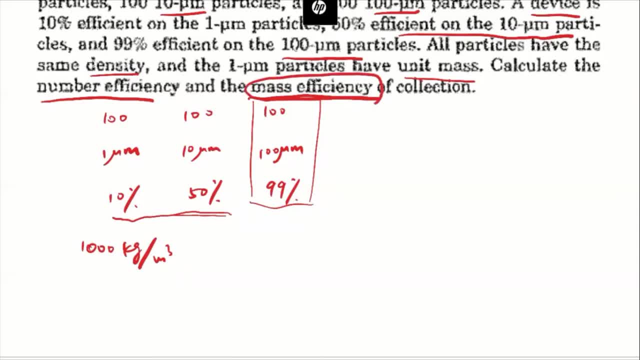 removing pm. they're mainly referring to removing pm. they're mainly referring to the mass efficiency, the mass efficiency, the mass efficiency. okay, so we'll find out actually how. okay, so, we'll find out actually how. okay, so we'll find out actually how that's different in terms of different. 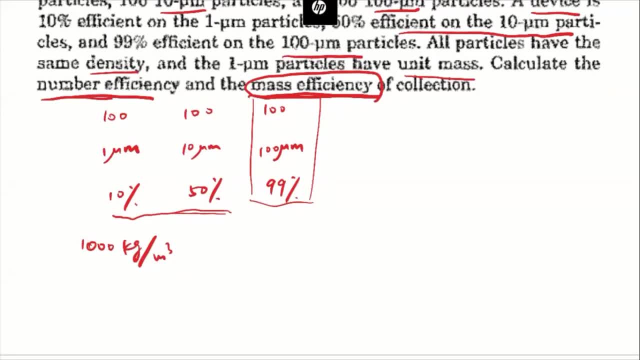 that's different in terms of different, that's different in terms of different quantities: quantities, quantities. let's say regarding the number, let's say regarding the number, let's say regarding the number: efficiency, we know that efficiency, we know that efficiency, we know that. so we know the total quantity is 300. 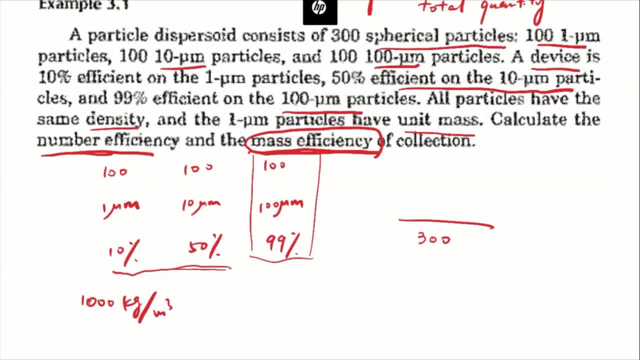 so we know the total quantity is 300. so we know the total quantity is 300. okay, by using this equation 300. okay, by using this equation 300. okay, by using this equation 300. so the quantity removed for the one, so the quantity removed for the one. 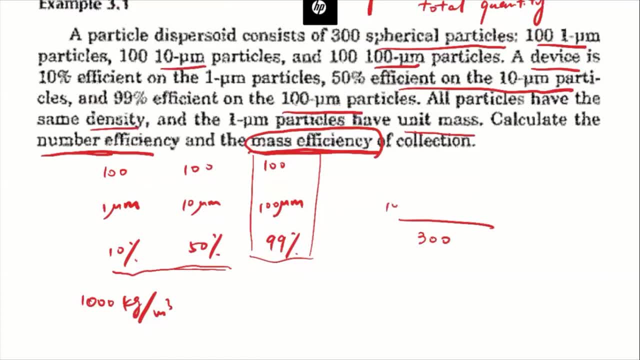 so the quantity removed for the one micrometer particle, so that's 10 micrometer particle, so that's 10 micrometer particle, so that's 10, which is 10 particle right for the 100, which is 10 particle right for the 100. 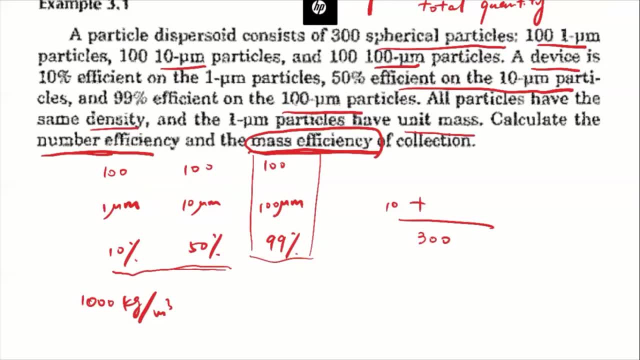 which is 10 particle right for the 100 particle, one hand for the 10 micrometer particle, one hand for the 10 micrometer particle, one hand for the 10 micrometer. particle 50 is removed. particle 50 is removed. particle 50 is removed, so this should be 30, not 10. okay. 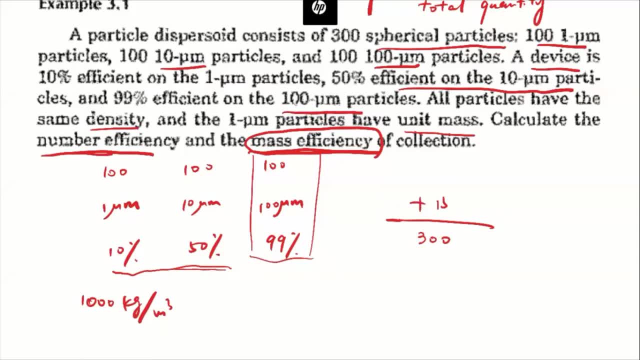 so this should be 30, not 10. okay, so this should be 30, not 10, okay. 30 and this is uh no, it should be 10.. 30 and this is uh no, it should be 10.. 30 and this is uh no, it should be 10.. so we're just talking about this: 100. 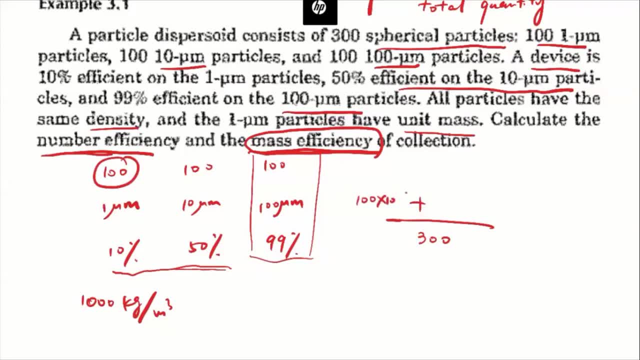 so we're just talking about this 100. so we're just talking about this 100 micron particles, right? so that's going, micron particles, right. so that's going, micron particles, right. so that's going to be 100 multiplied by 10, to be 100 multiplied by 10. 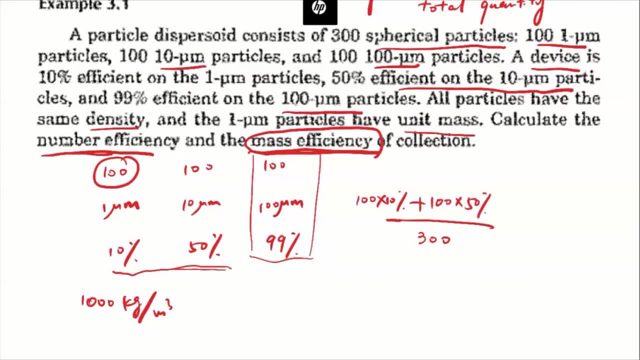 to be 100 multiplied by 10, 100 multiplied by 50, 100 multiplied by 50, 100 multiplied by 50 and 100 multiplied by 99, and 100 multiplied by 99 and 100 multiplied by 99. okay, so this is the number removal. 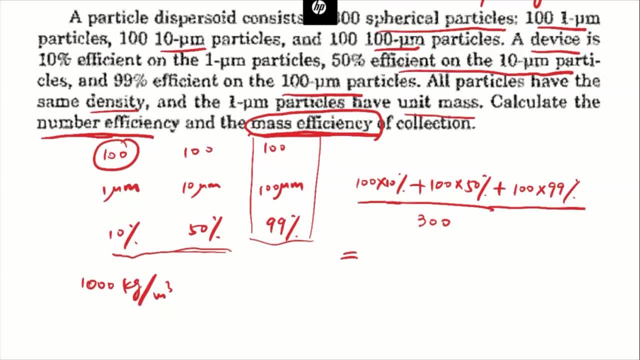 okay, so this is the number removal. okay, so this is the number removal efficiency, right? so if you do the calculation, i right. so if you do the calculation, i right. so if you do the calculation, i think i have the answer here. think i have the answer here. 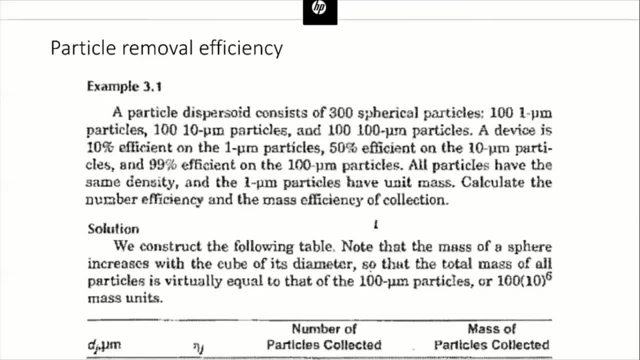 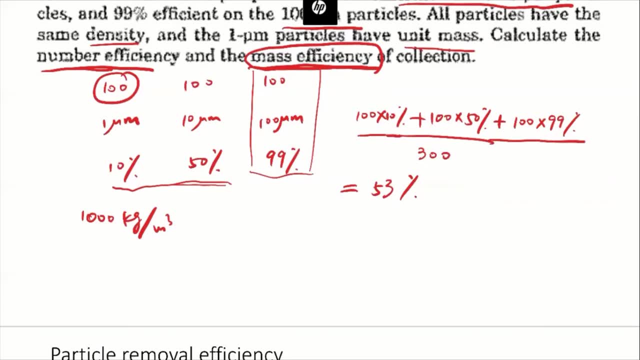 think i have the answer here. do the calculation that's going to be. do the calculation that's going to be. do the calculation that's going to be around 53 percent. okay, okay, okay. so this is the number removal efficiency. so this is the number removal efficiency. 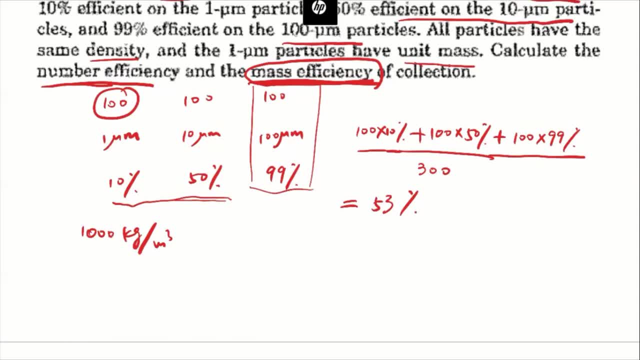 so this is the number: removal efficiency and in terms of mass removal efficiency, and in terms of mass removal efficiency, and in terms of mass removal efficiency, then we need to use a different quantity, then we need to use a different quantity, then we need to use a different quantity, right? so the total quantity 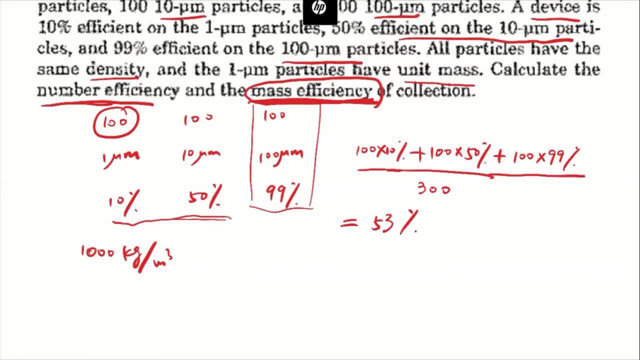 right. so the total quantity: right. so the total quantity is going to be the total mass of all of is going to be the total mass of all of is going to be the total mass of all of these particles, right, these particles right, these particles, right. so let's say this is number efficiency. 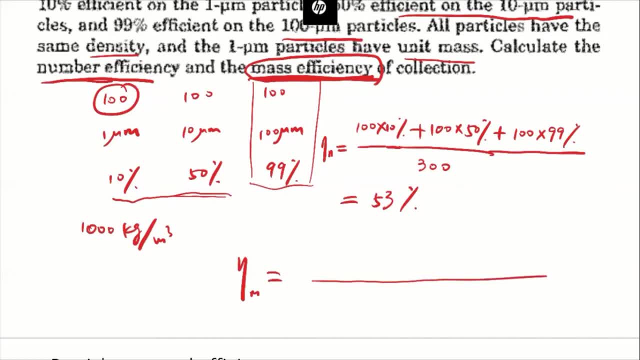 so let's say: this is number efficiency. so let's say this is number efficiency, this is mass efficiency, this is mass efficiency, this is mass efficiency. then this is going to be 100, then this is going to be 100, then this is going to be 100 multiplied by. 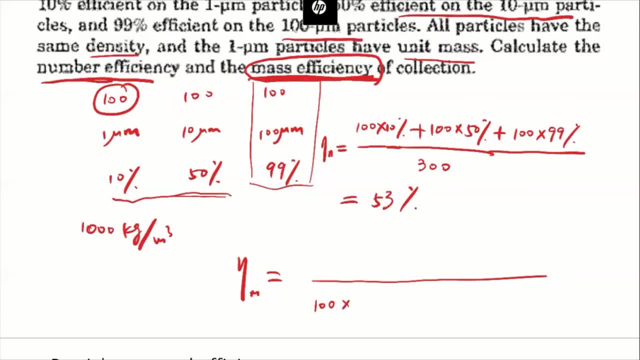 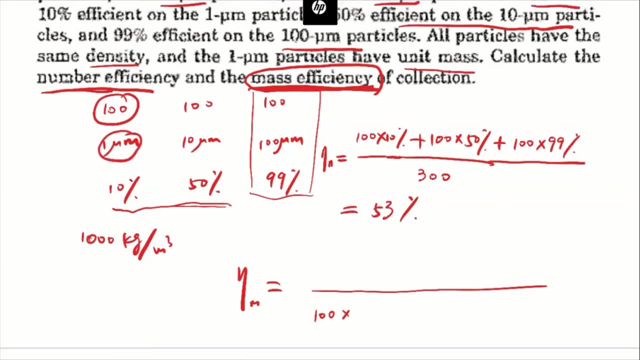 multiplied by, multiplied by. and we know, let's say, and we know, let's say, and we know, let's say: let's assume that, let's assume that the let's assume that, let's assume that the let's assume that let's assume that the one micrometer particle have a mass of 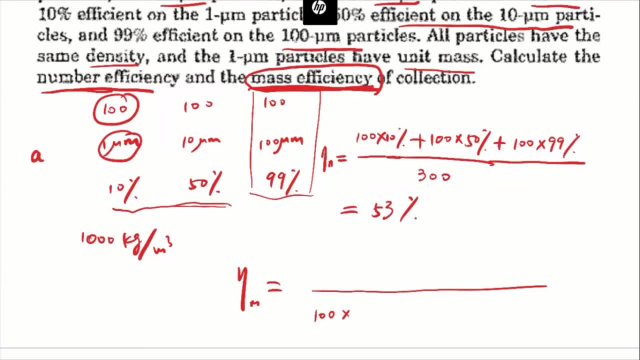 one micrometer particle have a mass of one micrometer particle, have a mass of a right, a right, a right. so we know that the mass scales with. so we know that the mass scales with. so we know that the mass scales with volume and the volume is. 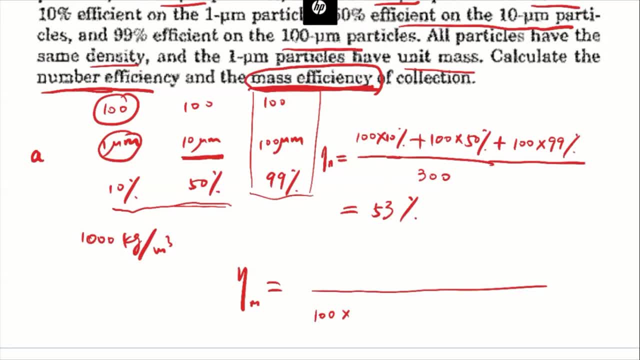 volume and the volume is volume and the volume is the 10 to the third. or added the uh the 10 to the third, or added the uh the 10 to the third, or added the uh, let's say 10 to the third of the, let's say 10 to the third of the. 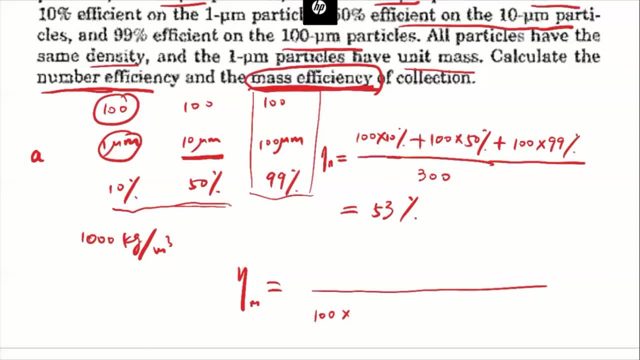 let's say 10 to the third of the diameter right. so basically diameter right, so basically diameter right. so basically, for the 10 micrometer particle, the mass for the 10 micrometer particle, the mass for the 10 micrometer particle, the mass of of. 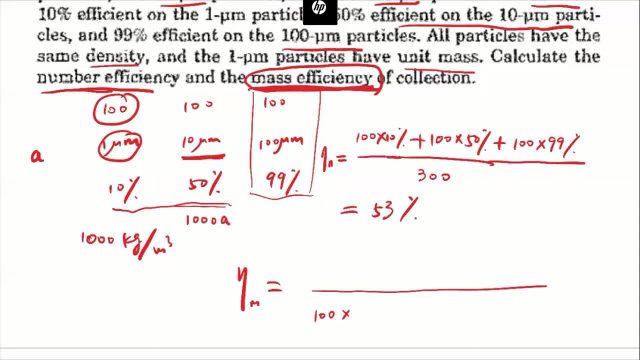 of those particles will be 1000a right. those particles will be 1000a right. those particles will be 1000a right. because, because, because let's say volume is pi over six, let's say volume is pi over six. let's say volume is pi over six. dp to the third. 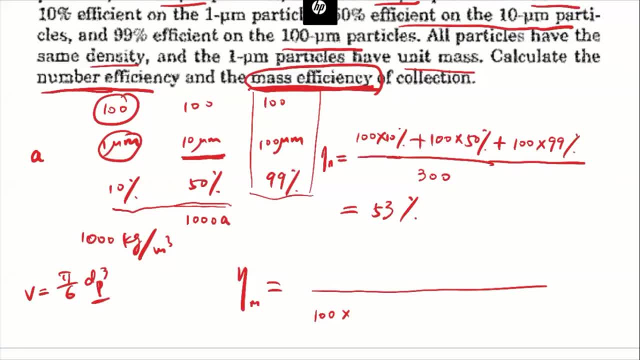 dp to the third. dp to the third. okay, it's, it's a cube of the particle. okay, it's, it's a cube of the particle. okay, it's, it's a cube of the particle. diameter, diameter, diameter. so if the the one micrometer particle, so if the the one micrometer particle, 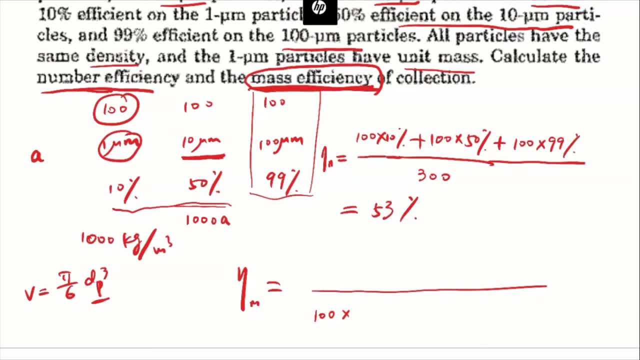 so if the, the one micrometer particle have a, have a, have a mass of a, then 10 micrometer particle, mass of a, then 10 micrometer particle. mass of a, then 10 micrometer particle will have a mass of one thousand, will have a mass of one thousand. 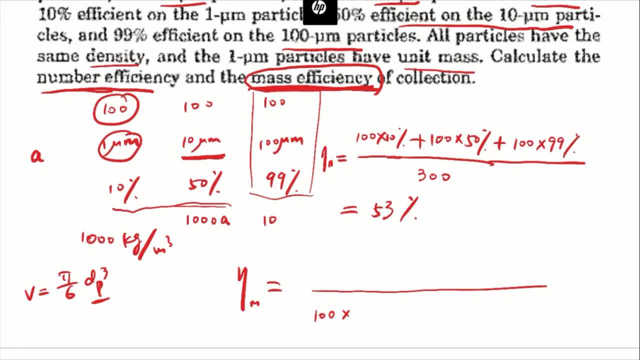 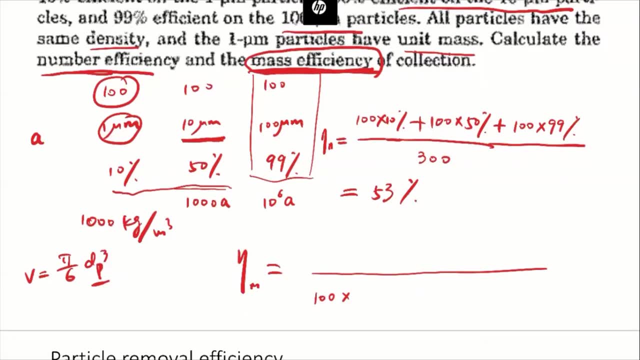 will have a mass of one thousand right, right, right, and then the 100 micrometer particles, and then the 100 micrometer particles, and then the 100 micrometer particles will have, will have, will have a mass of 10 to the sixth of a right, so then, the total quantity being 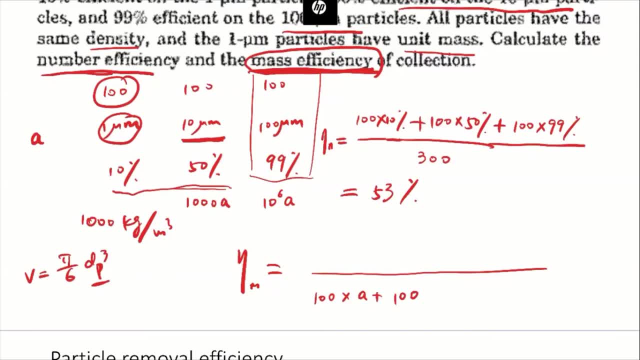 right. so then the total quantity being right, so then the total quantity being removed removed. removed are just 100 multiplied by a. are just 100 multiplied by a. are just 100 multiplied by a. 100 multiplied by 1000 a. 100 multiplied by 1000 a. 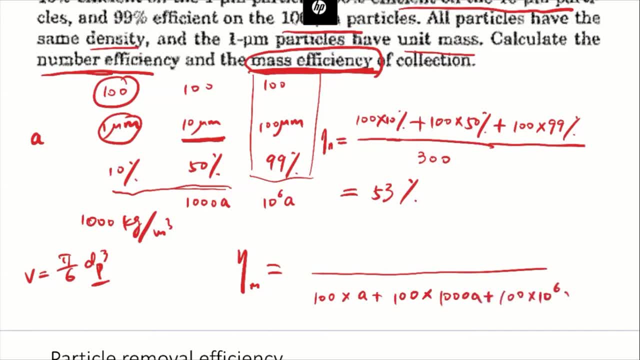 100 multiplied by 1000 a and 100 multiplied by 10 to the sixth, and 100 multiplied by 10 to the sixth and 100 multiplied by 10 to the sixth of a. so this is the total quantity of a. so this is the total quantity. 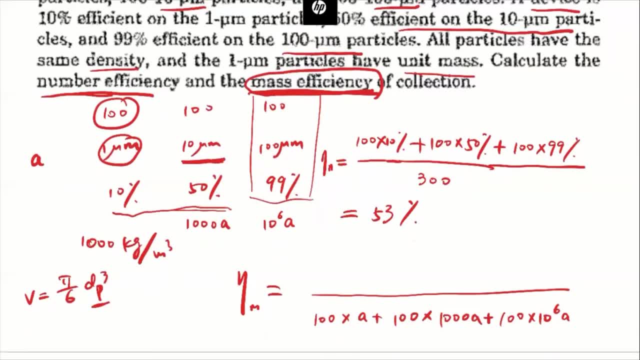 of a. so this is the total quantity and the quantity removed, and the quantity removed and the quantity removed is basically 100, is basically 100, is basically 100 multiplied by a multiplied by 10 percent, multiplied by a multiplied by 10 percent, multiplied by a multiplied by 10 percent. 100 multiplied by 1000. a. 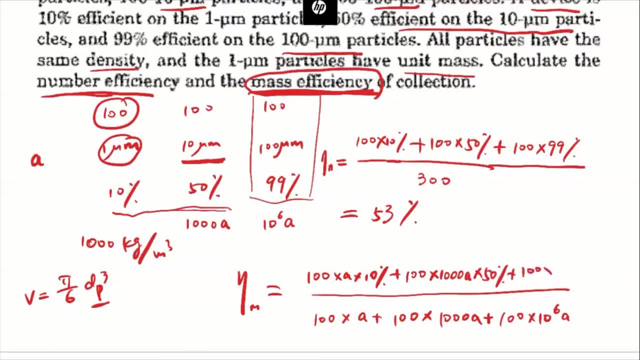 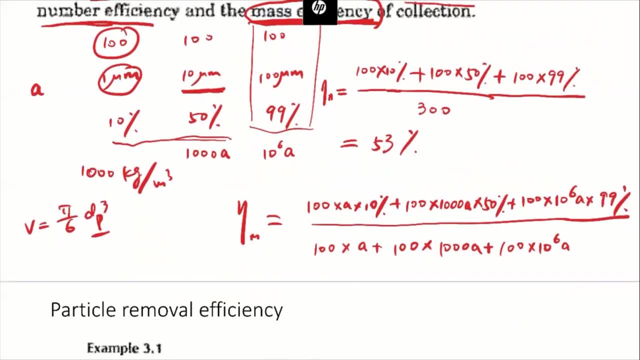 100 multiplied by 1000, a 100 multiplied by 1000 a 50 percent and 99 99, 99. so now you can see that, basically this. so now you can see that, basically this. so now you can see that, basically this number in denominator and denominator. 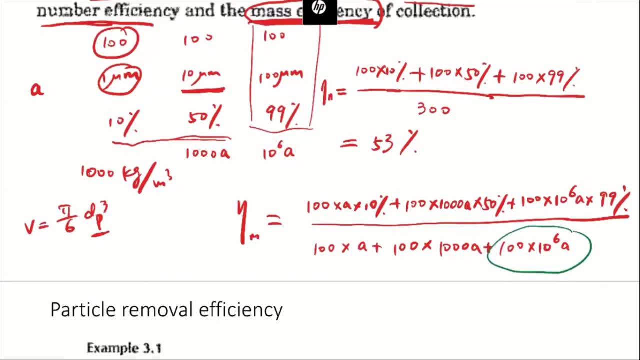 number in denominator and denominator, number in denominator and denominator, the denominator, the denominator, the denominator are just, are just, are just largely determined by this value here, largely determined by this value here, largely determined by this value here. okay, because all the a will just cancel. okay, because all the a will just cancel. 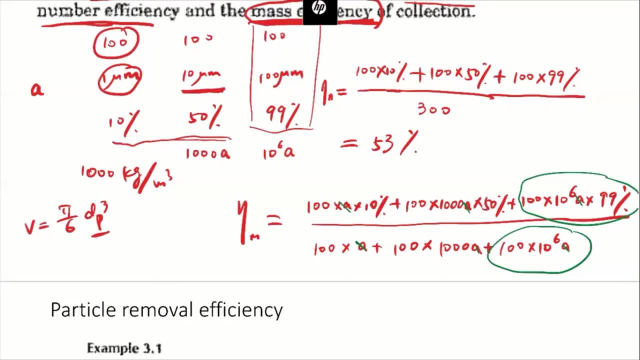 okay, because all the a will just cancel out out out. it doesn't matter what is the mass? it doesn't matter what is the mass. it doesn't matter what is the mass. for the uh, it is for the one micrometer. for the uh, it is for the one micrometer. 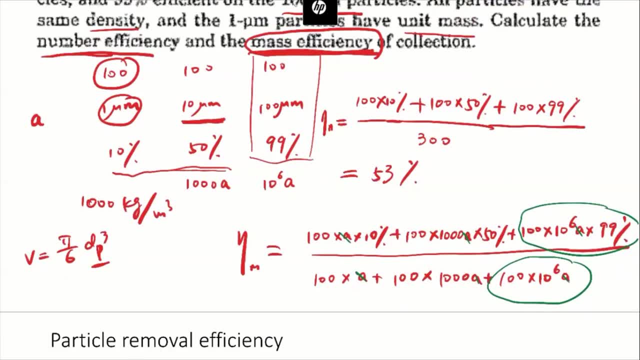 for the uh, it is for the one micrometer. particles, they're all, they're all particles, they're all, they're all particles, they're all, they're all. cancelled out, cancelled out, cancelled out. so the number here is largely determined. so the number here is largely determined. 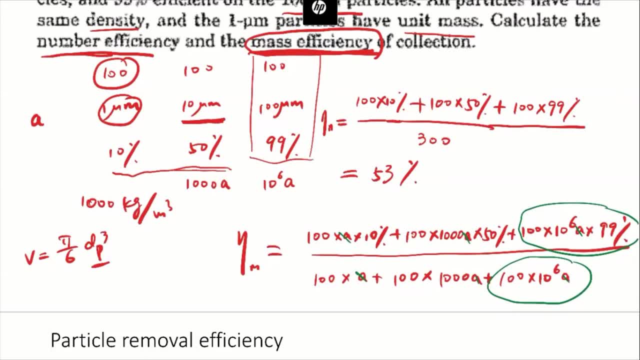 so the number here is largely determined by this, by this, by this larger sizes or the larger particles, larger sizes or the larger particles, larger sizes or the larger particles. so if you plug in all of these numbers, so if you plug in all of these numbers, so if you plug in all of these numbers, you'll find out that the removal 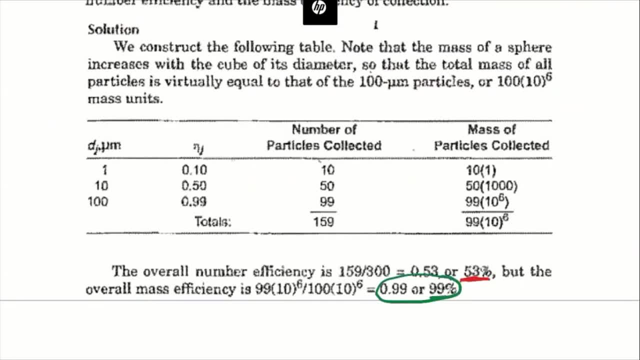 you'll find out that the removal, you'll find out that the removal, efficiency for efficiency, for efficiency, for, in terms of the mass, it's 99. in terms of the mass, it's 99. in terms of the mass, it's 99. okay mainly because. okay mainly because. 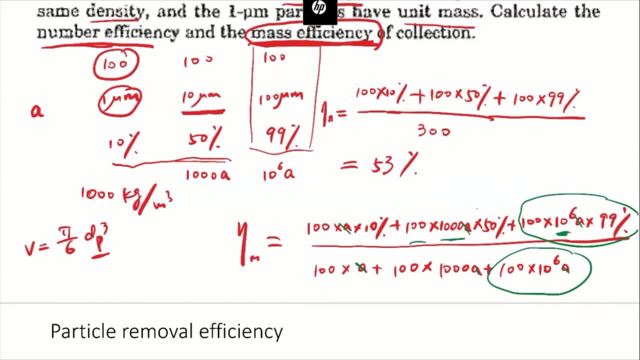 okay, mainly because these numbers are too small. this is 10 to. these numbers are too small. this is 10 to. these numbers are too small. this is 10 to the sixth. the sixth, the sixth. it's much, much larger than these numbers. it's much, much larger than these numbers. 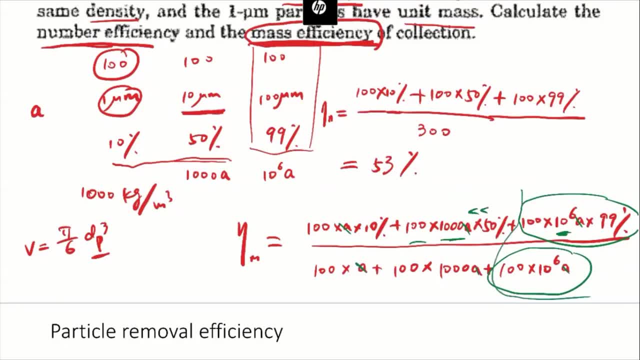 it's much, much larger than these numbers. right so, finally, right so, finally, right so, finally, if we do the approximation, it's just. if we do the approximation, it's just. if we do the approximation, it's just going to be similar to this value, going to be similar to this value. 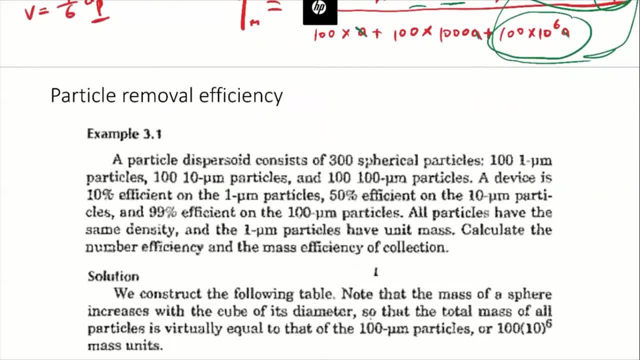 going to be similar to this value and we have 99 here, okay, and we have 99 here- okay, and we have 99 here- okay. so now you can see how different it is. so now you can see how different it is. so now you can see how different it is when we talk about the remove efficiency. 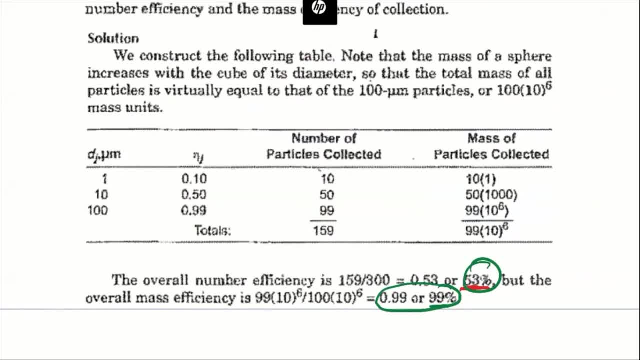 when we talk about the remove efficiency, when we talk about the remove efficiency, if it's number efficiency. if it's number efficiency. if it's number efficiency, then it's 53. if it's mass efficiency, then it's 53. if it's mass efficiency, then it's 53. if it's mass efficiency, that's 99. 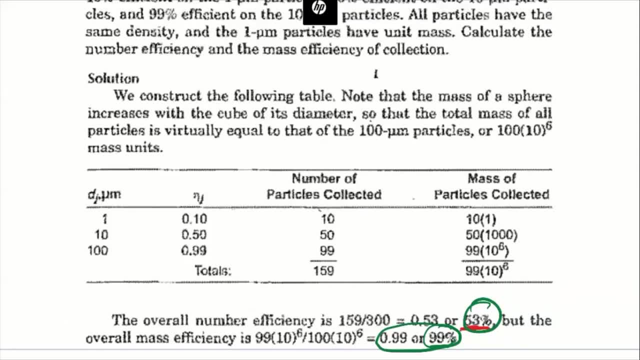 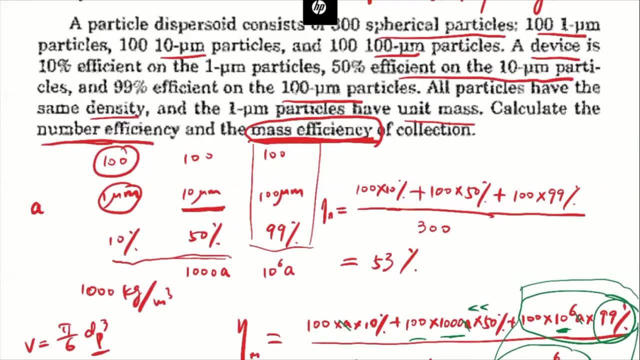 that's 99, that's 99. what happens is. what happens is. what happens is we are generating a lot of pm 2.5. we are generating a lot of pm 2.5. we are generating a lot of pm 2.5 from this process, right? so? 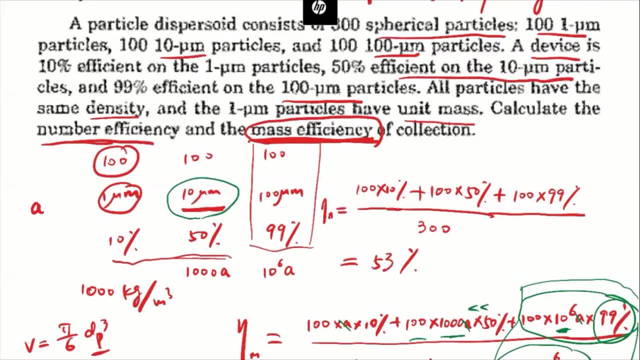 from this process, right, so from this process, right. so basically, a lot of the particles are basically a lot of the particles are basically a lot of the particles are below 10 micrometer, below 10 micrometer, below 10 micrometer or pm10. a lot of them are not even 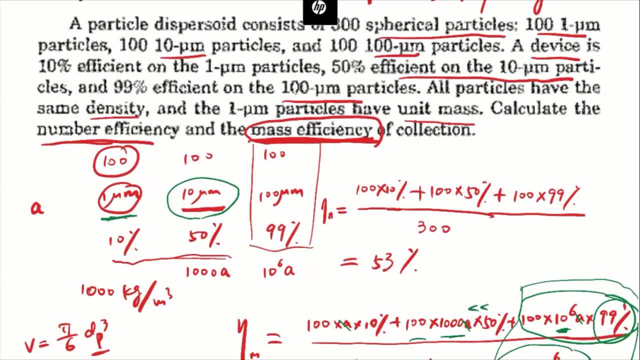 or pm10. a lot of them are not even- or pm10, a lot of them are not even removed in terms of pm1. removed in terms of pm1. removed in terms of pm1. right so, uh, that's why, although a lot, right so, uh, that's why, although a lot, 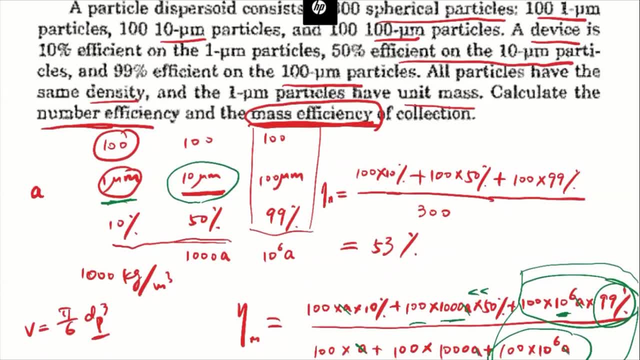 right. so, uh, that's why, although a lot of um, of um, of um, part pm control devices right now, they're part pm control devices right now. they're part pm control devices right now, they're stating that they have, stating that they have, stating that they have even have 99.9 remove efficiency. 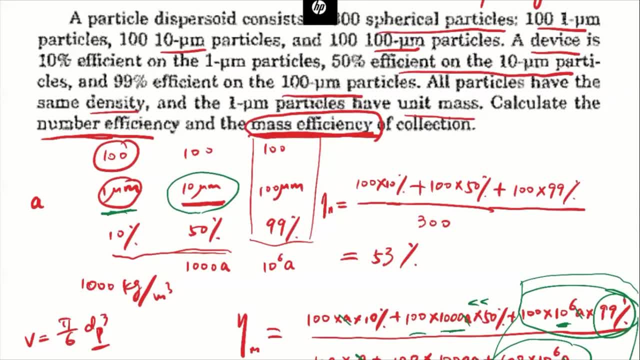 even have 99.9 remove efficiency, even have 99.9 remove efficiency. but if we talk about those particles, but if we talk about those particles, but if we talk about those particles that have the most, that have the most, that have the most, um negative, negative effects on human 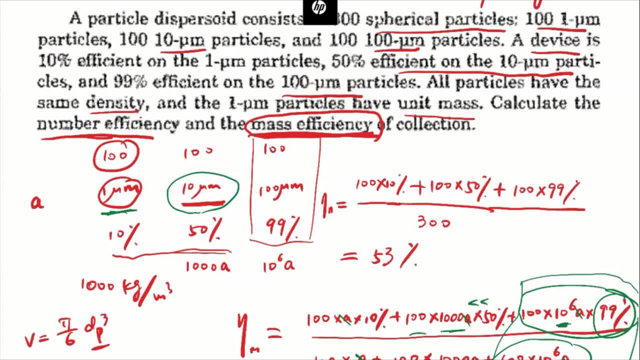 um negative, negative effects on human um negative, negative effects on human health, health, health. so those devices are still not so. those devices are still not so. those devices are still not efficient in removing them, efficient in removing them, efficient in removing them right um so just pay attention when we 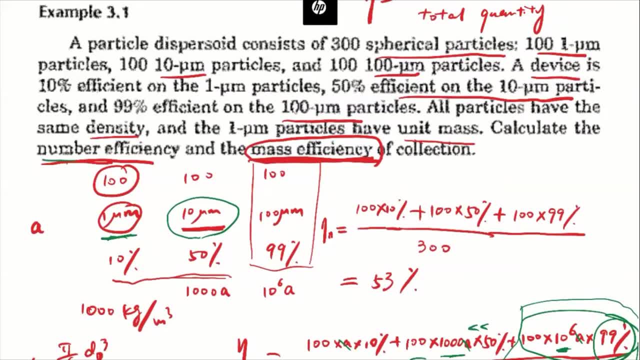 right um. so just pay attention when we right um. so just pay attention when we talk about talk about. talk about either number efficiency or mass, either number efficiency or mass, either number efficiency or mass efficiency, because they will differ by efficiency, because they will differ by efficiency, because they will differ by quite a lot if we talk about particles. 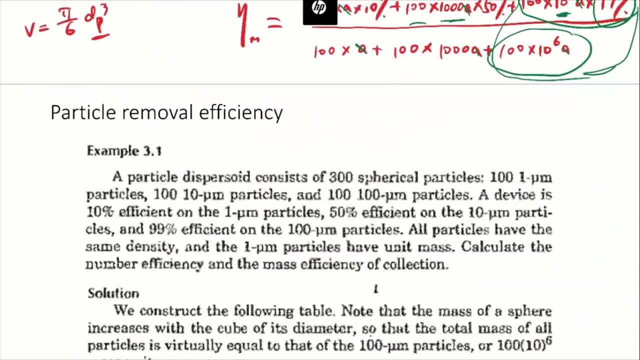 quite a lot if we talk about particles. quite a lot if we talk about particles with different sizes, with different sizes, with different sizes. all right, um. so that's all for the all right, um. so that's all for the all right, um. so that's all for the contents of this class. 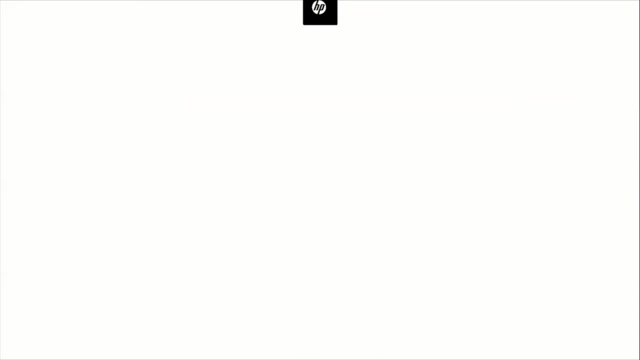 contents of this class. contents of this class: um so uh, we don't have class. um so uh, we don't have class. um so uh, we don't have class for the upcoming monday because of the for the upcoming monday because of the for the upcoming monday because of the labor day holiday. 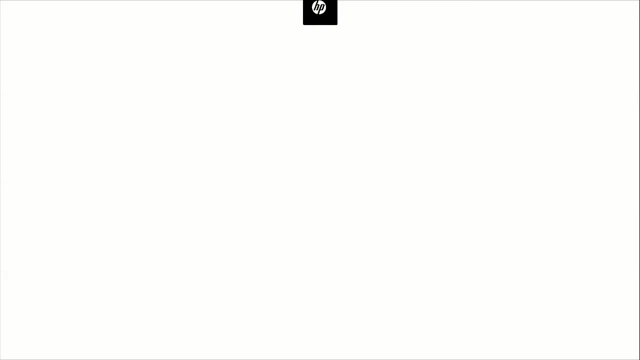 labor day holiday. labor day holiday, and um so. on wednesday i'll briefly, and um so on wednesday i'll briefly, and um so on wednesday i'll briefly introduce the, introduce the introduce the uh term projects. we're going to work. uh term projects, we're going to work. 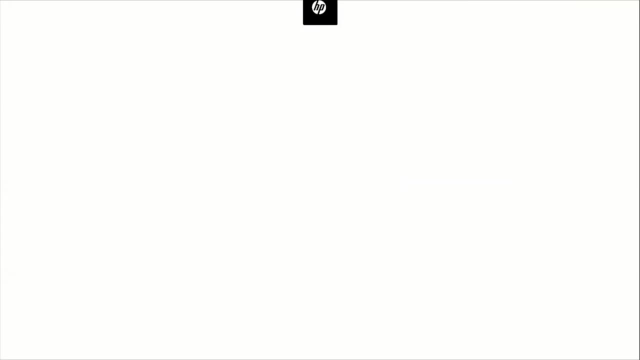 uh, term projects we're going to work on, so on, so on. so by that time, you also have your team. by that time, you also have your team. by that time you also have your team assigned. so you can assigned, so you can assigned, so you can get in contact with your teammates. and